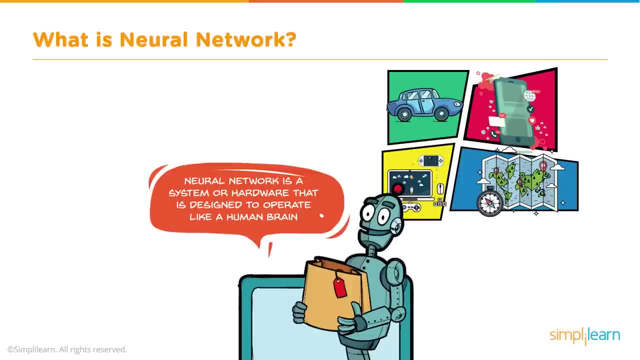 will redefine what these mean. But as far as we can in today's world, in today's commercial development, we have to compare it to what humans do. So it's we want to compare how it operates to a human brain and how it solves problems like a human does. 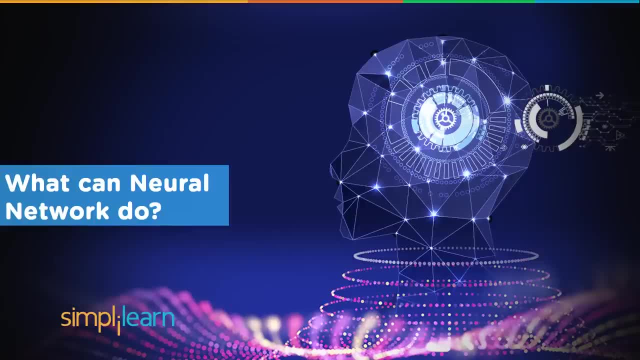 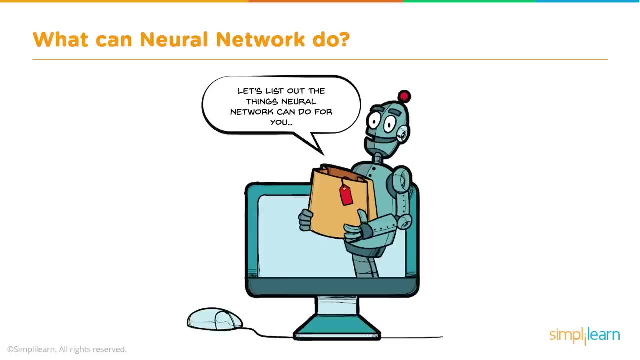 What can a neural network do? And really we're just gonna dive in deeper to what we just covered and look at other examples. So what can a neural network do? Well, let's list out the things neural networks can do for you. Translate text: 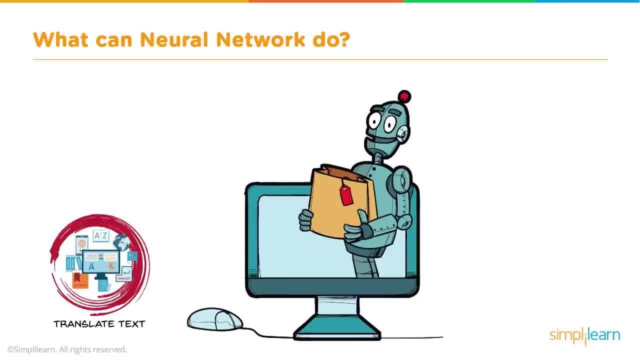 Boy. we got Google Translate and Microsoft has their own Translate. They have some really cool. They actually have an earpiece that's supposed to start translating as you talk. What a cool technology. What a cool time to live. Identify faces: Can you imagine all the uses for facial identification? 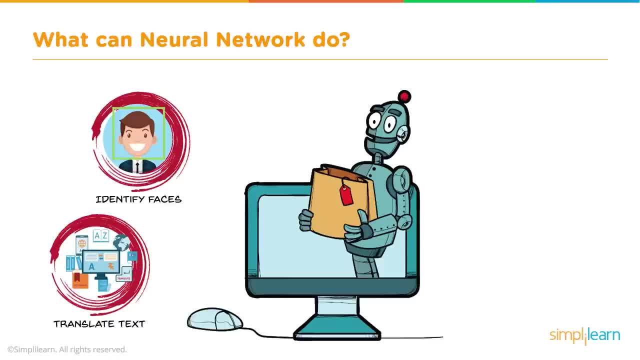 In the case of our sample or our code that we're gonna look at later, we'll be identifying dogs and cats, So not quite as detailed as understanding whose face belongs to who. I'm waiting for the Google Glasses to come out so I can see who's who and identify faces as I'm walking around. 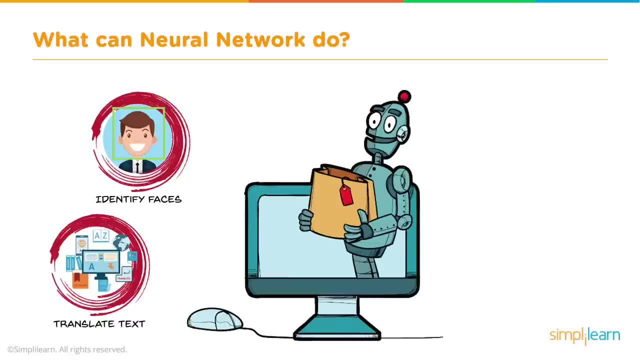 Have a little name tag over them- Not out there yet, but boy, we are close, We can identify the faces, and they have all kinds of technologies to bring that information back. Recognize speech goes along with the Translate text. So now, as you're talking into your assistant, it can use that to do commands, turn lights, on all kinds of things you can do with recognizing speech. 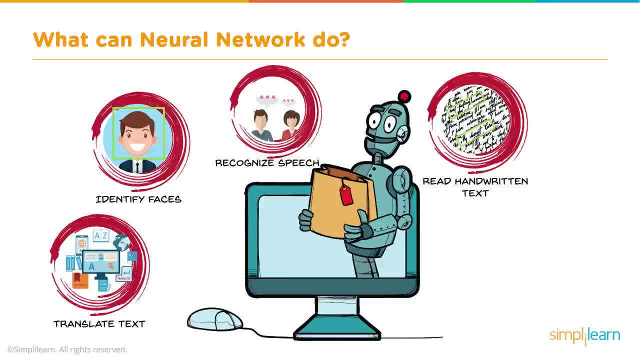 Read handwritten text. They're starting to translate all these old text documents that they've had in storage Instead of doing it individually, where somebody's going through each text by themself in a room Picture, like an old Raiders of the Lost Ark theme, where he's in the back, you know, archaeologist studying the text. 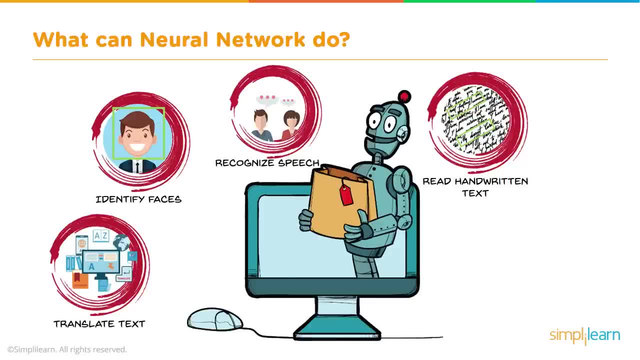 Now it's fed into a computer. They take a picture. They even use neural networks to take a scroll that is so messed up that they can't undo the scroll and they x-ray it. And then they use that x-ray to translate the text off of it without ever opening the scroll. 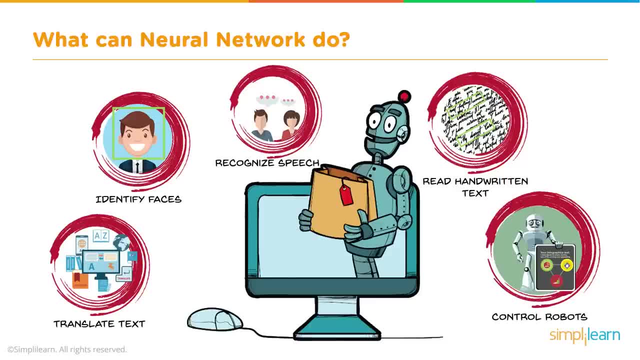 I mean, just way cool stuff they're starting to do with all this And, of course, control robots. What would be a neural network without bringing in the robots? And we have our own favorite robot in the middle who goes to our red tag cell and goes shopping for us. 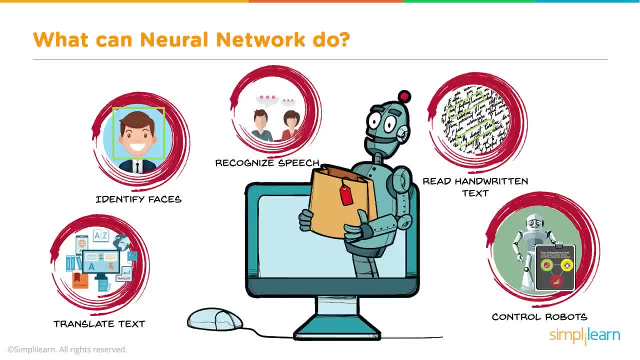 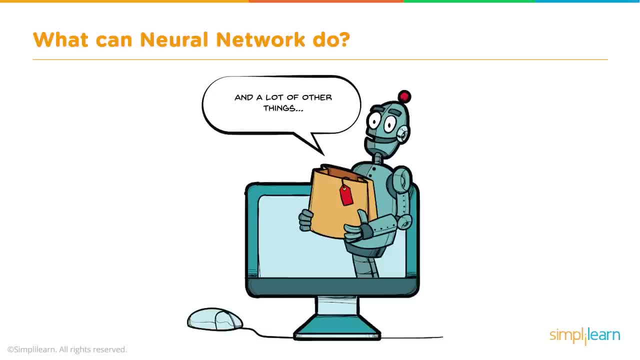 So you know, these are just a few of the wonderful things And I think that neural networks are being applied to. It's such an infant stage technology. What a wonderful time to jump in. And there are a lot of other things it goes into. 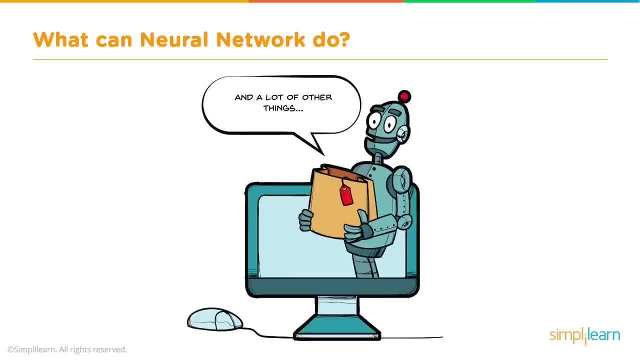 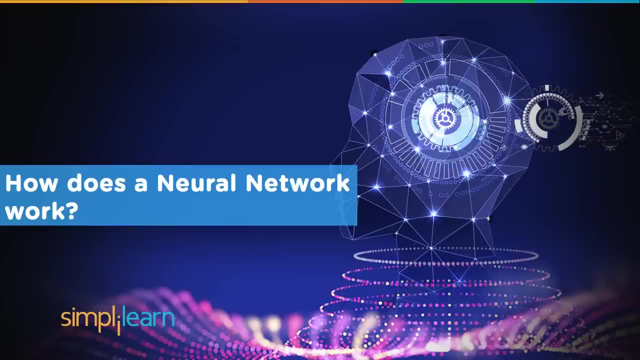 I mean, we could spend just forever talking about all the different applications, from business to whatever you can even imagine. They're now applying neural networks to help us understand. So now that we've talked a little bit about all the cool things you can do with a neural network, let's dive in and say: how does a neural network work? 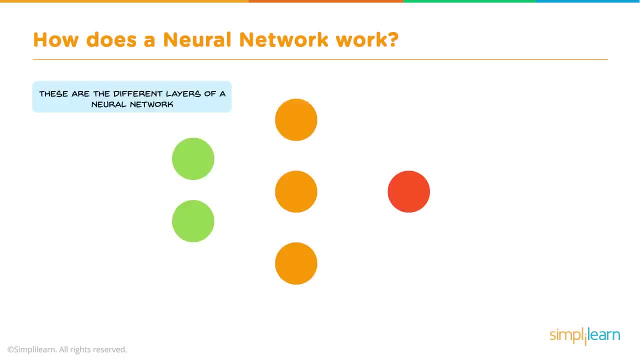 So now we've come far enough to understand how a neural network works. Let's go ahead and walk through this. So a neural network is a nice graphical representation. They usually describe a neural network as having different layers, And you'll see that we've identified a green layer, an orange layer and a red layer. 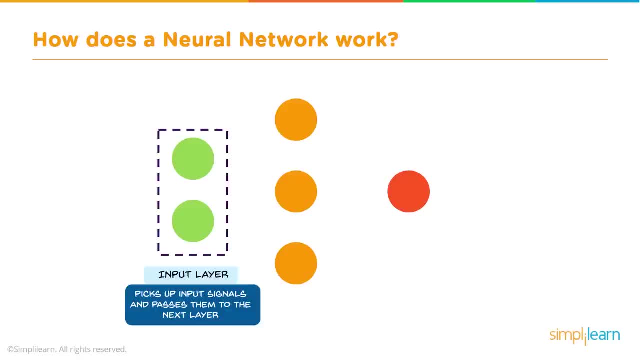 The green layer is the input, So you have your data coming in. It picks up the input signals and passes them to the next layer. The next layer does all kinds of calculations and feature extraction. It's called the hidden layer. A lot of times there's more than one hidden layer. 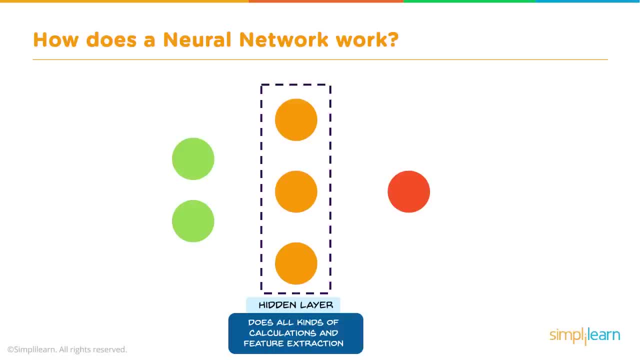 We're only showing one in this picture, but we'll show you how it looks like in more detail in a little bit. And then, finally, we have an output layer. This layer delivers the final result. So the only two things we see is the input layer and the output layer. 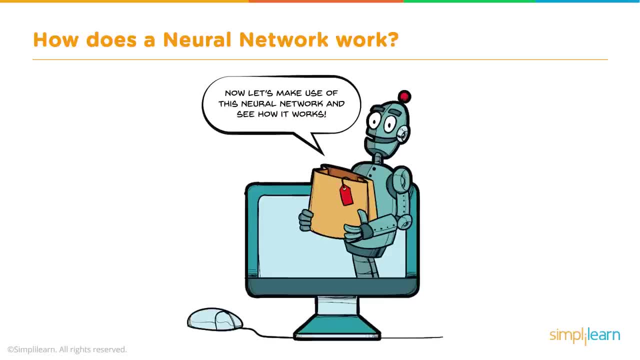 Now let's make use of this neural network and see how it works. Wonder how traffic cameras identify vehicles' registration plate on the road to detect speeding vehicles and those breaking the law. They got me going through a red light the other day. Well, last month. 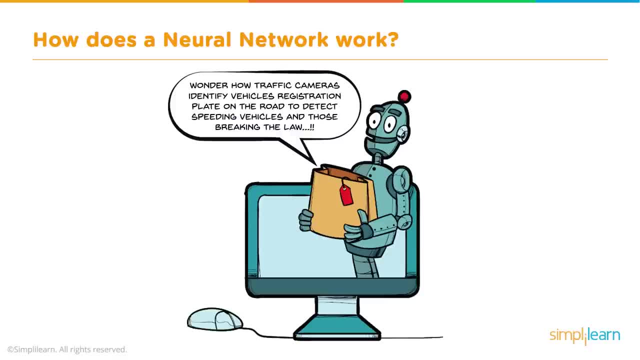 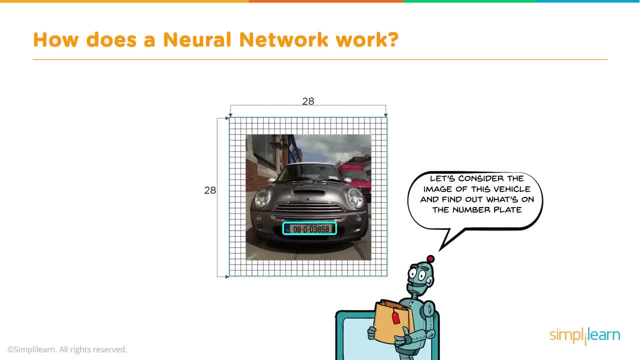 That's like the horrible thing. They send you this picture of you and all your information because they pulled it up off of your license plate and your picture. I should have gone through the red light. So here we are and we have an image of a car and you can see the license plate's on there. 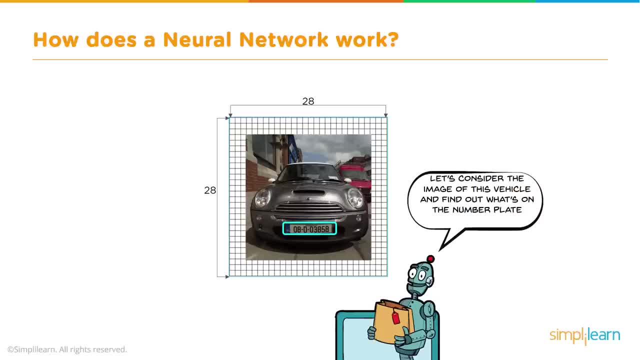 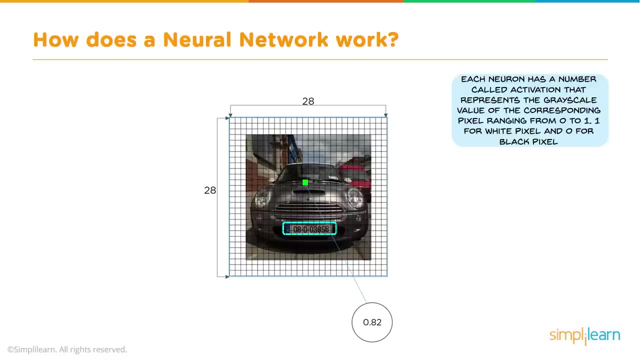 So let's consider the image of this vehicle and find out what's on the number plate. The picture itself is 28 by 28 pixels And the image is fed as an input to identify the registration plate. Each neuron has a number called activation that represents the grayscale value of the corresponding pixel range. 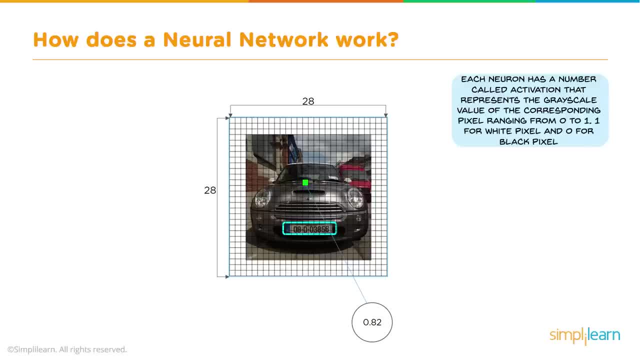 And we range it from 0 to 1.. 1 for a white pixel and 0 for a black pixel, And you can see down here we have an example where one of the pixels is registered as like 0.82, meaning it's probably pretty dark. 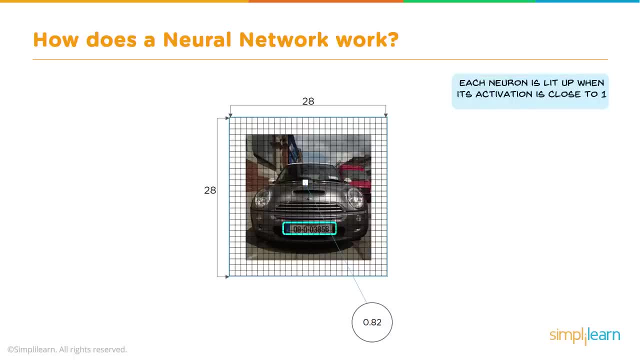 Each neuron is lit up when its activation is close to 1.. So as we get closer to black on white, we can really start seeing the details in there And you can see again. the pixel shows us one up there. It's like part of the car. 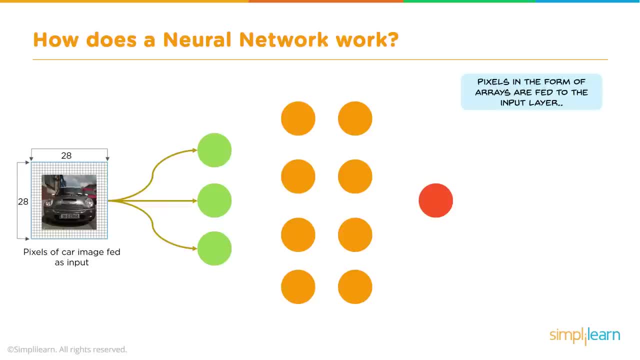 And so it lights up. So pixels in the form of arrays are fed to the input layer, And so we see here the pixel of a car image fed as an input, And you're going to see that the input layer, which is green, is one dimension. 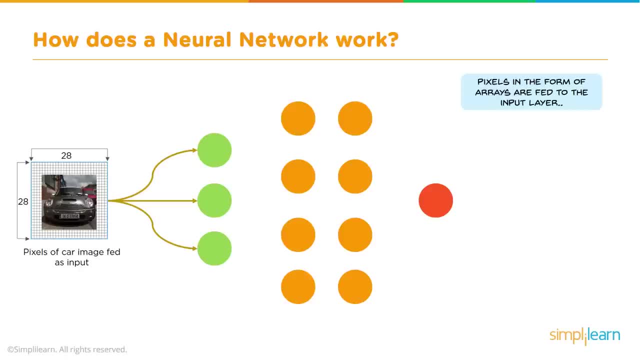 While our image is two dimension. Now, when we look at our setup that we're programming in Python, it has a cool feature that automatically does the work for us. If you're working with an older neural network pattern package, you then convert each one of those rows, so it's all one array. 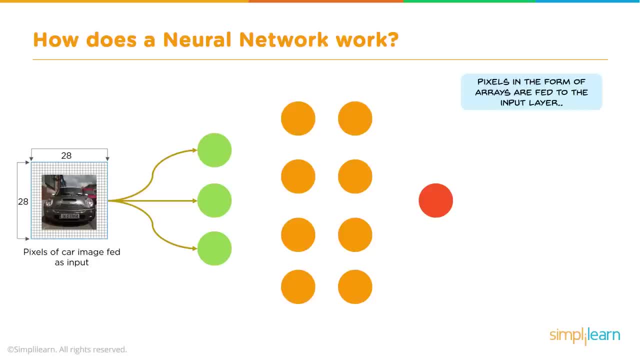 So you'd have like row 1 and then just tack row 2 onto the end. You can almost feed the image directly into some of these neural networks. The key is, though, is that if you're using a 28 by 28 and you get a picture of this 30 by 30, shrink the 30 by 30 down to fit the 28 by 28.. 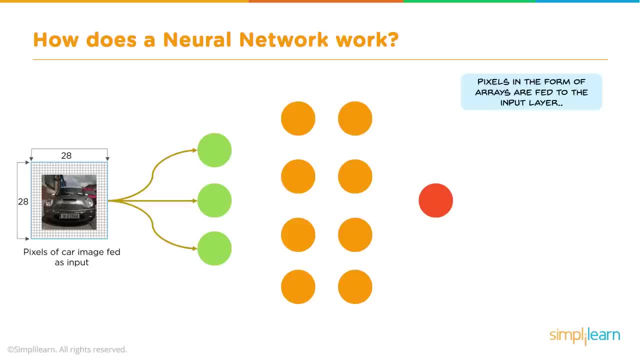 So you can't increase the number of input, in this case green dots. It's very important to remember when you're working on neural networks. And let's name the inputs x1, x2, x3 respectively, So each one of those represents one of the pixels coming in. 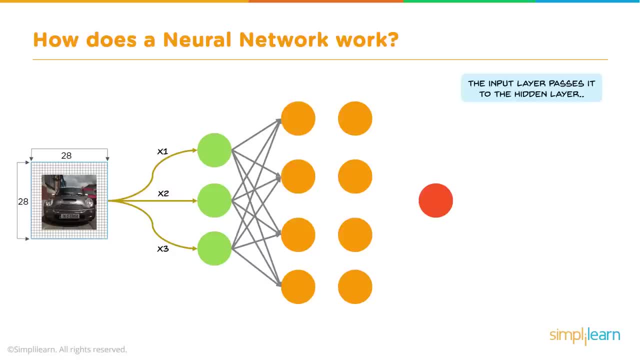 And the input layer passes it to the hidden layer. And you can see here we now have two hidden layers in this image, in the orange, And each one of those pixels connects to each one of those hidden layers And the interconnections are assigned weights at random. 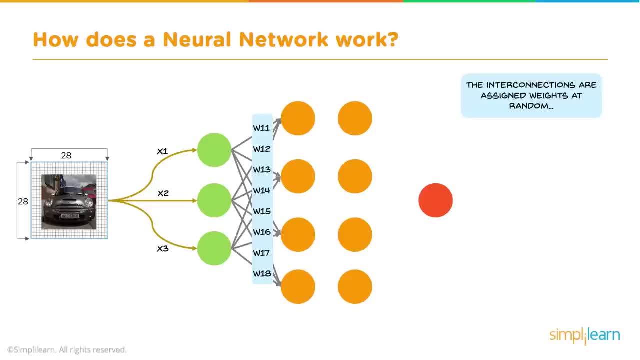 So it gets these random weights that come through. If x1 lights up, then it's going to be x1 times this weight going into the hidden layer And we sum those weights, The weights are multiplied with the input signal And a bias is added to all of them. 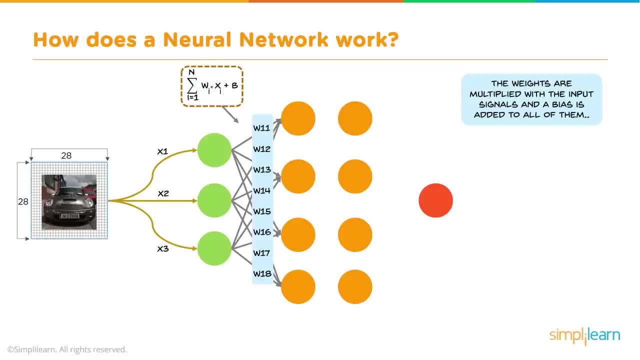 So, as you can see, here we have, x1 comes in And it actually goes to all the different hidden layer nodes, Or in this case, whatever you want to call them, Network setup, the orange dots. And so you take the value of x1, you multiply it by the weight for the next hidden layer. 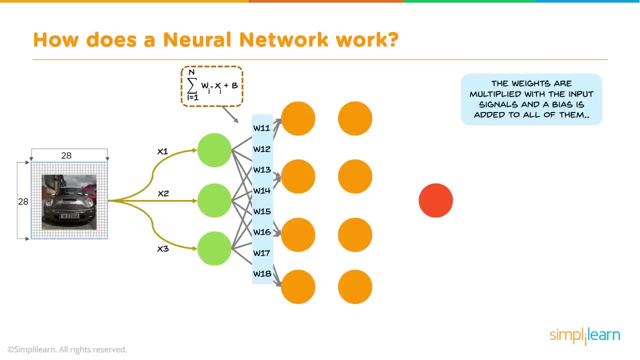 So x1 goes to hidden layer 1.. x1 goes to hidden layer 2.. x1 goes to hidden layer 1,, node 2.. Hidden layer 1,, node 3, and so on. And the bias: a lot of times they just put the bias in as like another green dot. 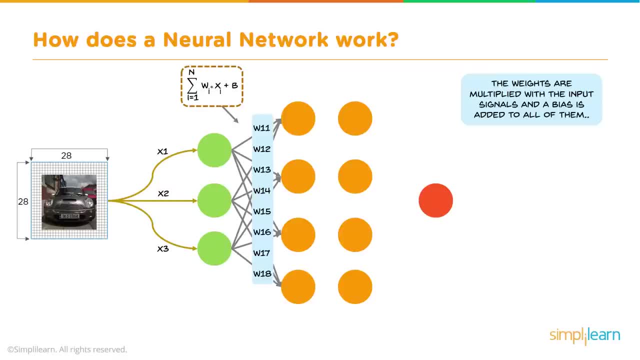 Or another orange dot, And they give the bias a value 1.. And then all the weights go in from the bias into the next node, So the bias can change. We always just remember that you need to have that bias in there. There's things that can be done with it. 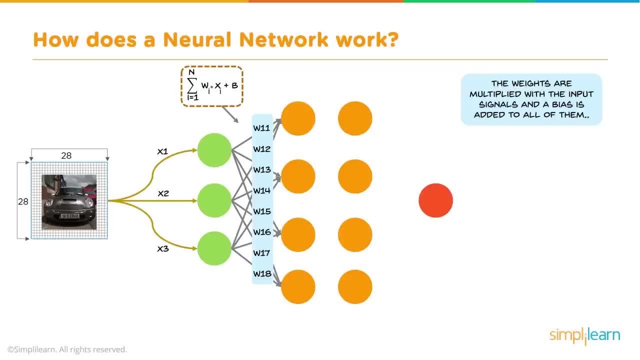 Generally, most of the packages out there control that for you, So you don't have to worry about figuring out what the bias is. But if you ever dive deep into neural networks, you've got to remember there's a bias Or the answer won't come out correctly. 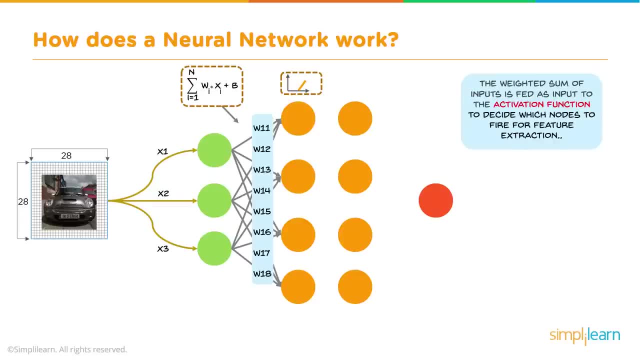 The weighted sum of the input is fed as an input to the activation function To decide which nodes to fire and for feature extraction. As the signal flows within the hidden layers, the weighted sum of inputs is calculated And is fed to the activation function in each layer to decide which nodes to fire. 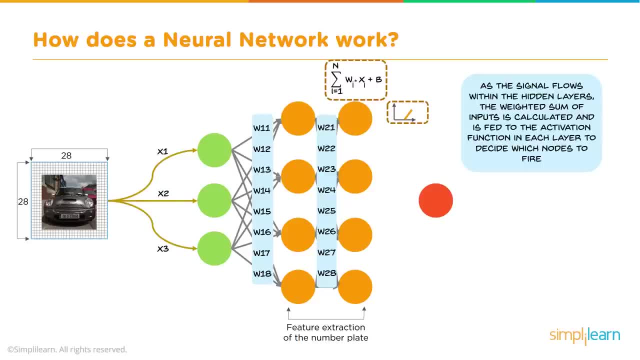 So here's our feature: extraction of the number plate. And you can see these are still hidden nodes in the middle And this becomes important. We're going to take a little detour here and look at the activation function. So we're going to dive just a little bit into the math. 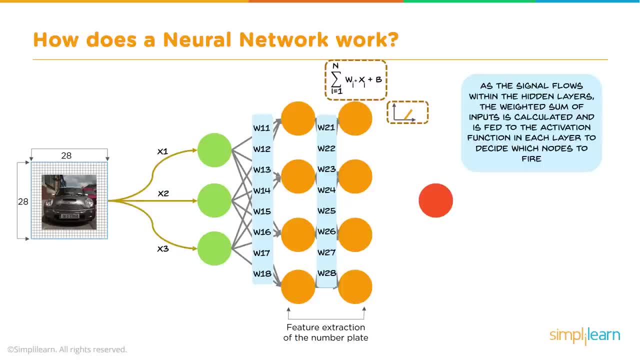 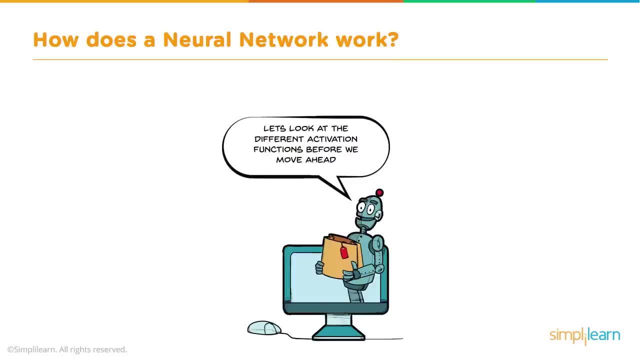 So you can start to understand where some of the games go on when you're playing with neural networks in your programming. So let's look at the different activation functions Before we move ahead. here's our friendly red tag shopping robot, And so one is the sigmoid function. 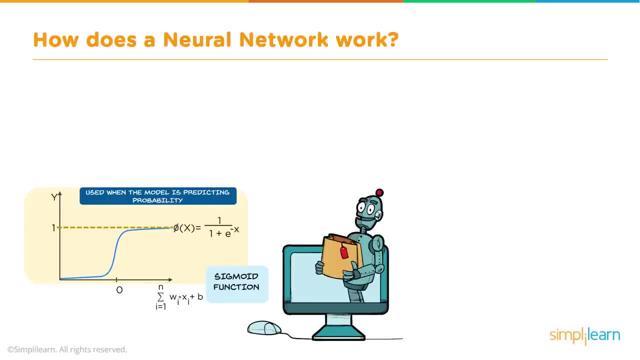 And the sigmoid function, which is 1 over 1 plus e to the minus x. takes the x value And you can see where it generates almost a 0 and almost a 1.. With a very small area in the middle where it crosses over. 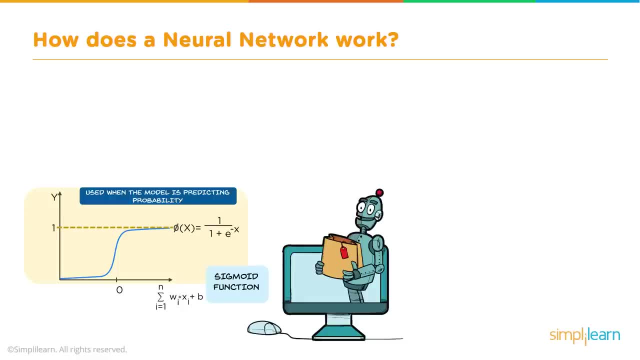 And we can use that value to feed into another function. So if it's really uncertain, it might have a 0.1 or 0.2 or 0.3.. But for the most part it's going to be really close to 1 and really close to, in this case, 0.. 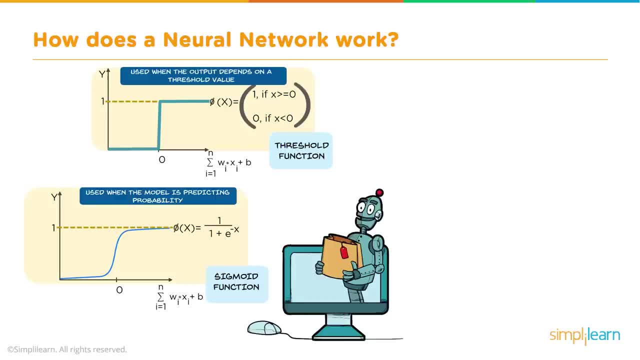 0 to 1.. The threshold function. So if you don't want to worry about the uncertainty in the middle, you just say: oh, if x is greater than or equal to 0. If not, then x is 0.. 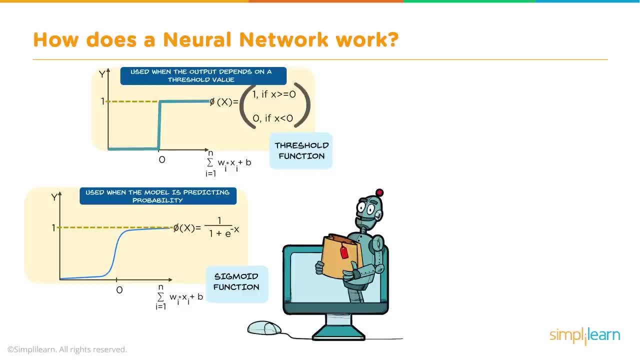 So it's either 0 or 1.. Really straightforward. There's no in between, in the middle, And then there's the threshold function. Then you have what they call the relu function, And you can see here where it puts out the value. 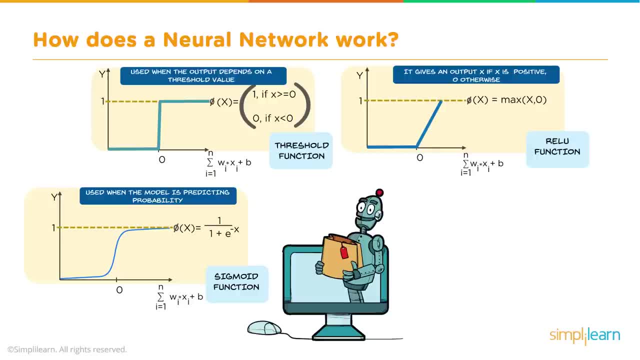 But then it says, well, if it's over 1, it's going to be 1., And if it's less than 0, it's 0. So it kind of just dead ends it on those two ends, But it allows all the values in the middle. 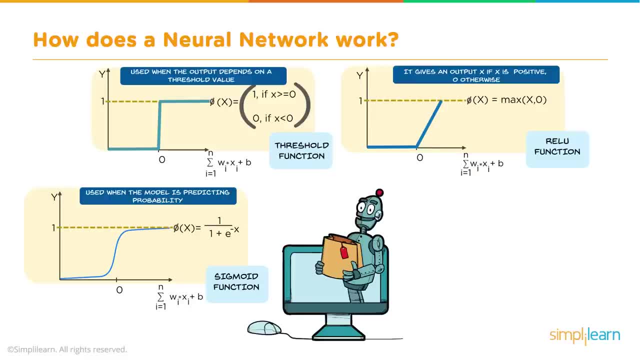 And again, this, like the sigmoid function, allows that information to go to the next level. So it might be important to know if it's a 0.1 or a minus 0.1.. The next hidden layer might pick that up and say, oh, this piece of information is uncertain. 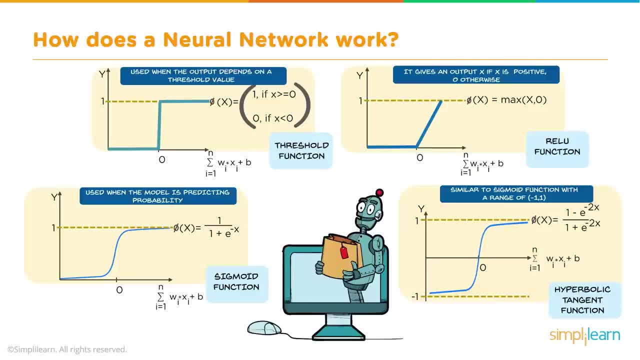 Or this value has a very low certainty to it. And then the hyperbolic tangent function, And you can see here it's 1 minus e to the minus 2x over 1 plus e to the minus 2x And it's very much along the same theme. 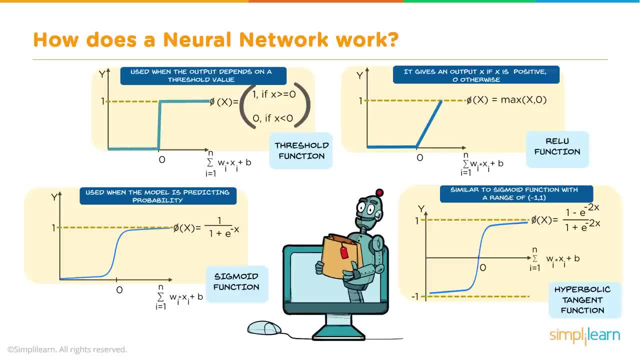 A little bit different in here, in that it goes between minus 1 and 1.. So you'll see some of these. they go 0 to 1. But this one goes minus 1 to 1. And if it's less than 0, it doesn't fire. 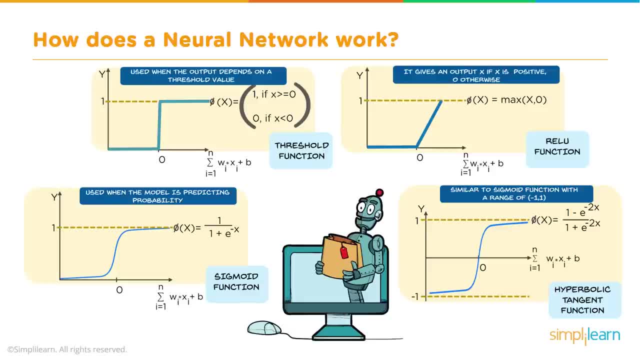 And if it's over 0, it fires And it also still puts out a value. So you still have a value. you can get off of that Just like you can with the sigmoid function and the ReLU function- Very similar in use. 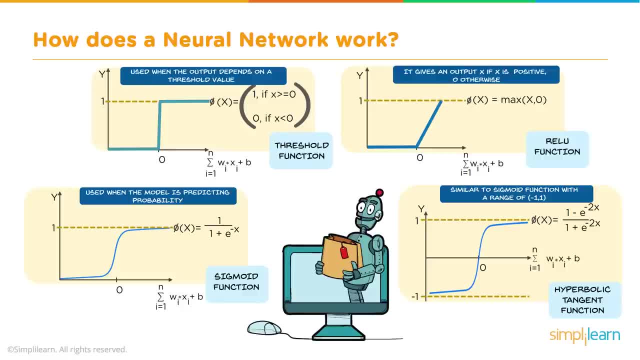 And I believe they originally used to be. everything was done in the sigmoid function That was the most commonly used, And now they just kind of use more the ReLU function. The reason is one: it processes faster Because you already have the value. 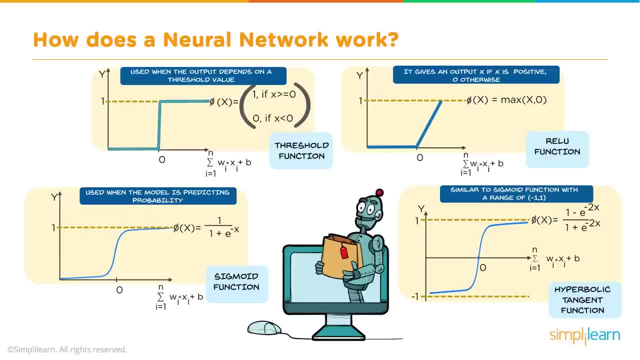 And you don't have to add another compute the 1 over 1 plus e to the minus x for each hidden node And the data coming off works pretty good. as far as putting it into the next level, If you want to know just how close it is to 0.. 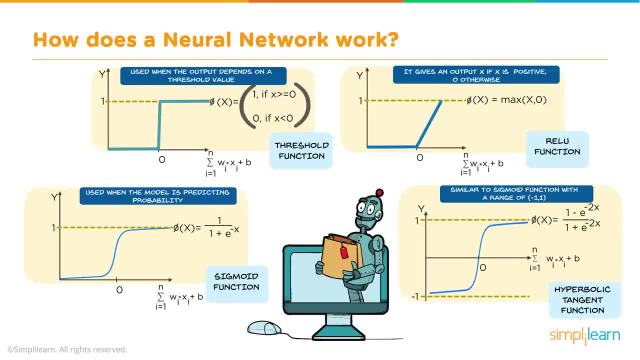 How close is it not to functioning? Is it minus 0.1? Minus 0.2?? Usually they're float values. You get like minus 0.00138 or something. So you know important information. But the ReLU is most commonly used these days. as far as the setup we're using, 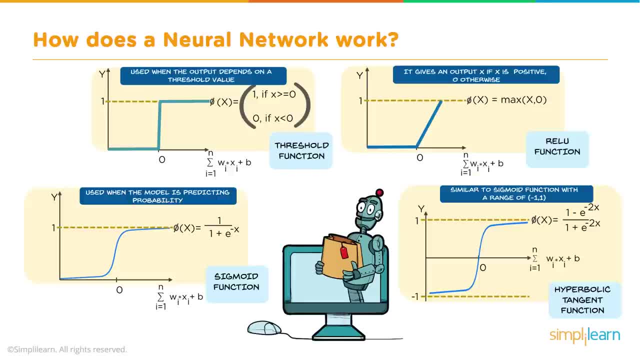 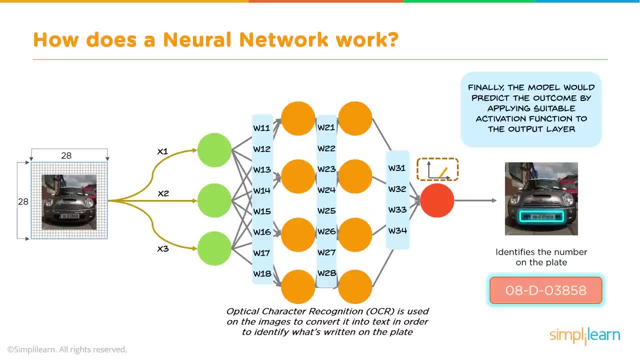 But you'll also see the sigmoid function, very commonly used also. Now that you know what an activation function is, let's get back to the neural network. So finally, the model would predict the outcome of applying a suitable activation function to the output layer. 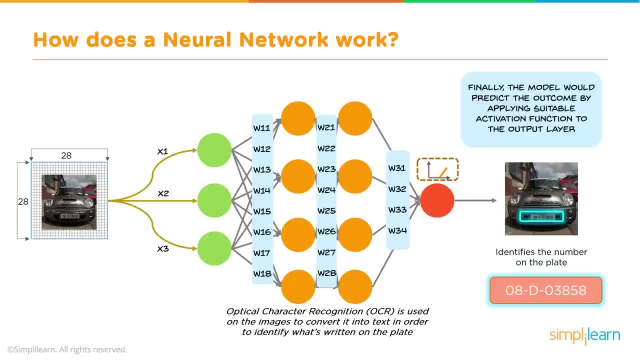 So we go in here, We look at this. The optical character recognition, OCR, is used on the images to convert it into a text in order to identify what's written on the plate, And as it comes out, you'll see the red node. 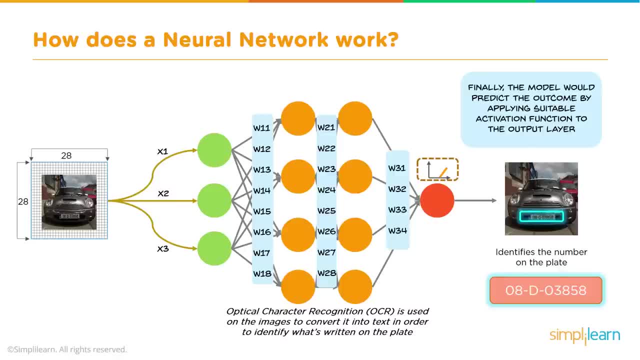 And the red node might actually represent just the letter A, So there's usually a lot of outputs when you're doing text identification. We're not going to show that on here, But you might have it even in the order. It might be what order the license plate's in. 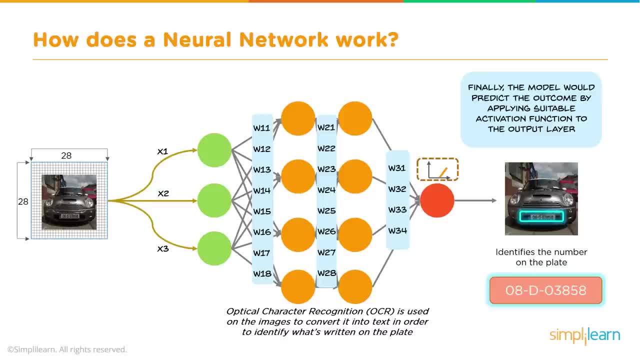 So you might have A, B, C, D, E, F, G- you know the alphabet plus the numbers- And you might have the 1,, 2,, 3,, 4,, 5,, 6,, 7, 8.. 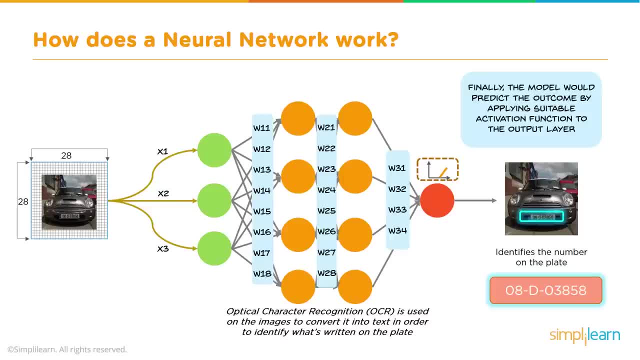 Ten places, So it's a very large array that comes out. It's not a small amount of. you know we show three dots coming in, eight hidden layer nodes. you know two sets of four. We just show one red coming out. 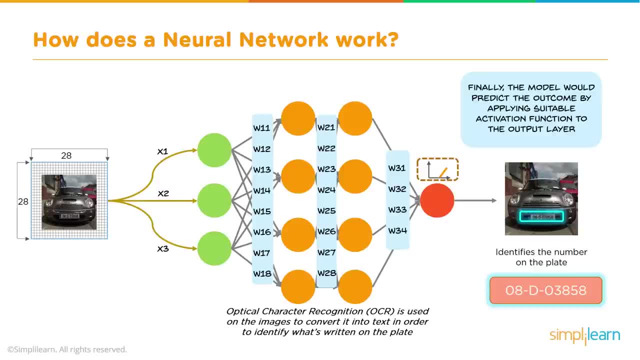 A lot of times this is you know 28 times 28.. If you did 30 times 30, that's you know 900 nodes. So 28 is a little bit less than that, Just on the input. 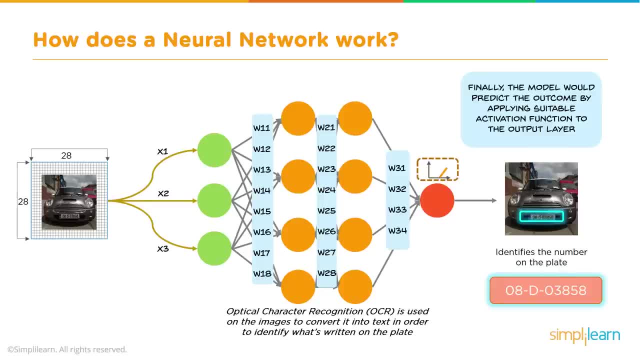 And so you can imagine, the hidden layer is just as big. Each hidden layer is just as big, if not bigger, And the output is going to be. There's so many digits. You know it's a lot, It's a huge amount of input and output. 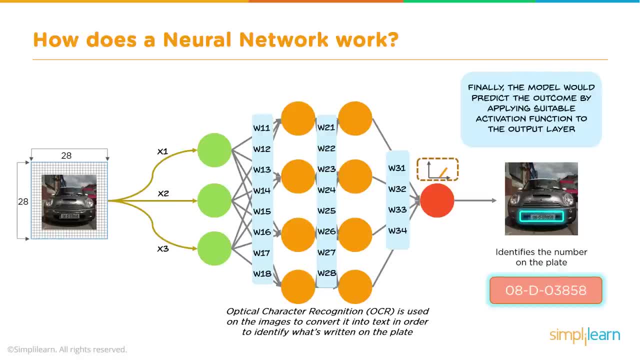 But we're only showing you just. you know it would be hard to show in one picture. And so it comes up and this is what it finally gets out on. the output is: it identifies a number on the plate, And in this case we have 08-D-03858.. 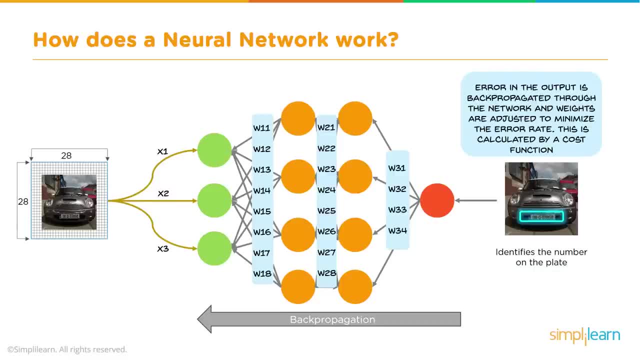 Error in the output is back propagated through the network And weights are adjusted to minimize the error rate. This is calculated by a cost function. When we're training our data, this is what's used And we'll look at that in the code. 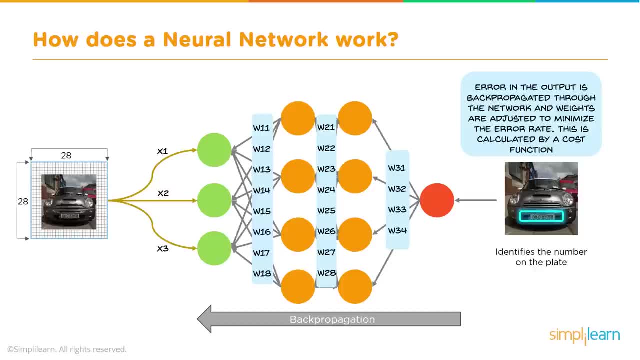 And we do the data training. So we have stuff we know the answer to And then we put the information through And it says, yes, that was correct or no, Because, remember, we randomly set all the weights to begin with And if it's wrong we take that error. 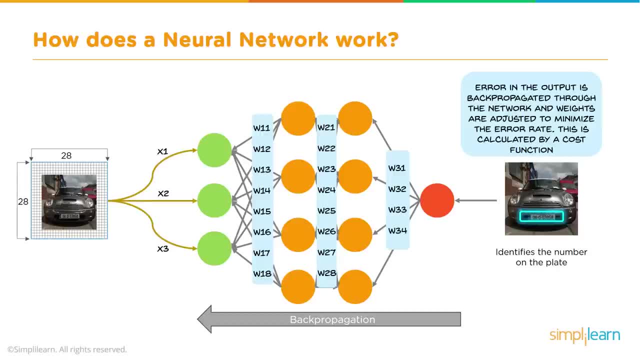 How far off are you? You know, are you off by? if it was like minus 1, you're just a little bit off. If it's like minus 300 was your output. Remember when we're looking at those different options. 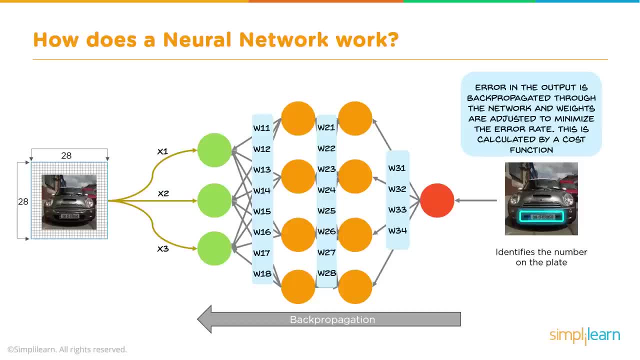 You know, hyperbolic or whatever, And we're looking at the REL. The REL doesn't have a limit on time. It's either top or bottom. It actually just generates a number. So if it's way off you have to adjust those weights a lot. 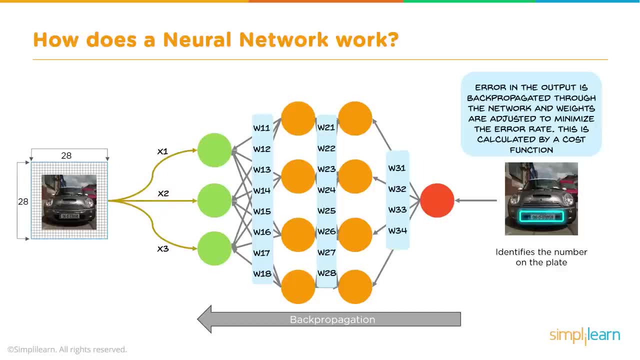 But if it's pretty close you might adjust the weights just a little bit And you keep adjusting the weights until they fit all the different training models you put in. So you might have 500 training models And those weights will adjust using the back propagation. 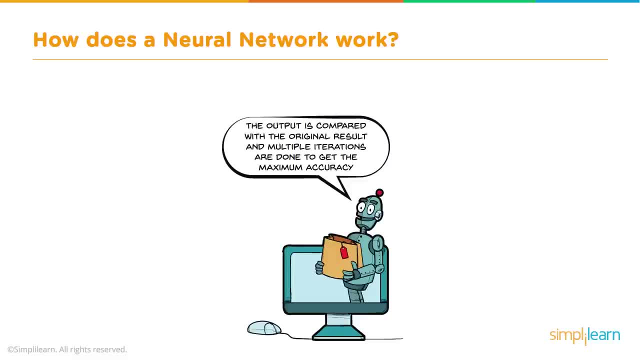 It sends the error backward, The output is compared with the original result, And multiple iterations are done to get the maximum accuracy. So not only does it look at each one, But it goes through it And it just keeps cycling through the data. 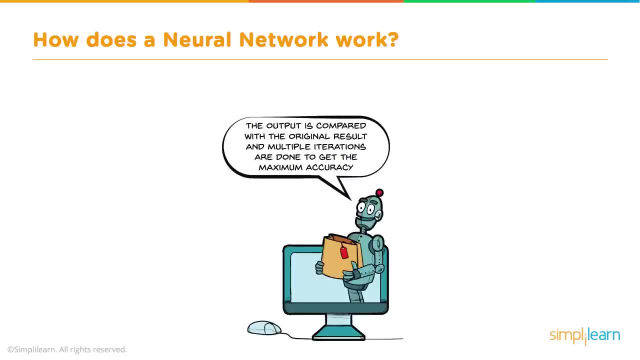 Making small changes in the network until it gets the right answers. With every iteration, the weights at every interconnection are adjusted based on the error. We're not going to dive into that math Because it is a differential equation And it gets a little complicated. 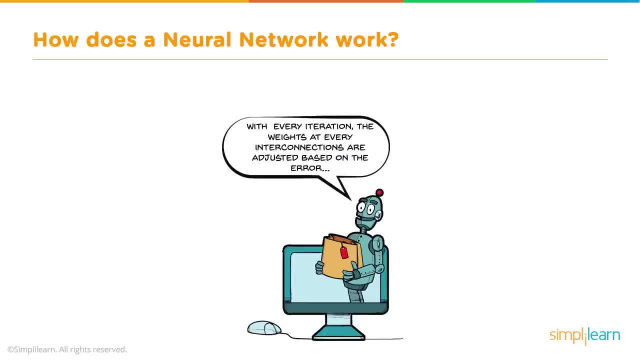 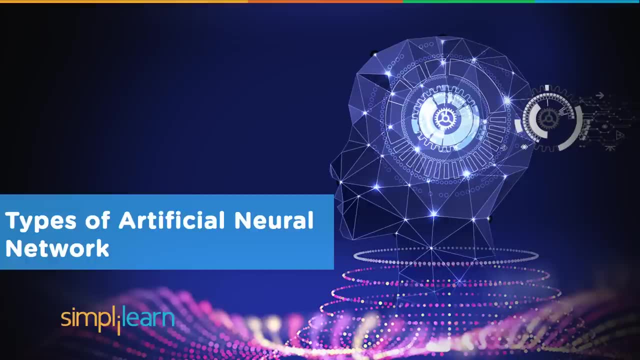 But I will talk a little bit about some of the different options they have when we look at the code. So we've explored a neural network. Let's look at the different types of artificial neural networks, And this is like the biggest area growing. 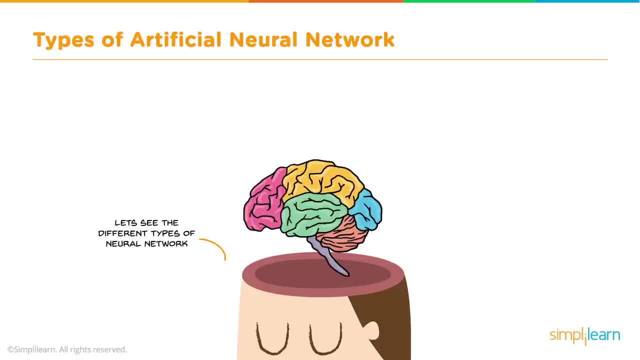 Is how these all come together. Let's see the different types of neural network. And again, we're comparing this to human learning. So here's a human brain. I feel sorry for that poor guy. So we have a feed forward: neural network. 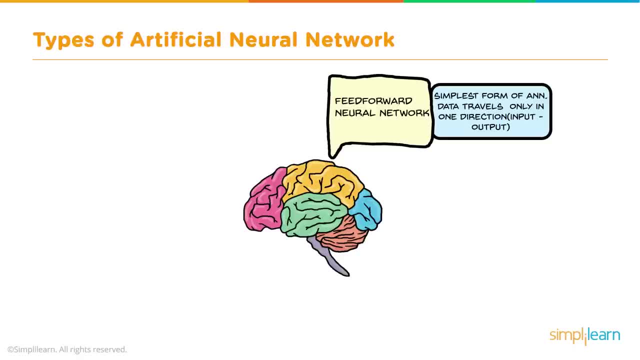 Simplest form of a. they call it an ANN, A neural network. Data travels only in one direction: Input to output. This is what we just looked at. So as the data comes in, All the weights are added, It goes to the hidden layer. 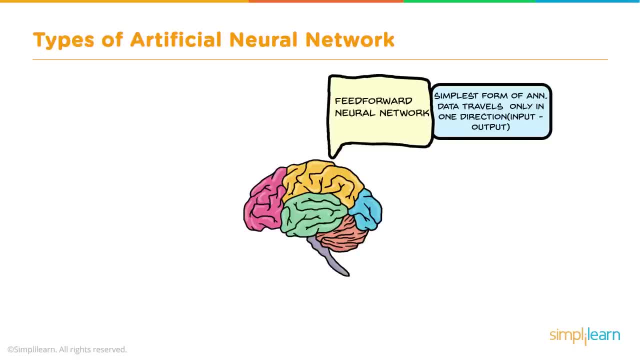 All the weights are added, It goes to the next hidden layer. All the weights are added And it goes to the output. The only time you use the reverse propagation is to train it, So when you actually use it, it's very fast. 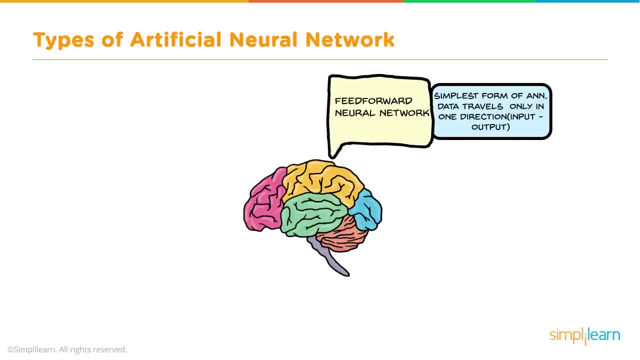 When you're training it. it takes a while Because it has to iterate through all your training data And you start getting into big data, Because you can train these with a huge amount of data. The more data you put in, the better train they get. 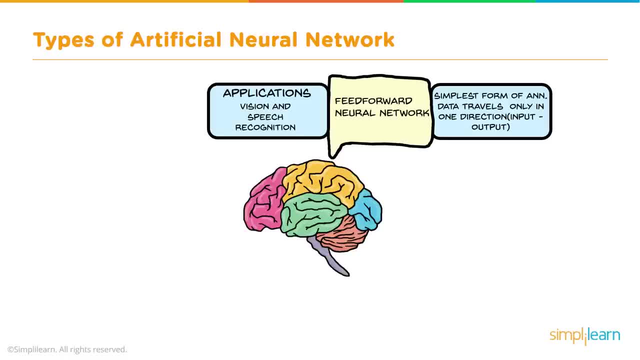 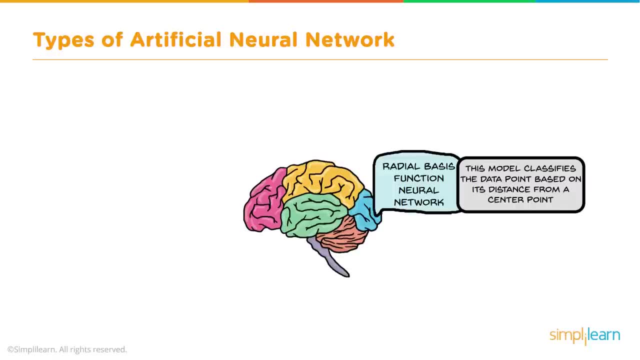 The applications: Vision and speech recognition. Actually, they're pretty much everything we talked about. A lot of almost all of them use this form of neural network at some level. Radial basis function Neural network. This model classifies the data point based on its distance from a center point. 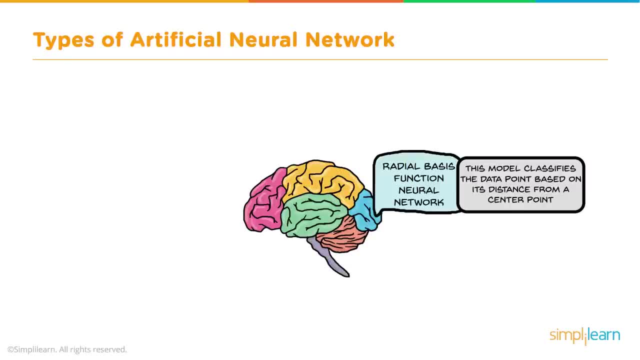 What that means is that you might not have training data, So you want to group things together And you create central points And it looks for all the things You know. some of these things are just like the other. If you've ever watched the Sesame Street as a kid, that dates me. 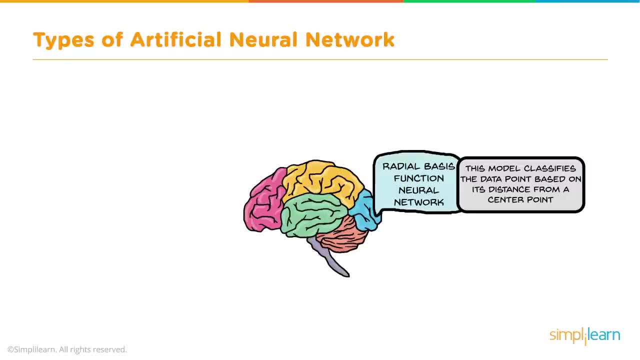 So it brings things together And this is a great way. if you don't have the right training model, You can start finding things that are connected. you might not have noticed before: Applications, Power restoration systems- They try to figure out what's connected. 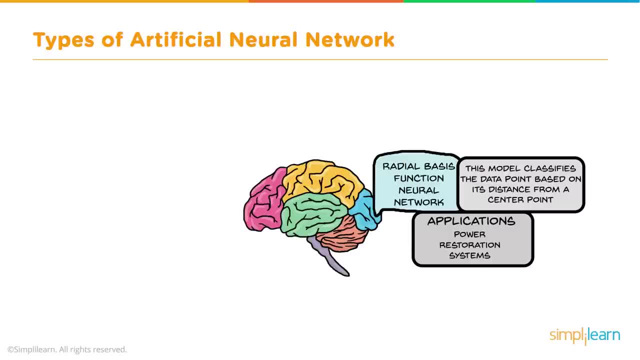 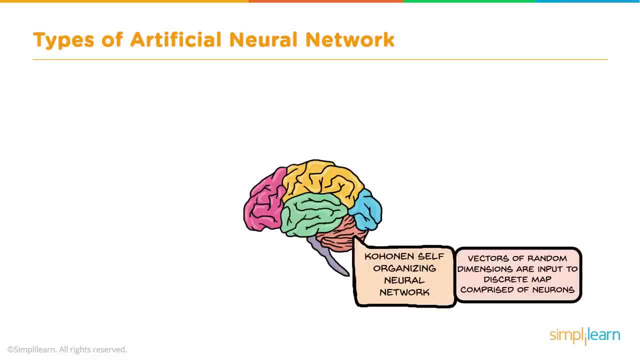 And then, based on that, they can fix the problem if you have a huge power system, Cajon and self-organizing neural network. Vectors of random dimensions are input to discrete map comprised of neurons, So they basically find a way to draw. 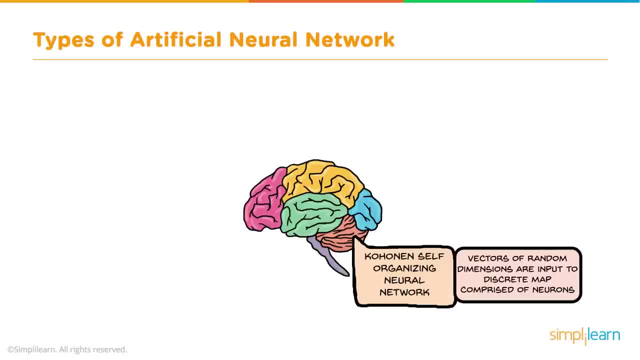 And they call them. they say dimensions Or vectors Or planes, Because they actually chop the data in one dimension, two, dimension, three, dimension four, five, Six. They keep adding dimensions and finding ways to separate the data And connect different data pieces together. 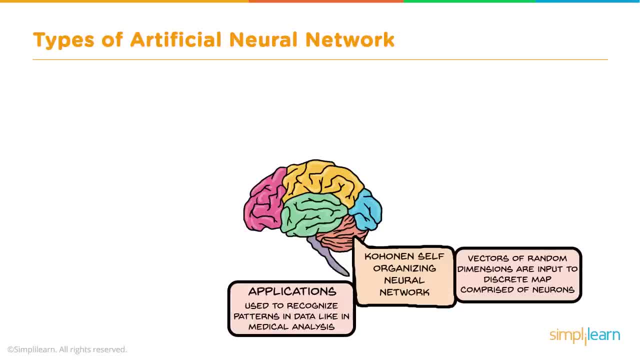 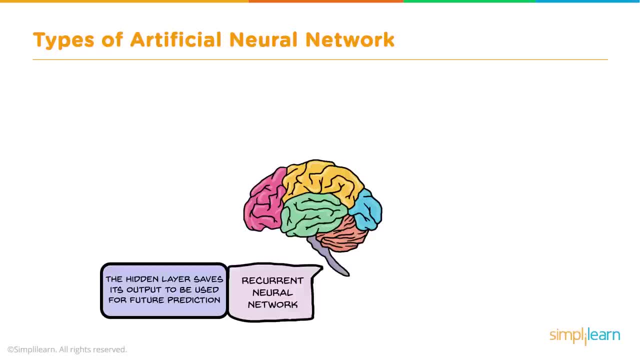 Applications Used to recognize patterns in data, Like in medical analysis. The hidden layer saves its output to be used for future prediction, Recurrent neural networks. So the hidden layers remember its output from last time And that becomes part of its new input. 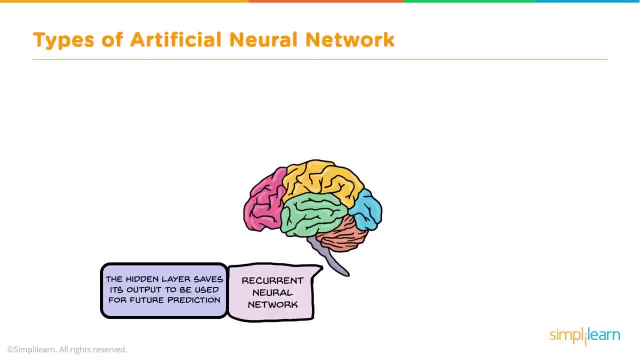 You might use that, especially in robotics or flying a drone. You want to know what your last change was And how fast it was going, To help predict what's your next change You need to make is To get to where the drone wants to go. 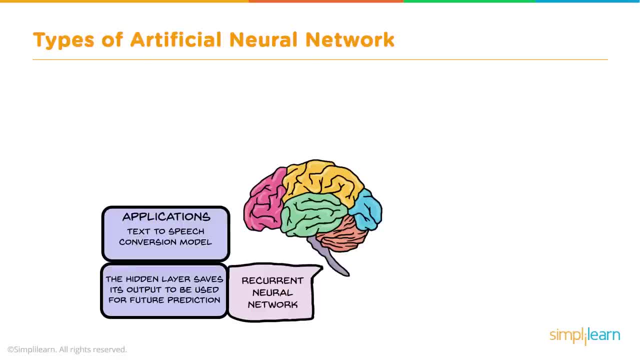 Applications: Text to speech Conversation model. So I talked about drones, But just identifying on Lexus or Google Assistant Or any of these They're starting to add in. I'd like to play a song on my Pandora And I'd like it to be at volume 90%. 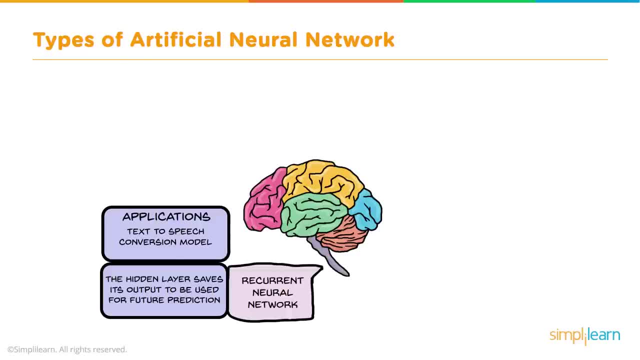 So you now can add different things in there And it connects them together. The input features are taken in batches Like a filter. This allows a network to remember an image in parts: Convolution, Neural network, Today's world in photo identification. 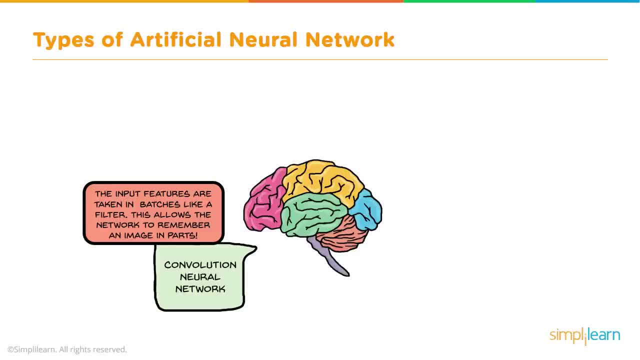 And taking apart photos And trying to Have. you ever seen that on Google, Where you have five people together? This is the kind of thing: Separates all those people, So then it can do a face recognition on each person. Applications used in signal and image processing. 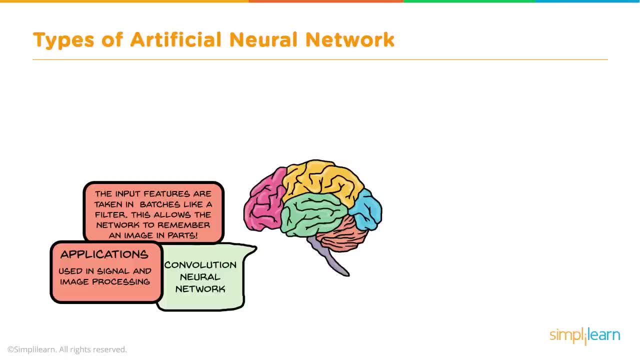 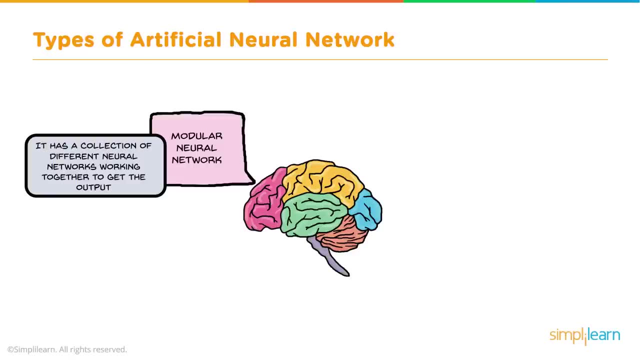 In this case, I used facial images Or Google picture images as one of the options. Modular neural network: It has a collection of different neural networks Working together to get the output. So, wow, We just went through all these different types of neural networks. 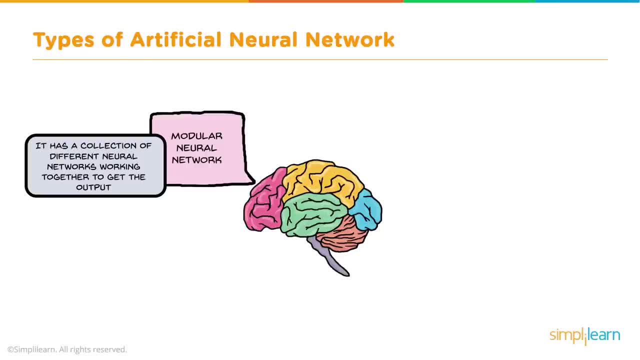 And the final one Is to put multiple neural networks together, And I mentioned that a little bit When we separated people in a larger photo And individuals in the photo And then do the facial recognition on each person. So one network is used to separate them. 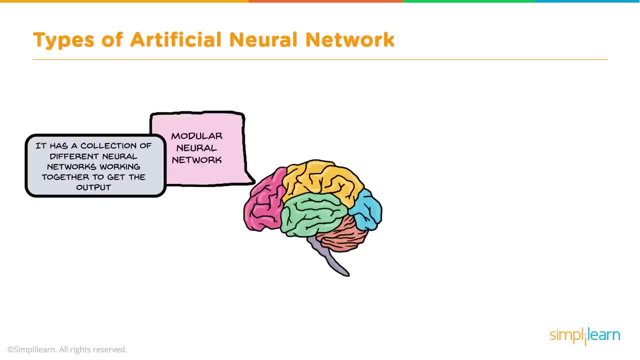 And the next network is then used to figure out who they are And do the facial recognition Applications still undergoing research. This is the cutting edge. You hear the term pipeline And there's actual In Python code And in almost all the different neural network setups out there. 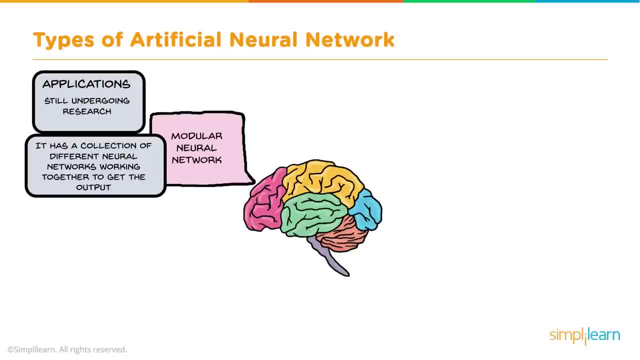 They now have a pipeline feature usually, And it just means you take the data from one neural network And maybe another neural network, Or you put it into the next neural network And then you take three or four other neural networks And feed them into another one. 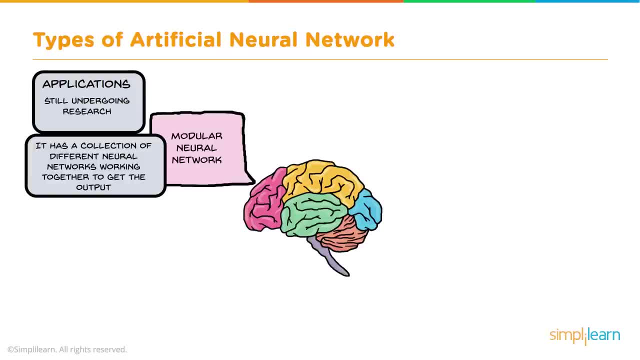 So how we connect the neural networks Is really just cutting edge, And it's so experimental- I mean it's almost creative in its nature. There's not really a science to it, Because each specific domain Has different things it's looking at. 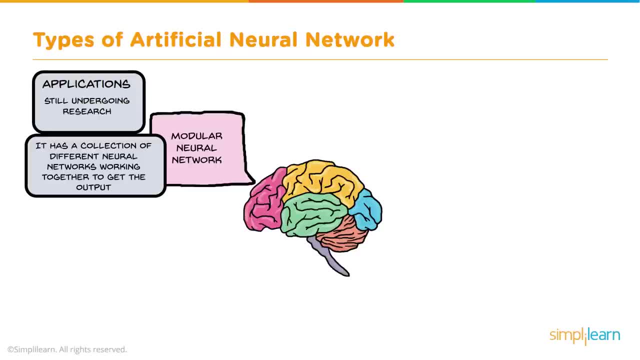 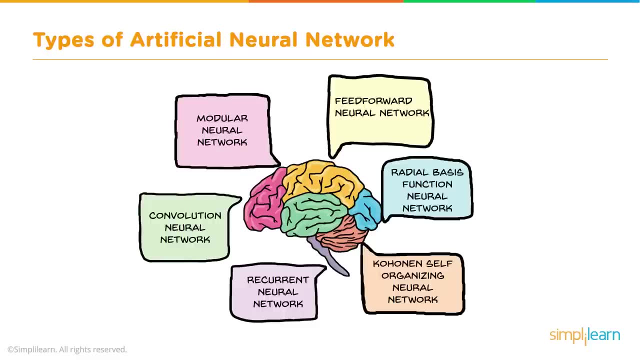 So if you're in the banking domain, It's going to be different than the medical domain, Than the automatic car domain, And suddenly figuring out how those all fit together Is just a lot of fun And really cool. So we have our types of artificial neural network. 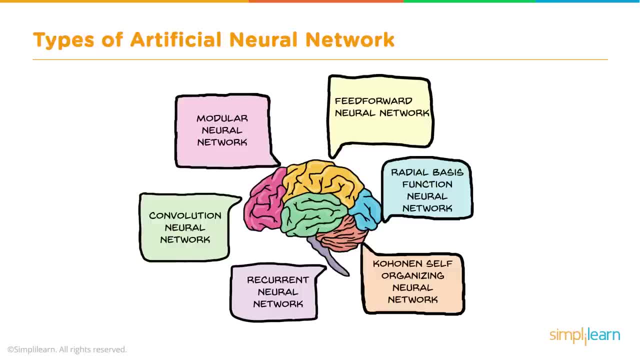 We have our feed forward neural network. We have a radial basis function neural network. We have our cohenin self organizing neural network, Recurrent neural network, Convolution neural network And modular neural network. So we have all of them all together. 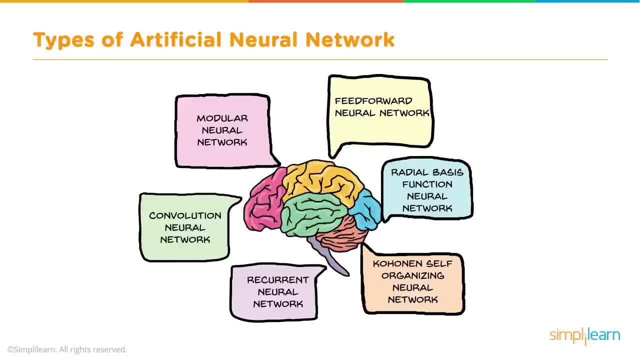 And know that colors on the brain Do not match what your brain actually does, But they do bring it out That most of these were developed By understanding how humans learn. And as we understand more and more Of how humans learn, We can build something in the computer industry. 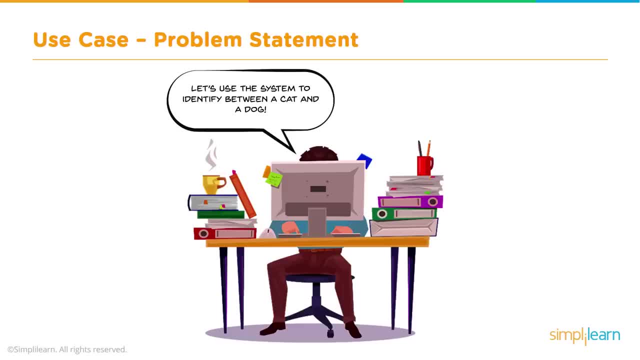 To mimic that, To reflect that, And that's how these were developed. So exciting part: Use case: Problem statement. So this is where we jump in. This is my favorite part. Let's use the system to identify Between a cat and a dog. 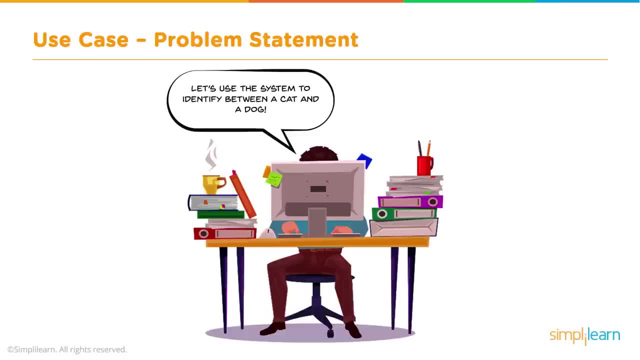 Correctly. I said we're going to do some python code And you can see over here My hair is kind of sticking up over the computer. A cup of coffee on one side And a little bit of old school- A pencil and a pen- on the other side. 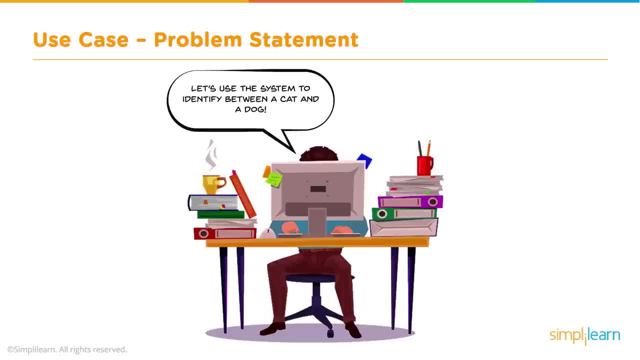 Most people now take notes. I love the stickies on the computer. That's great. That is my computer. I have sticky notes on my computer In different colors, So not too far from today's programmer. So the problem is We want to classify photos of cats and dogs. 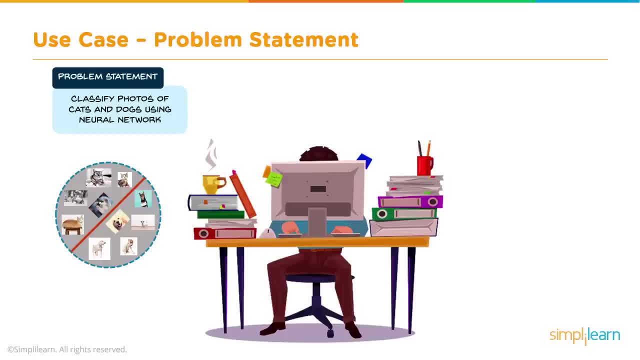 Using a neural network And you can see over here We have quite a variety of dogs in the pictures And cats And just sorting out, It is a cat. It's pretty amazing And why would anybody want to even know The difference between a cat and a dog? 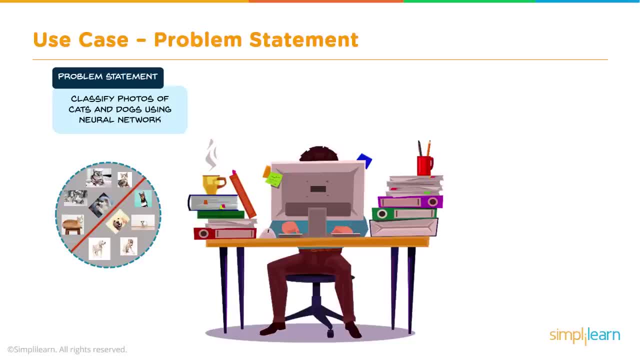 Okay, You know why? Well, I have a cat door. It would be kind of fun That, instead of it identifying, Instead of having like a little collar With a magnet on it, Which is what my cat has- The door would be able to see. 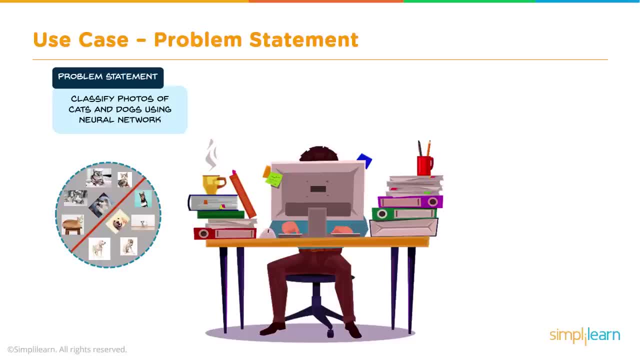 Oh, that's the cat. That's our cat coming in. Oh, that's the dog. We have a dog too. That's the dog I want to let in. Maybe I don't want to let this other animal in Because it's a raccoon. 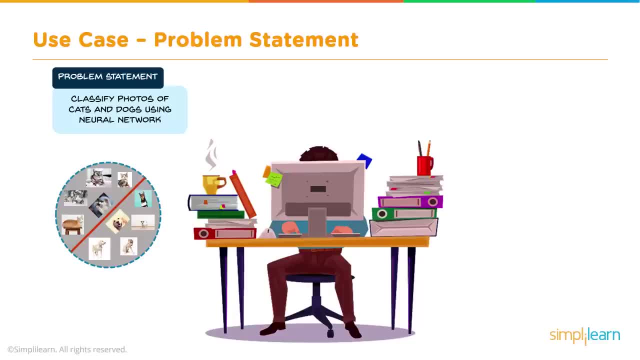 You can see where you could take this one step further And actually apply this. You could actually start a little startup company idea Self identifying door. So this use case will be implemented on Python. I am actually in Python 3.6.. 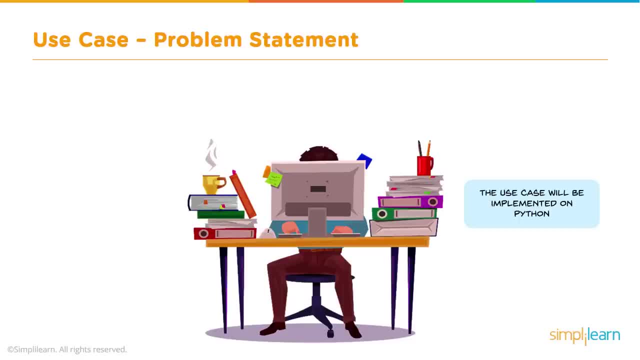 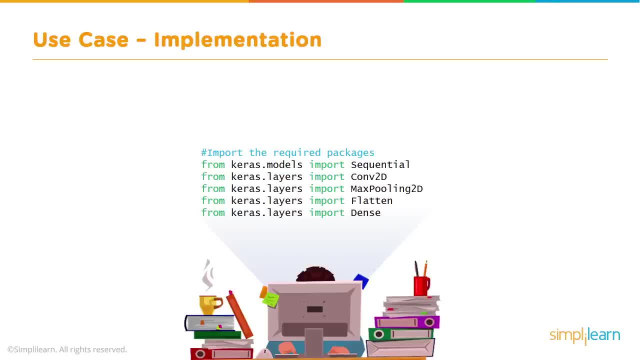 It's always nice to tell people the version of Python, Because it does affect sometimes which modules you load and everything. And we're going to start by importing the required packages. I told you we're going to do this in Keras, So we're going to import from Keras models. 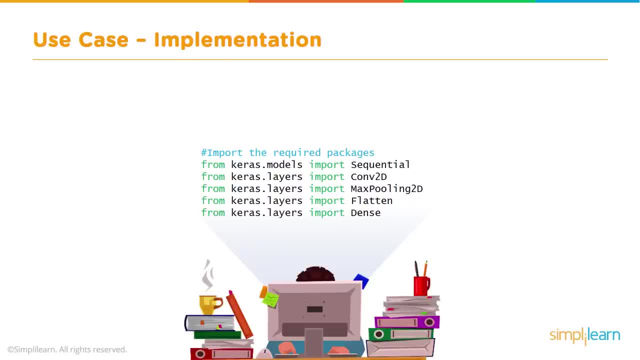 A sequential from the Keras layers: Conversion 2D or CONV 2D, Max pooling 2D, Flatten and Dense, And we'll talk about what each one of these do in just a second. But before we do that, 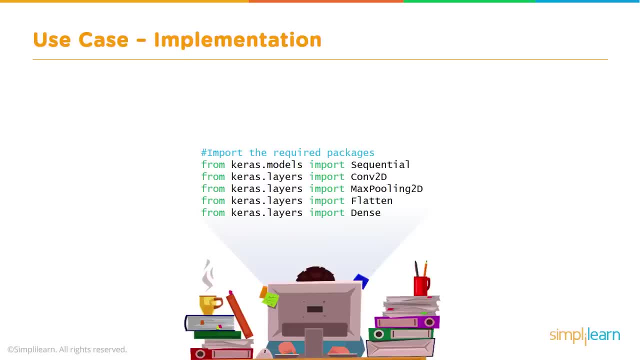 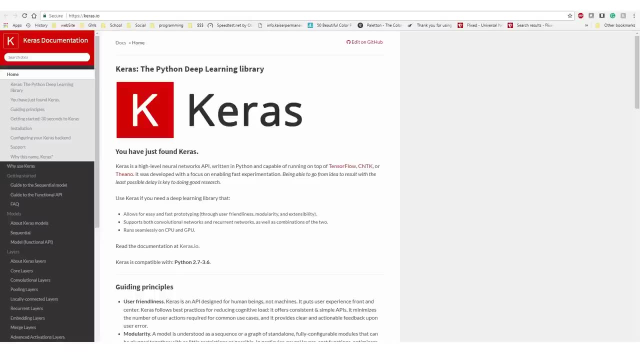 Let's talk a little bit about the environment we're going to work in, And you know. in fact, Let me go ahead and open the website Keras' website, So we can learn a little bit more about Keras. So here we are on the Keras website. 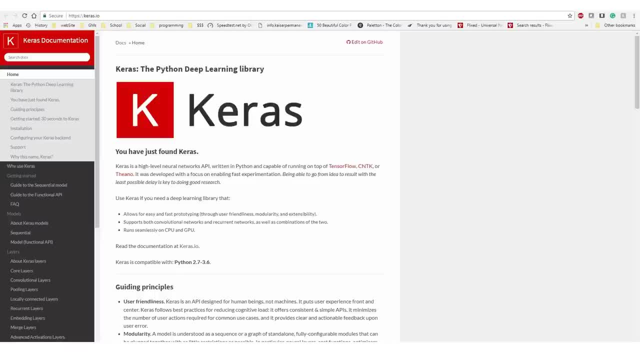 And it's Kerasio. That's the official website for Keras, And the first thing you'll notice Is that Keras runs on top of Either TensorFlow, CNTK, And I think it's pronounced Thano Or Thiano. 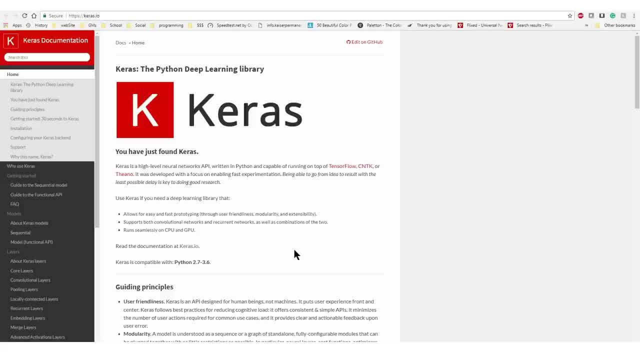 What's important on here Is that TensorFlow- And the same is true for all these, But TensorFlow is probably one of the most widely used Currently packages out there with the Keras And of course, you know, Tomorrow this is all going to change. 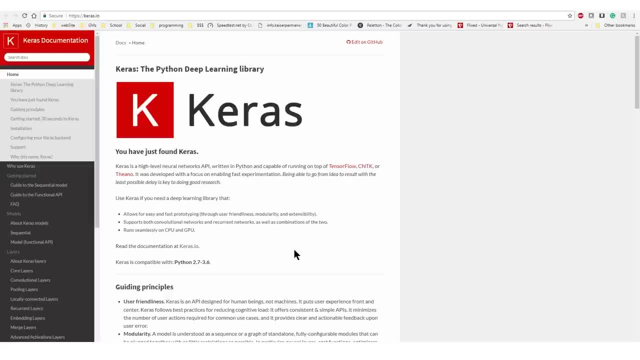 It's all going to disappear And they'll have something new out there. So make sure, when you're learning this code, That you understand what's going on And also know the code. I mean When you look at the code, It's not as complicated. 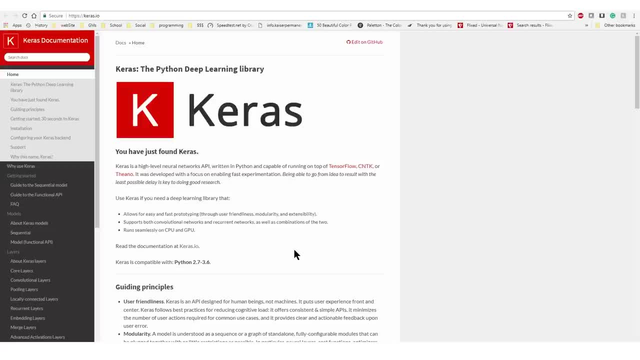 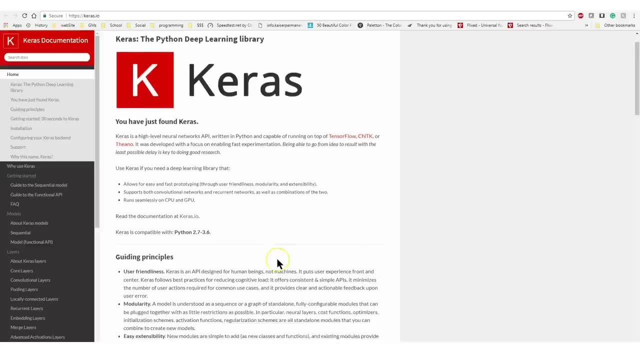 Once you understand what's going on, The code itself is pretty straightforward, And the reason we like Keras And the reason that people are jumping on it right now And it's such a big deal, Is if we come down here. Let me just scroll down a little bit. 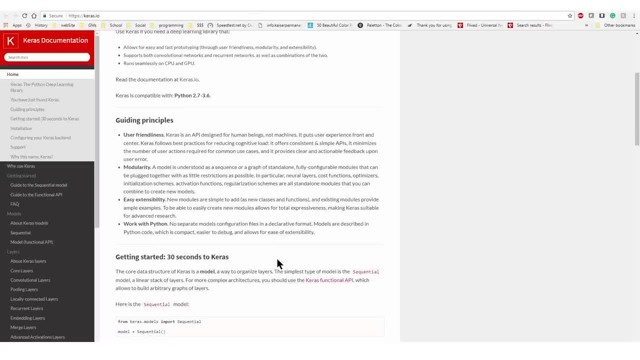 They talk about user friendliness, Modularity, Easy extensibility, Work with Python. Python's a big one Because a lot of people in data science now use Python. Although you can actually access Keras other ways Is if we continue down here. 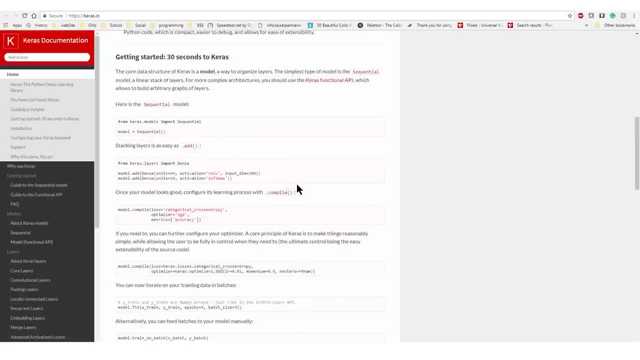 Is layers, And this is where it gets really cool. When we're working with Keras, You just add layers on. Remember those hidden layers we were talking about? And we talked about the RELU activation You can see right here. Let me just up that a little bit in size. 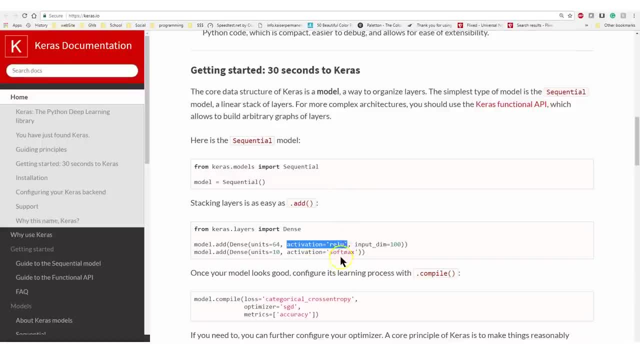 There we go. That's big, I can add in an RELU layer And then I can add in a softmax layer, The next instance. We didn't talk about softmax, So you can do each layer separate. Now, if I'm working in some of the other kits I use, 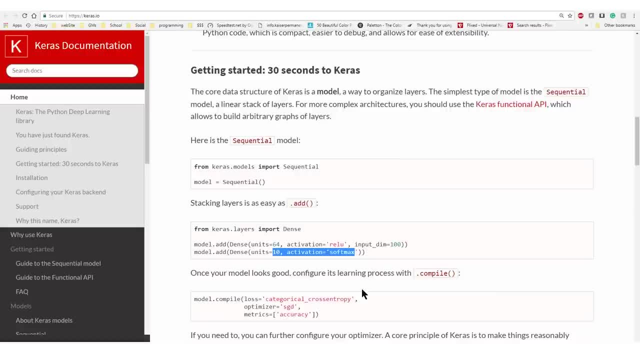 I take that And I have one setup And then I feed the output into the next one. This one Just add hidden layer after hidden layer with the different information in it, Which makes it very powerful And very fast to spin up and try different setups. 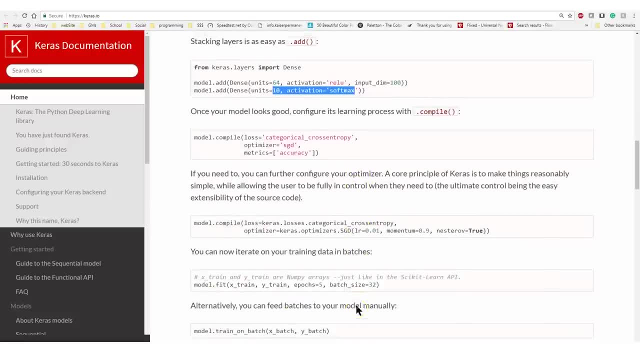 And see how they work with the data you're working on, And we'll dig a little bit deeper in here, And a lot of this is very much the same. So when we get to that part, I'll point that out to you also. 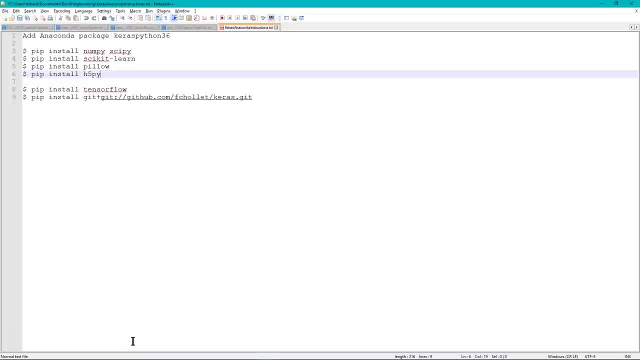 Now just a quick side note. I'm using Anaconda with Python in it And I went ahead and created my own package And I called it the Keras Python 3.6.. Because I'm in Python 3.6.. Anaconda is cool that way. 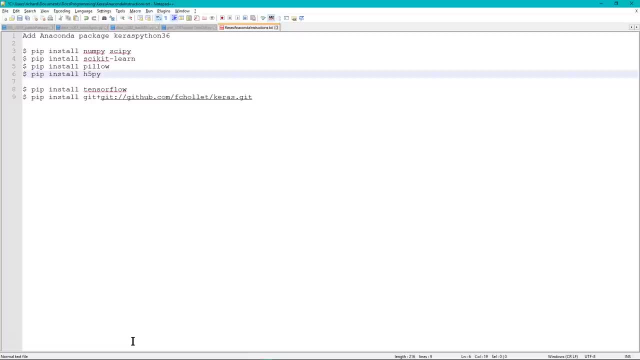 You can create different environments really easily. If you're doing a lot of different, experimenting with these different packages, You probably want to create your own environment in there, And the first thing is: you can see right here There's a lot of dependencies. 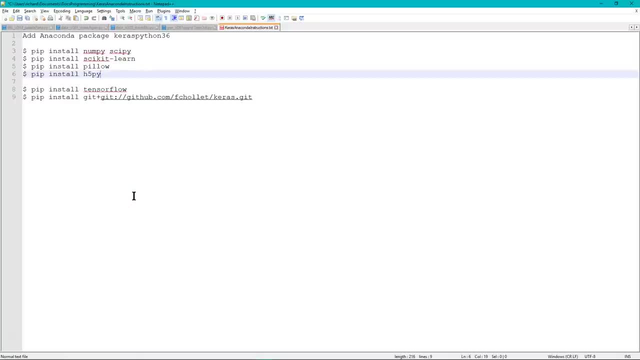 A lot of these. you should recognize by now If you've done any of these videos. If not, Kudos for you for jumping in today. pip, install numpy scipy. The scikit-learn Pillow and h5py are both needed for the tensor flow. 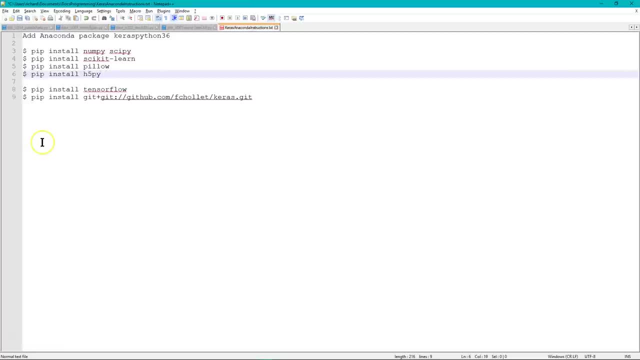 And then putting the Keras on there, And then you'll see here- And pip is just a standard installer That you use with Python- And you'll see here that we did pip install tensor flow, Since we're going to do Keras on top of tensor flow. 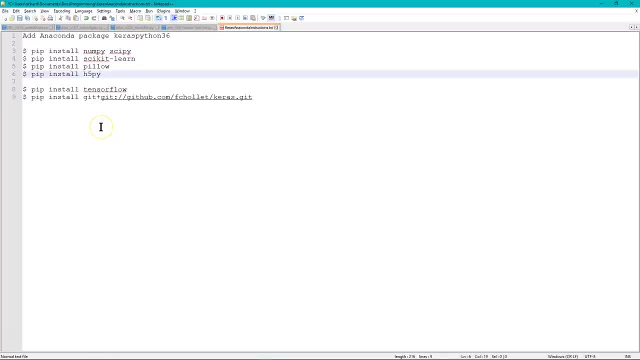 And then pip install And I went ahead and used the GitHub. So git plus git And you'll see here githubcom. This is one of their releases, One of the most current release on there, That goes on top of tensor flow. 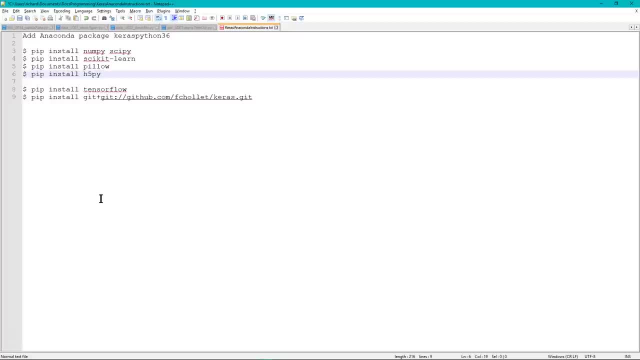 And you can look up these instructions pretty much anywhere. This is for doing it on Anaconda. Certainly you'd want to install these. If you're doing it in Ubuntu server setup, You'd want to get. I don't think you need the h5py in Ubuntu. 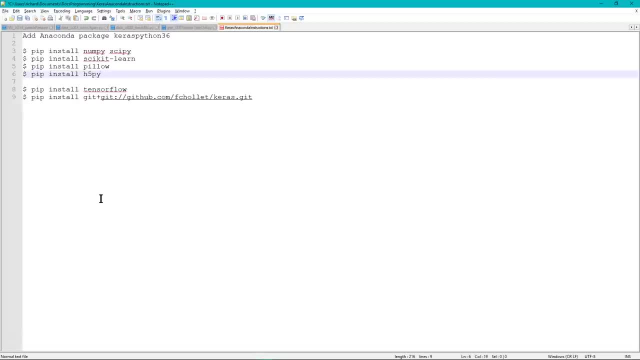 But you do need the rest in there Because there really are dependencies in there And it's pretty straight forward And that's actually in some of the instructions They have on their website, So you don't have to necessarily go through this. 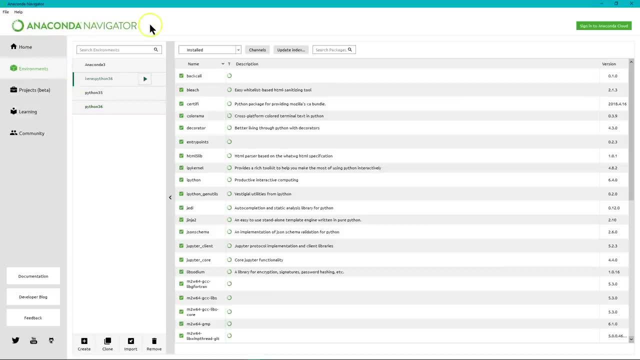 Just remember their website on there And then when I'm under my Anaconda navigator, Which I like, You'll see where I have environments, And on the bottom I created a new environment And I called it Keras, Python 36.. Just to separate everything. 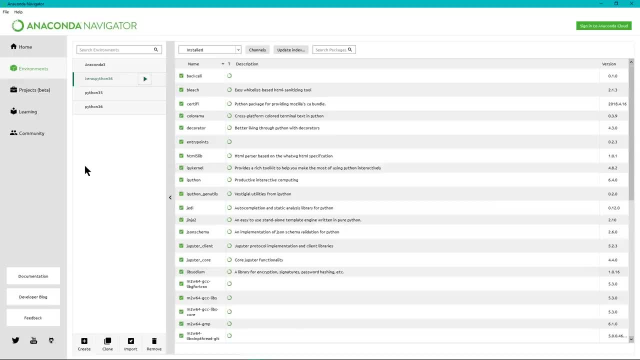 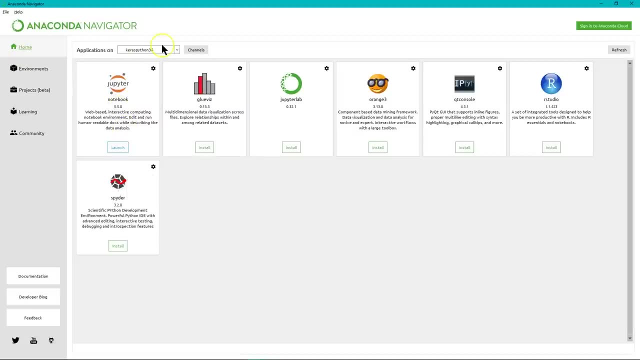 You can say I have Python 30.5 and Python 36.. I used to have a bunch of other ones, But I kind of cleaned house recently And, of course, once I go in here I launch my Jupyter Notebook, Making sure I'm using the right environment. 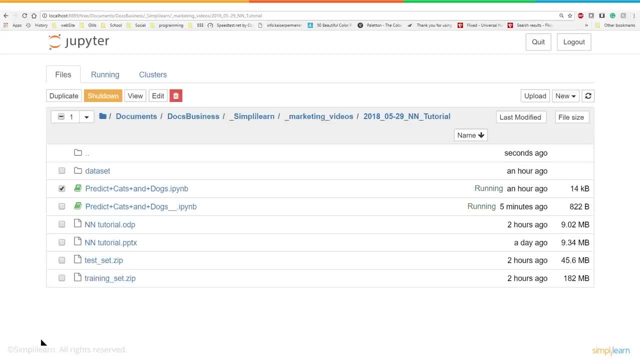 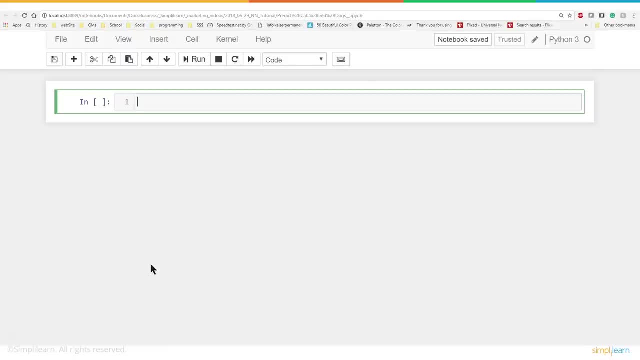 That I just set up. This, of course, opens up my- In this case I'm using Google Chrome- And in here I can go and just create a new document in here And this is all in your browser When you use the Anaconda. 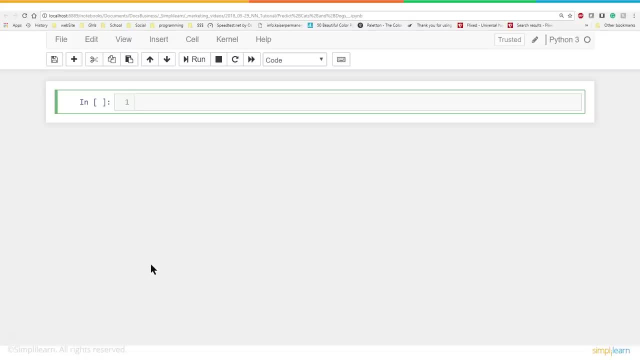 Do you have to use Anaconda in Jupyter Notebook? No, You can use any kind of Python editor, Whatever setup you're comfortable with And whatever you're doing in there. So let's go ahead and go in here And paste the code in. 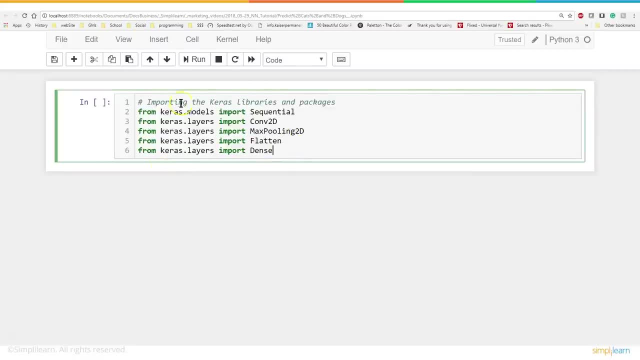 And we're importing a number of different settings in here. We have import sequential- That's under the models, Because that's the model we're going to use as far as our neural network. And then we have layers And we have conversion 2D. 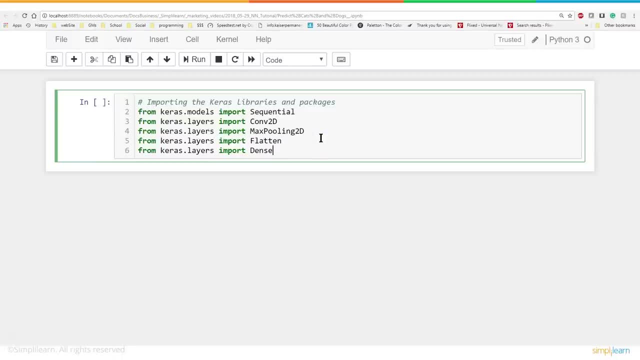 Max pooling 2D, Flatten, Dense, And you can actually just kind of guess at what these do. We're talking, We're working in a 2D photograph And, if you remember correctly, I talked about how the actual input layer is a single array. 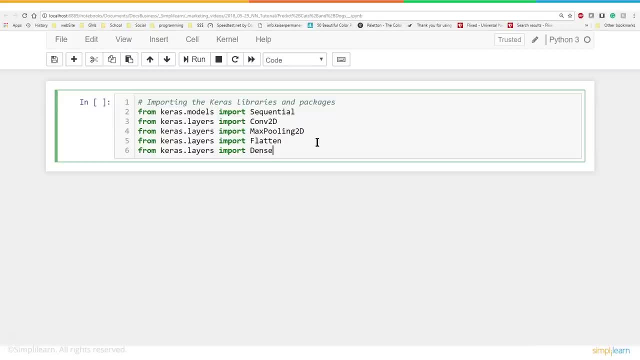 It's not in two dimensions, It's one dimension. All these do. These are tools to help flatten the image. So it takes a two dimensional image And then it creates its own proper setup. You don't have to worry about any of that. 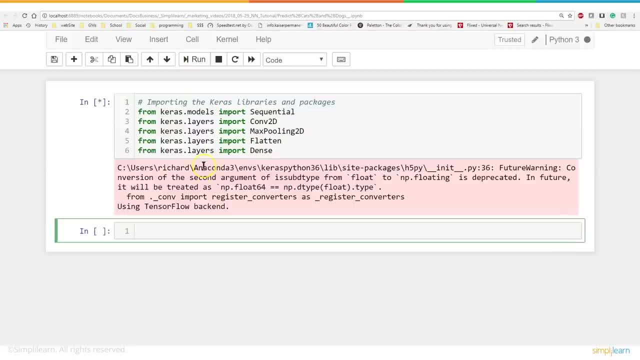 You don't have to do anything special with the photograph, You let the cross do it And we're going to run this And you'll see, right here They have some stuff that is going to be depreciated and changed, Because that's what it does. 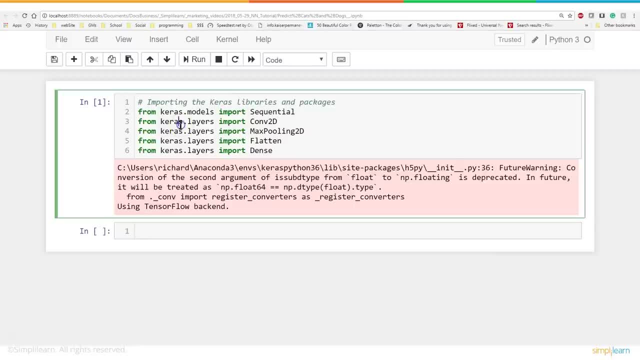 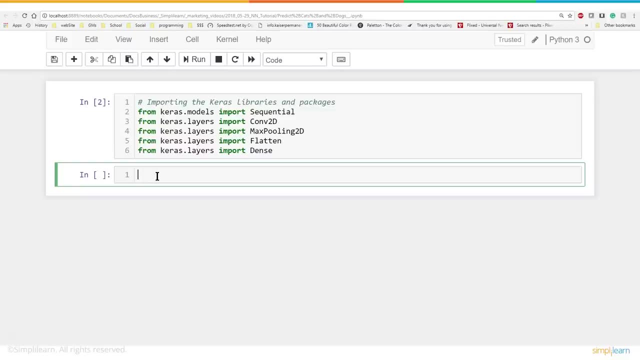 Everything is being changed as we go. You don't have to worry about that too much. If you have warnings, If you run it a second time, The warning will disappear, And this is just imported these packages for us to use. Jupyter is nice about this. 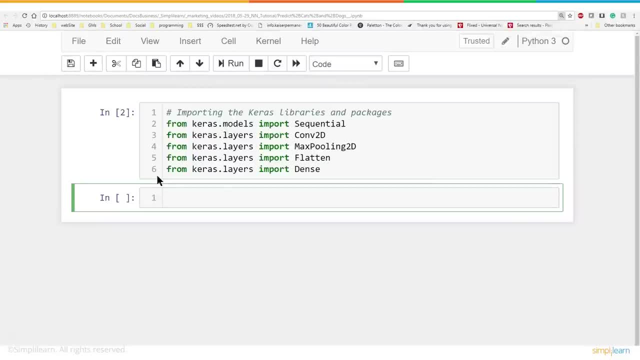 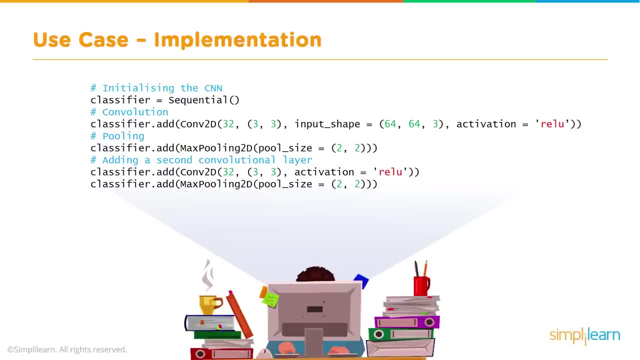 That you can do each thing step by step, And I'll go ahead and also zoom in there A little control plus. That's one of the nice things about being in a browser environment. So here we are back. Another sip of coffee. 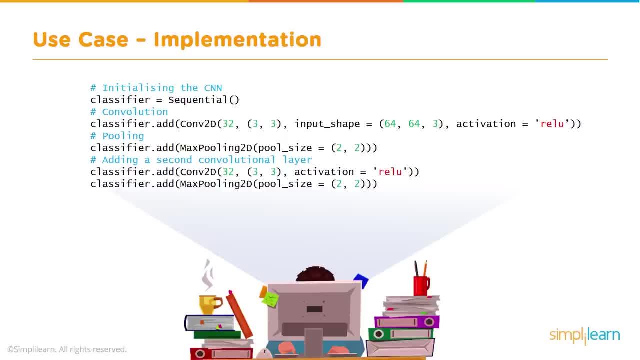 If you're familiar with my other videos, You'll notice I'm always sipping coffee. I always have in my case a latte, next to me An espresso. So the next step is to go ahead and initialize. We're going to call it the CNN. 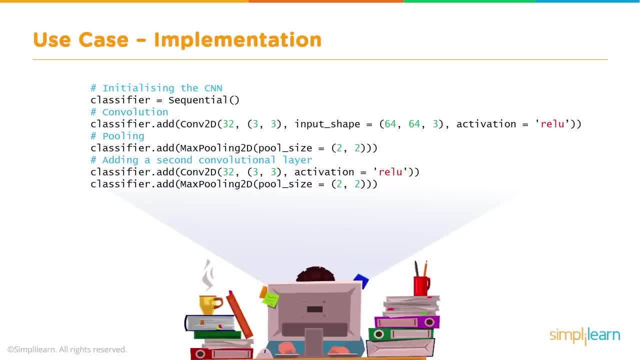 Or classifier neural network, And the reason we call it a classifier Is because it's going to classify it between two things: It's going to be cat or dog. So when you're doing classifiers, Classification, You're picking specific objects. It's a true or false. 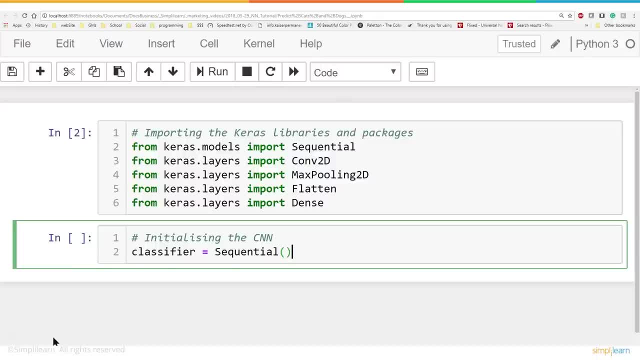 Yes, no, It is something or it's not. So, first thing, we're going to create our classifier And it's going to equal sequential. So their sequential setup is the classifier. That's the actual model we're using. That's the neural network. 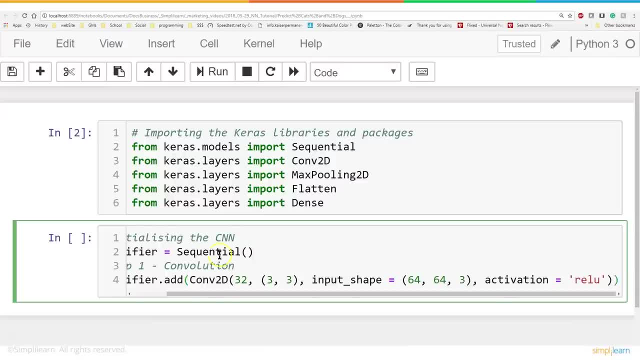 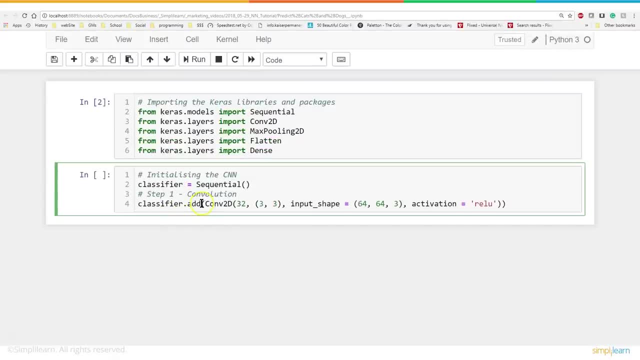 So we call it a classifier And the next step is to add in our convolution- And let me just do a, Let me shrink that down in size So you can see the whole line- And let's talk a little bit about what's going on here. 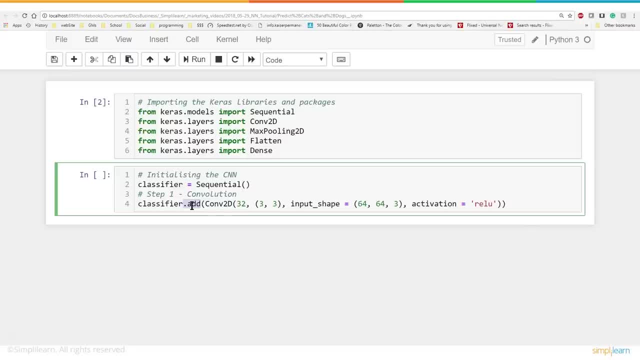 So I have my classifier And I add something. What am I adding? Well, I'm adding my first layer. This first layer we're adding in Is probably the one that takes the most work To make sure you have it set correct. 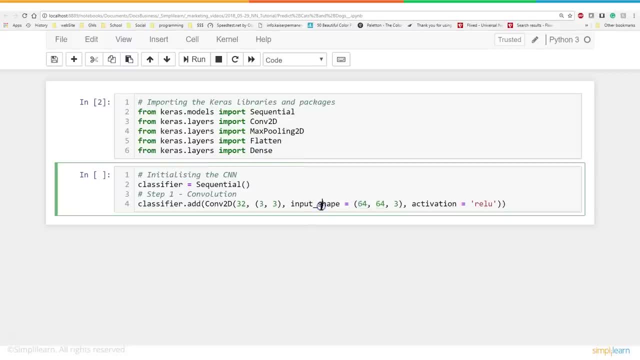 And the reason I say that This is your actual input, And we're going to jump here to the part that says: Input shape equals 64 by 64 by 3.. What does that mean? Well, that means That our picture's coming in. 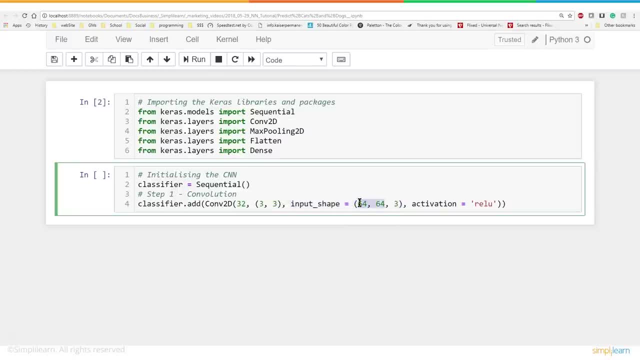 And there's these pictures. Remember we had like the picture of the car Was 128 by 128 pixels. Well, this one is 64 by 64 pixels And each pixel has three values. That's where these numbers come from, And it is so important. 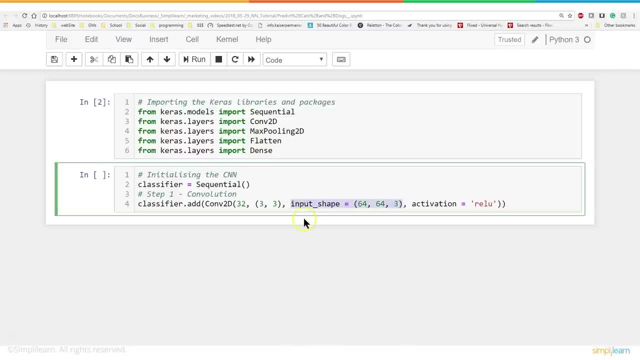 That this matches. I mentioned a little bit That if you have like a larger picture You have to reformat it to fit this shape. If it comes in as something larger, There's no input nodes. There's no input neural network there. 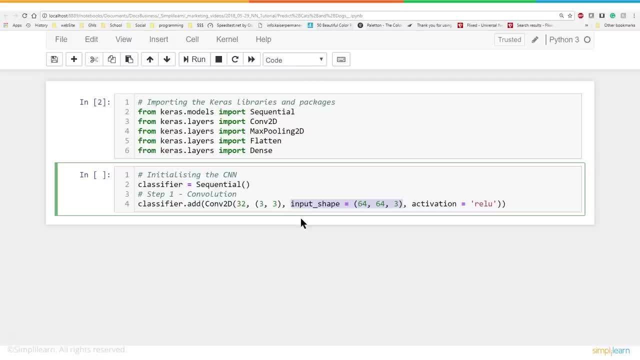 That will handle that extra space. So you have to reshape your data to fit in here. Now, the first layer is the most important, Because after that, Keras knows what your shape is coming in here And it knows what's coming out. 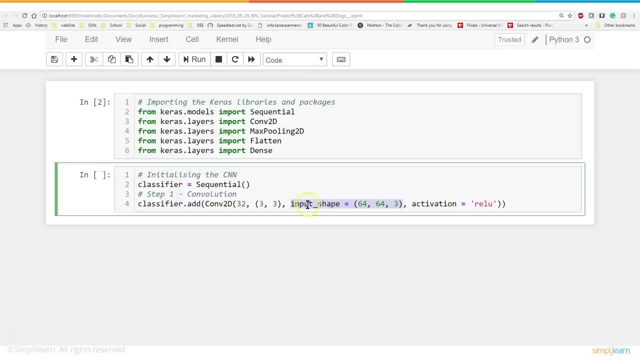 And so that really sets the stage. Most important thing is that input shape Matches your data coming in, And you'll get a lot of errors. if it doesn't, You'll go through there And picture number 55 doesn't match it correctly. 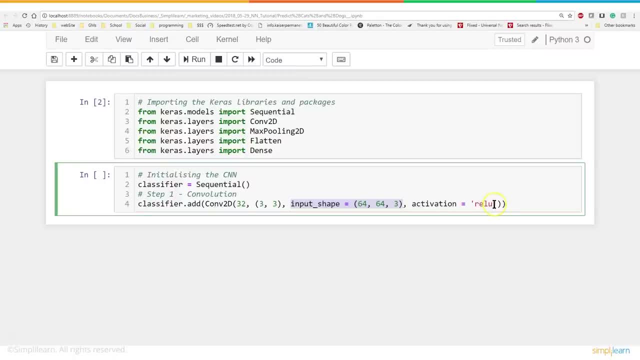 And guess what it does? It usually gives you an error. And then the activation. If you remember, We talked about the different activations on here. We're using the RELU model. Like I said, That is the most commonly used now. 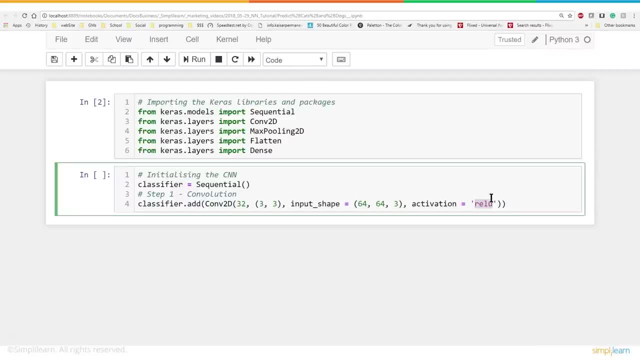 Because one- It's fast- Doesn't have the added calculations in it. It just says Here's the value coming out, Based on the weights And the value going in, And from there You know If it's over one. 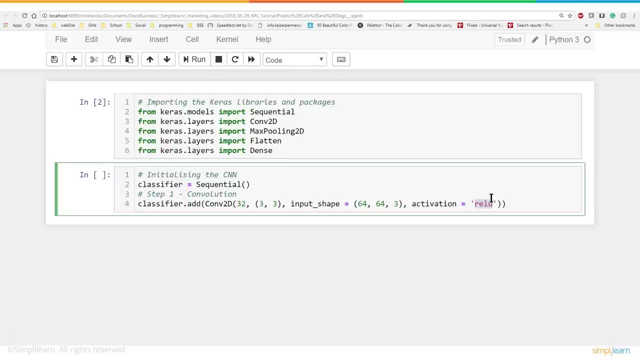 Then it's good Or over zero It's good. If it's under zero, Then it's considered not active. And then we have this conversion 2D. What the heck is conversion 2D? I'm not going to go into too much detail in this. 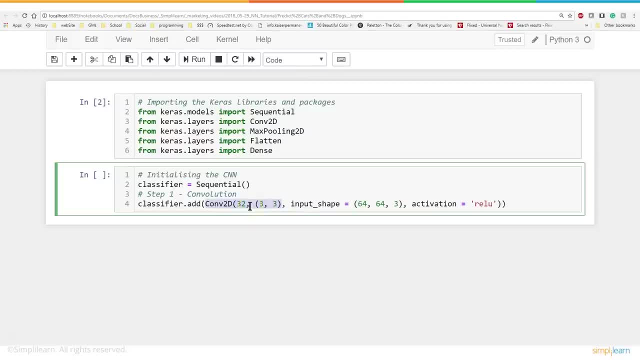 Because this has a couple of things it's doing in here A little bit more in depth And we're ready to cover in this tutorial. But this is used to convert from the photo Because we have 64 by 64 by 3.. 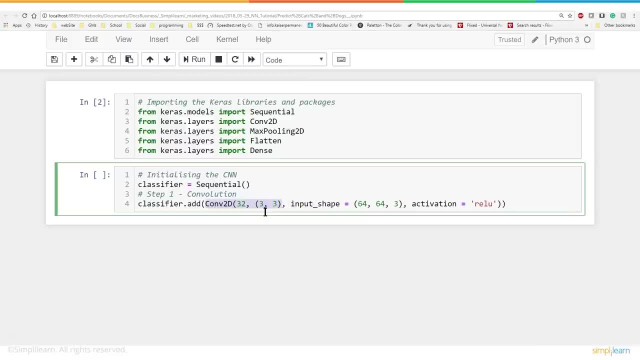 And we're just converting it to two-dimensional kind of setup. So it's very aware that this is a photograph And that different pieces are next to each other, And then we're going to add in a second convolutional layer. That's what the CONV stands for. 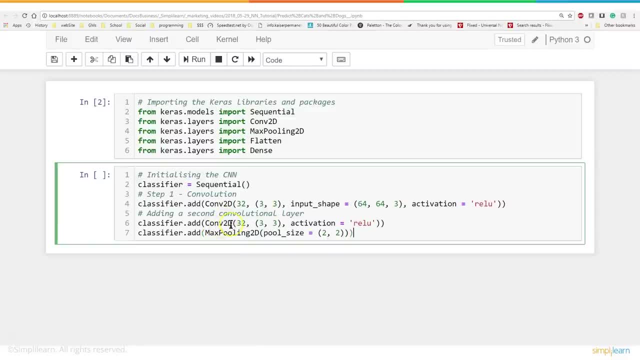 2D, So these are hidden layers. So we have our input layer And our two hidden layers And they are two-dimensional Because we're doing with a two-dimensional photograph And you'll see down here That we have two layers. 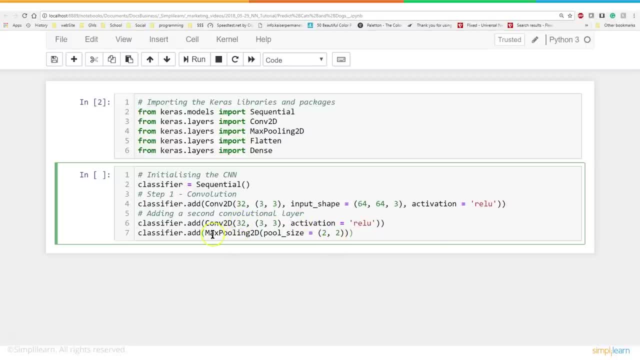 And we're going to add in A 2D photograph And you'll see down here That on the last one We add a max pooling 2D And we put a pool size equals 2, 2.. And so what this is. 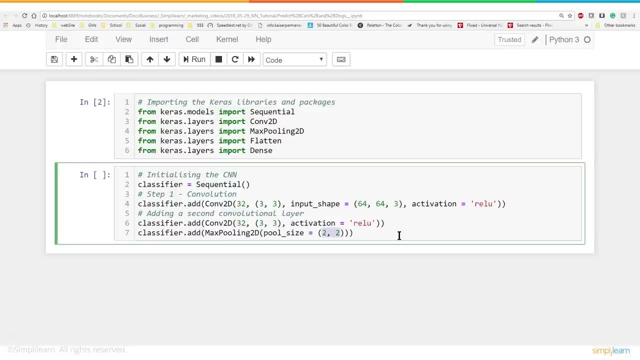 Is that, as you get to the end of these layers, One of the things you always want to think of Is what they call mapping and then reducing- Wonderful terminology from the big data. We're mapping this data through all these layers And now we want to reduce it to only two sets. 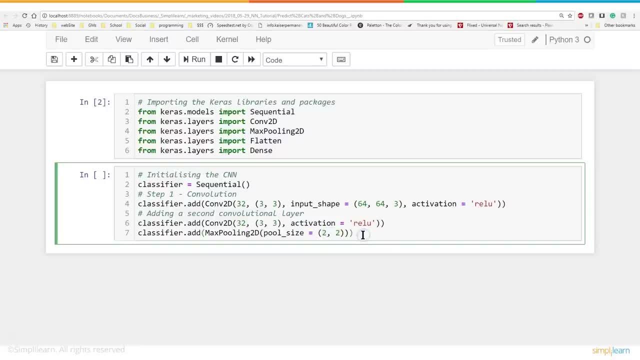 In this case it's already in two sets, Because it's a 2D photograph, But we had two dimensions. We actually have 64 by 64 by 3.. So now we're just getting it down to a 2 by 2.. 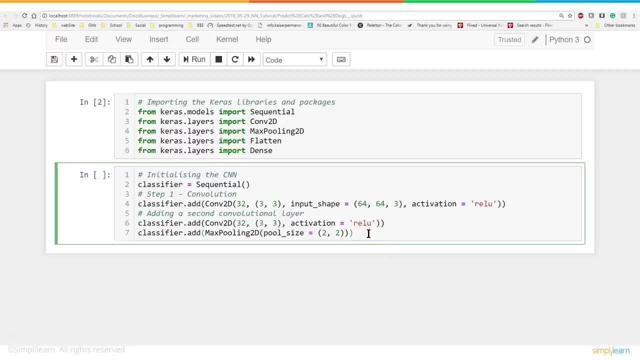 Just the two-dimensional and two-dimensional Instead of having the third dimension of colors, And we'll go ahead and run these. We're not really seeing anything on our run script Because we're just setting up. This is all set up And this is where you start playing. 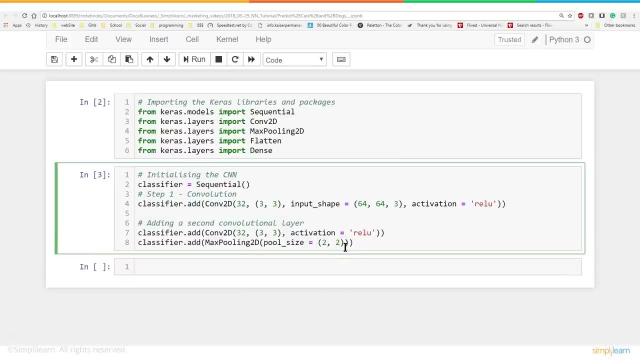 Because maybe you'll add a different layer in here To do something else, To see how it works And see what your output is. That's what makes Keras so nice Is I can, with just a couple flips of code, Put in a whole new layer. 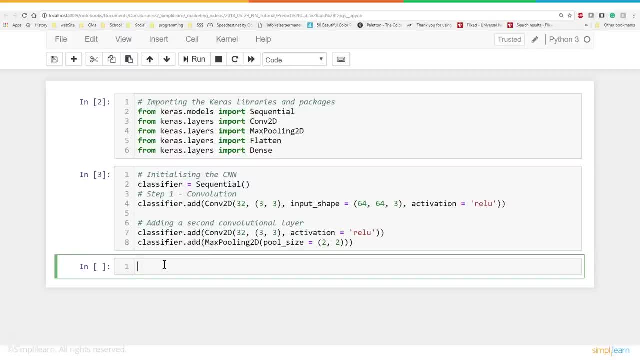 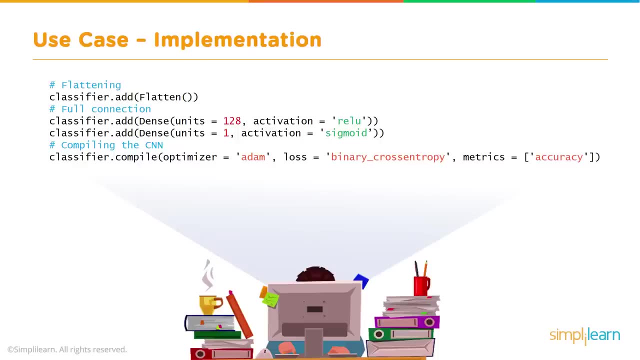 That does a whole new processing And see whether that improves my run Or makes it worse. And finally we're going to do the final setup, Which is to flatten Classifier, add a flatten setup, And then we're going to also add a layer. 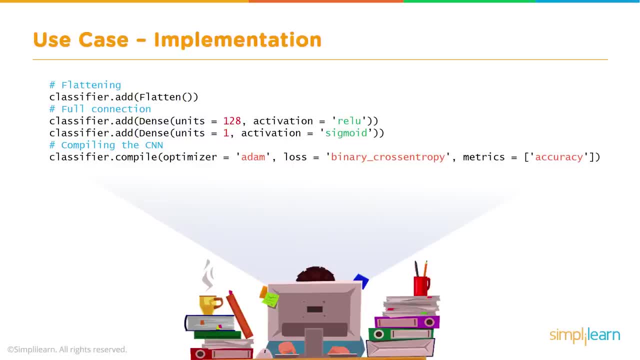 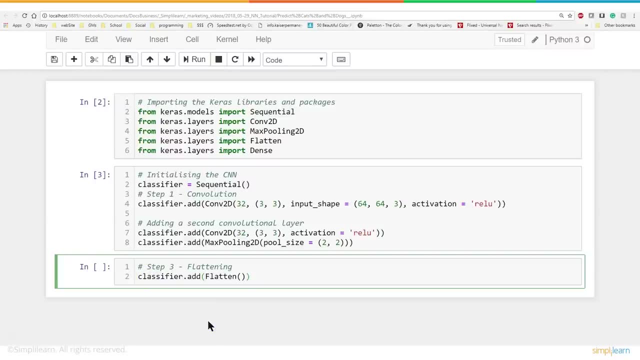 A dense layer, And then we're going to add in another dense layer And then we're going to build it. We're going to compile this whole thing together. So let's flip over and see what that looks like, And we've even numbered them for you. 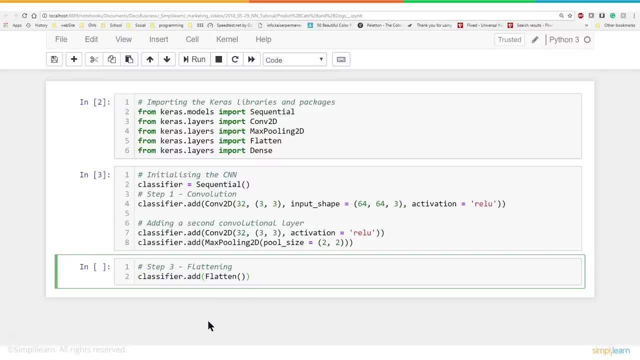 So we're going to do the flattening, And flatten is exactly what it sounds like. We've been working in a two-dimensional array of picture Which actually is in three dimensions Because of the pixels. The pixels have a whole other dimension to it. 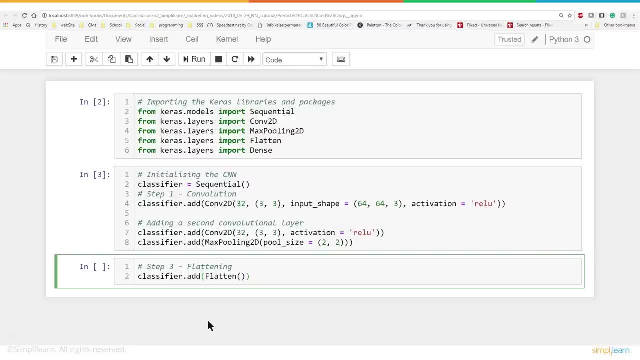 Of three different values And we've kind of resized those down to two by two. But now we're just going to flatten it. I don't want to have multiple dimensions being worked on By tensor and by Keras, I want just a single array. 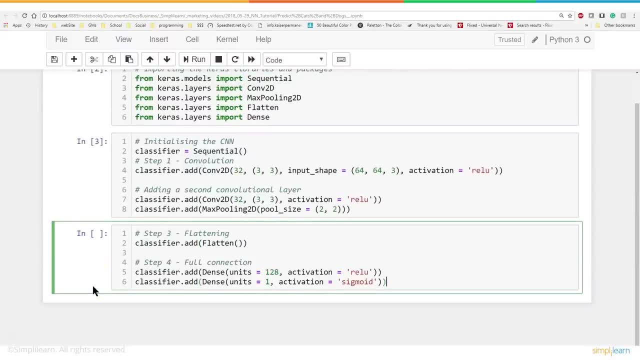 So it's flattened out. And then step four, Full connection. So we add in our final two layers And you could actually do all kinds of things with this. You could actually leave out some of these layers And play with them. You do need to flatten it. 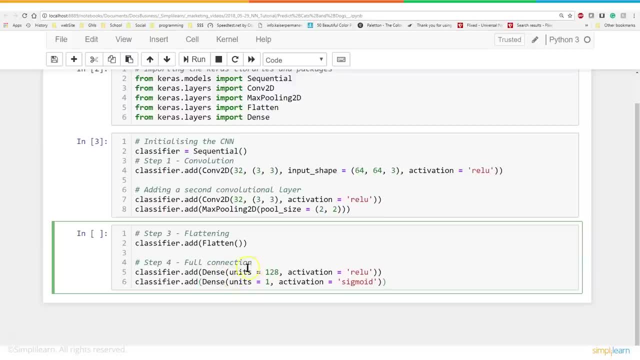 That's a good thing. It's very important. Then we want to use the dents. Again, we're taking this And we're taking whatever came into it. So once we take all those different, The two dimensions or three dimensions, as they are, 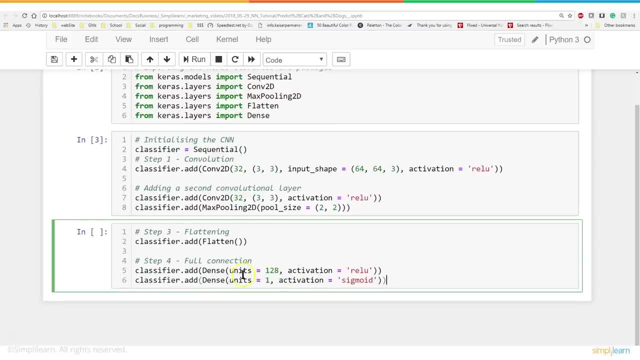 And we flatten it to one dimension. We want to take that And we're going to pool it into units of 128.. They got that. You're going to say: where did they get 128 from? You could actually play with that number. 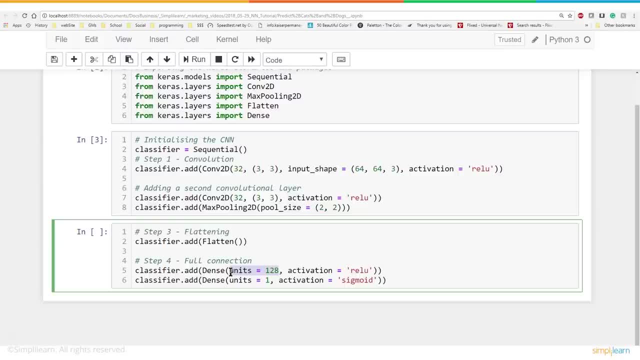 And get all kinds of weird results. But in this case We took the 64 plus 64 is 128.. You could probably even do this with 64 or 32.. But you want to keep it in the same multiple. Whatever the data shape you're already using is in. 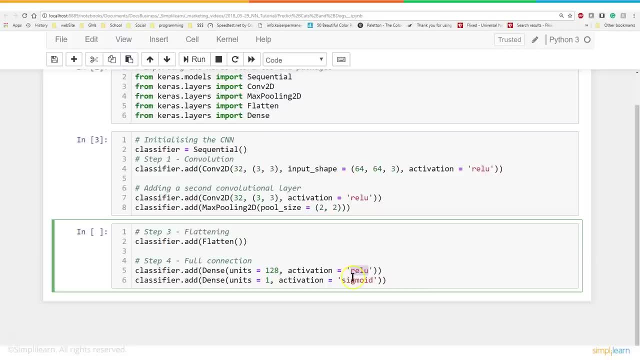 And we're using the activation, The RELU, Just like we did before, And then we finally filter all that into a single output. And it has how many units One? Why? Because we want to know whether true or false. It's either a dog or a cat. 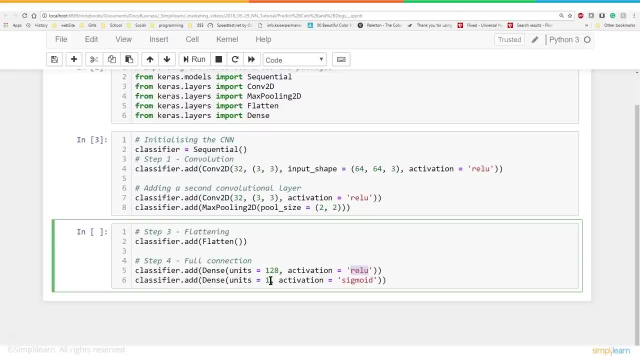 You could say: one is dog, Zero is cat, Or maybe you're a cat lover And it's: one is cat And zero is dog, And if you love both dogs and cats, You're going to have to choose. And then we use the sigmoid activation. 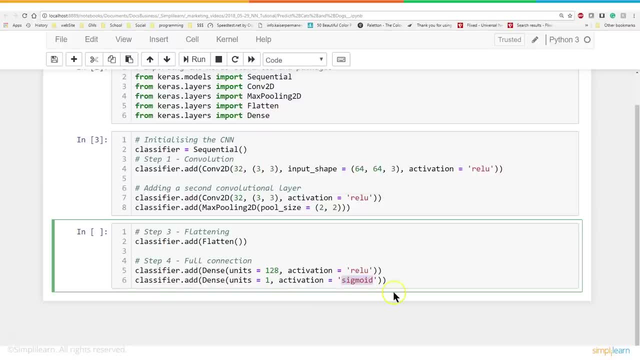 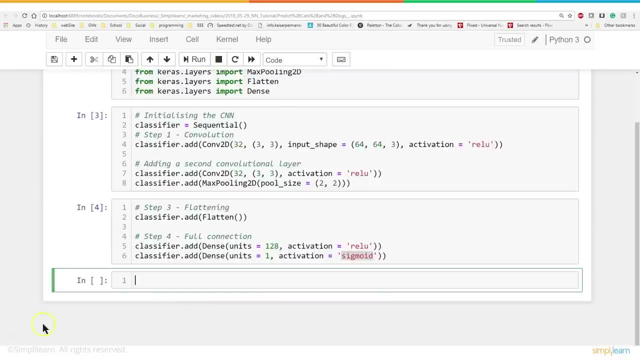 If you remember from before, We had the RELU And there's also the sigmoid. The sigmoid just makes it clear It's yes or no. We don't want any kind of in between number coming out And we'll go ahead and run this. 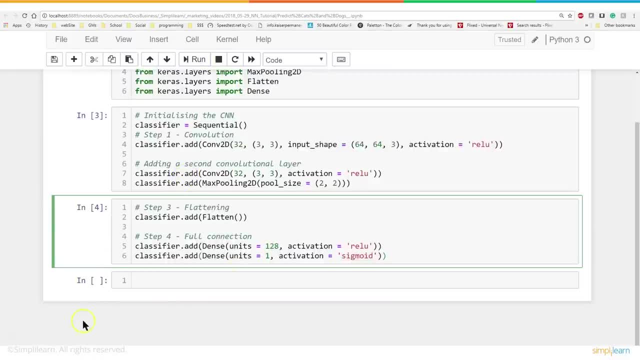 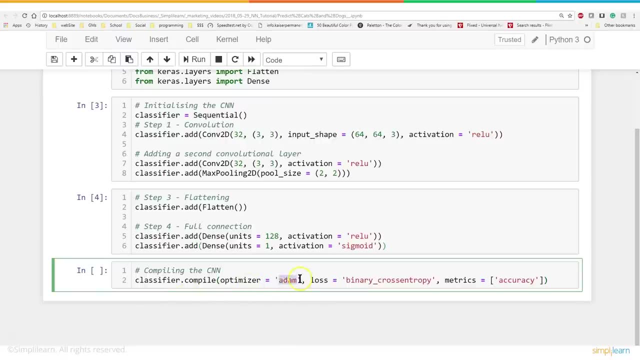 And you'll see it's still all in setup. And then, finally, we want to go ahead and compile And let's put the compiling our classifier neural network, And we're going to use the optimizer atom. And I hinted at this just a little bit before. 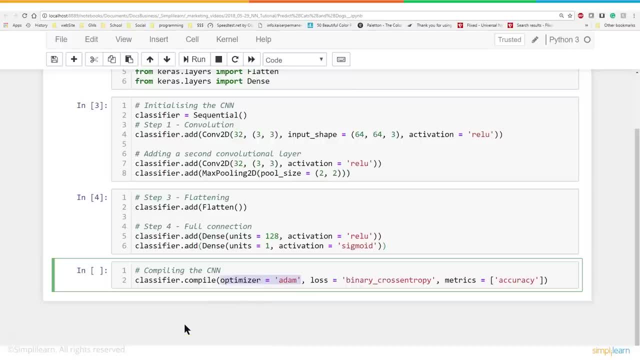 Where does atom come in? Where does an optimizer come in? Well, the optimizer is the reverse propagation. When we're training it, It goes all the way through and says error. And then how does it readjust those weights? There are a number of them. 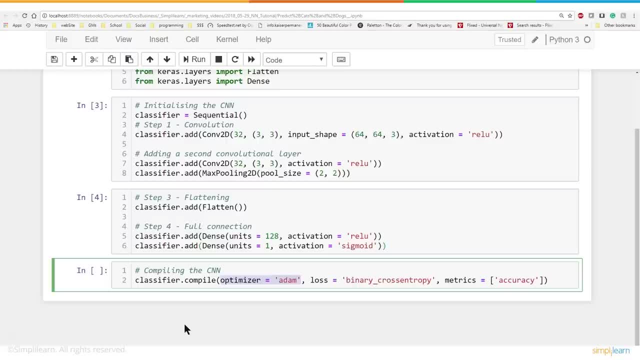 Atom is the most commonly used And it works best on large data. Most people stick with the atom Because when they're testing on smaller data, See if their model is going to go through And get all their errors out Before they run it on larger data sets. 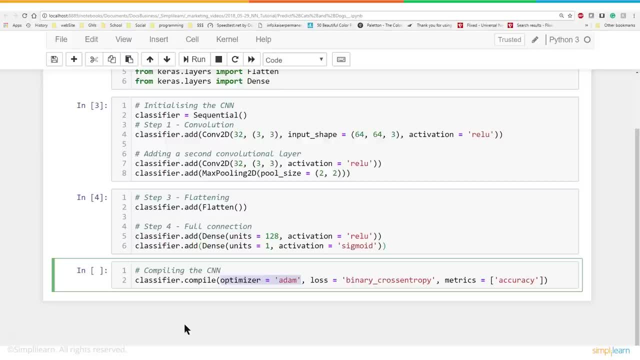 They're going to run it on atom anyway, So they just leave it on atom- Most commonly used. But there are some other ones out there. You should be aware of that That. you might try them If you're stuck in a bind. 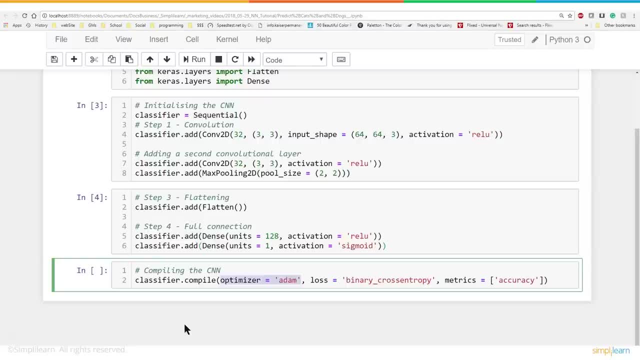 Or you might floor that in the future, But usually atom is just fine on there. And then you have two more settings. You have loss and metrics. We're not going to dig too much into loss or metrics. These are things you really have to explore cross. 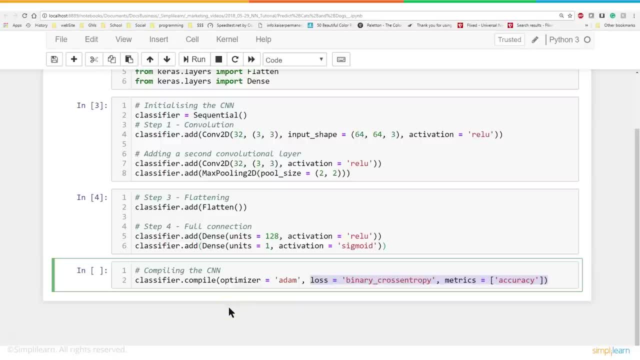 Because there are so many choices. This is how it computes the error. There's so many different ways to on your back, Propagation and your training, So we're using the atom model, But you can compute the error by standard deviation. Standard deviation squared. 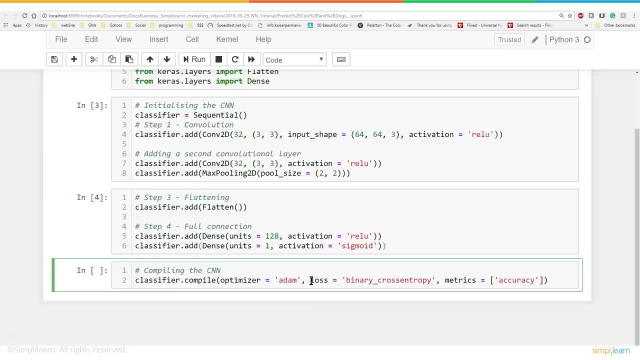 They use binary cross entropy. I'd have to look that up to even know what that is. There's so many of these. A lot of times you just start with the ones that look correct, That are most commonly used, And then you have to go read the cross site. 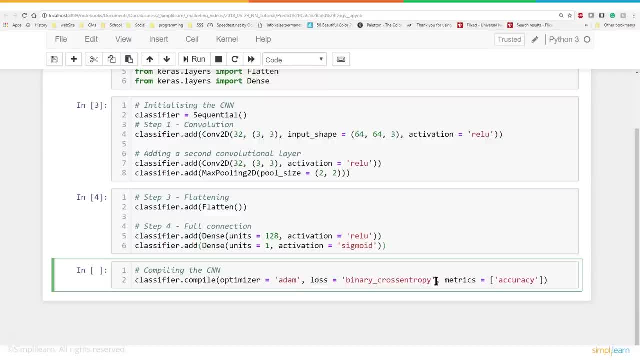 And actually see what these different losses and metrics And what different options they have. So we're not going to get too much into them, Other than to reference you over to the cross website To explore them deeper. But we are going to go ahead and run them. 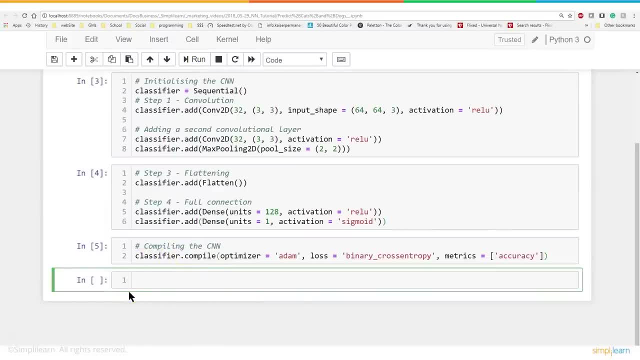 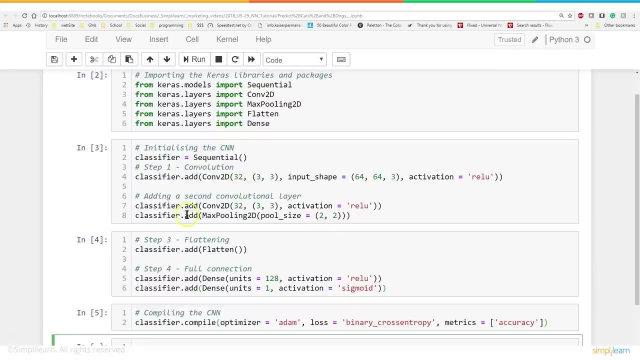 And now we've set up our classifier. So we have an object classifier And if you go back up here You'll see that we've added in Step one. we added in our layer for the input, We added a layer that comes in there. 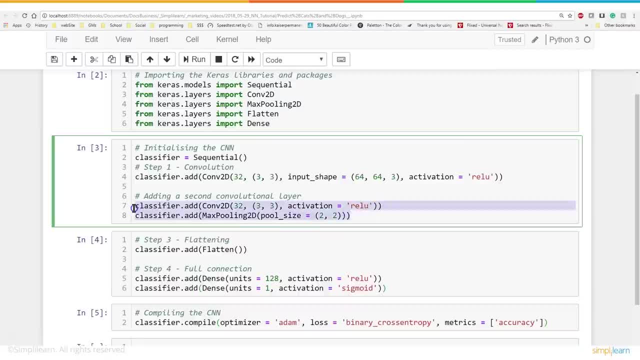 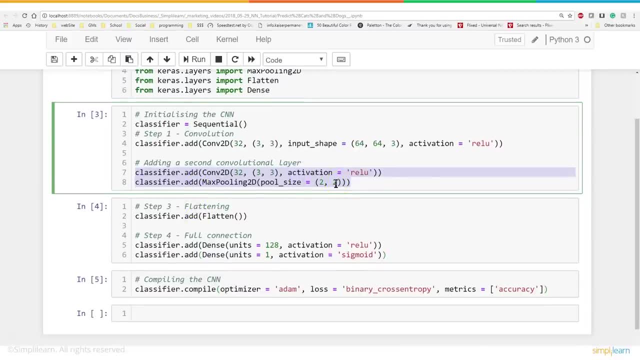 And uses the RELU for activation And then it pulls the data. So this is, Even though these are two layers- The actual neural network layer is up here- And then it uses this to pull the data into a two by two, So into a two dimensional array. 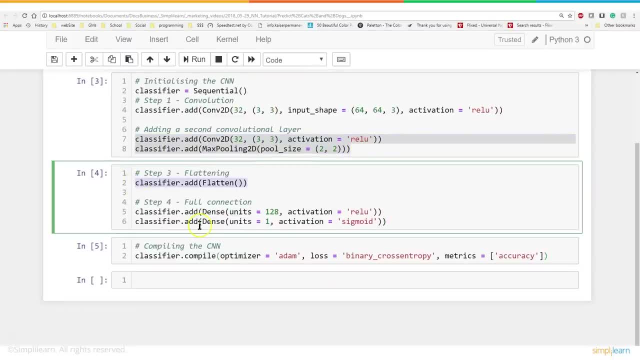 From a three dimensional array with the colors. Then we flatten it. So there's our add or flatten And then we add another dense, What they call dense layer. This dense layer goes in there And it downsizes it to 128.. 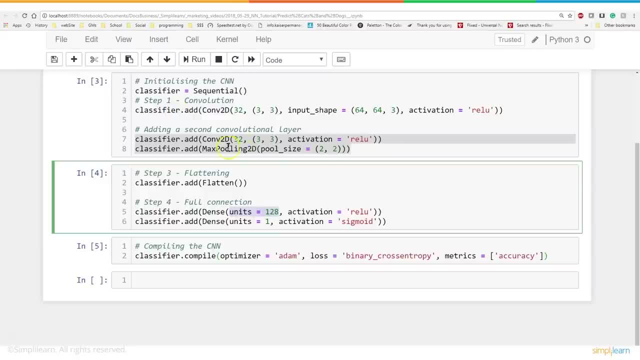 It reduces it. So you can look at this As we're mapping all this data down, The two dimensional setup, And then we flatten it. So we map it to a flatten map And then we take it And reduce it down to 128.. 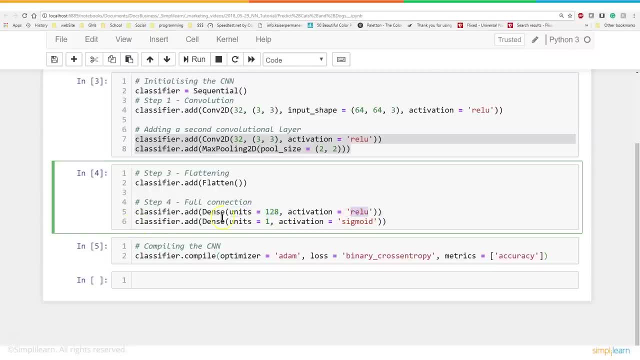 And we use the RELU again And then finally we reduce that down To just a single output And we use a sigmoid to do that, To figure out whether it's yes, no, true, false- In this case, cat or dog. 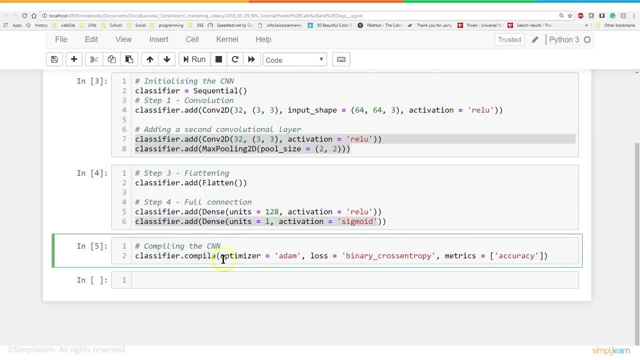 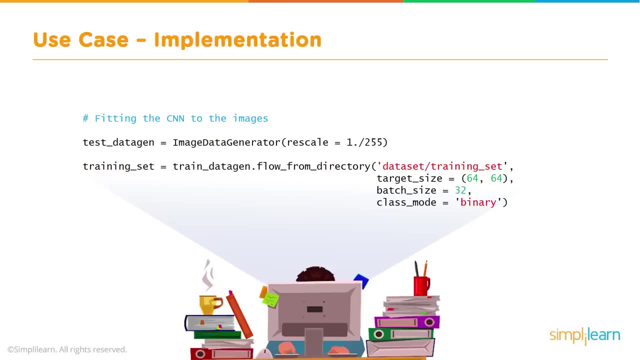 And then finally, once we put all these layers together, We compile them. That's what we've done here, And we've compiled them As far as how it trains To use these settings for the training Backpropagation. So, if you remember, 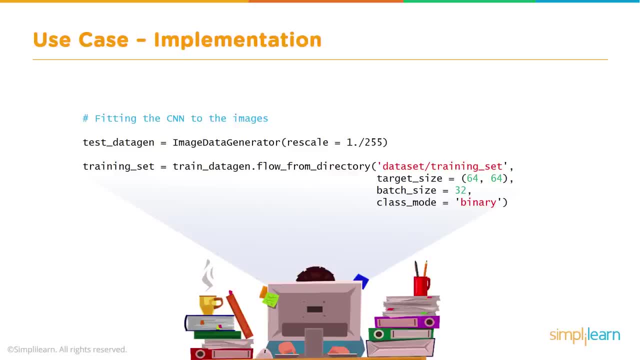 We talked about training our setup And when we go into this, You'll see that we have two data sets. We have one called the training set And the testing set, And that's very standard in any data processing Is you need to have? 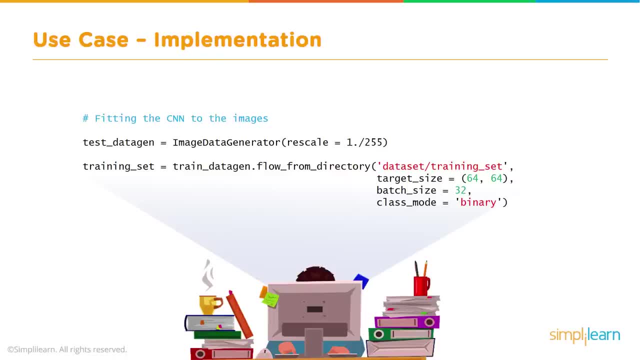 That's pretty common in any data processing Is you need to have a certain amount of data To train it, And then you got to know whether it works or not. Is it any good? And that's why you have a separate set of data. 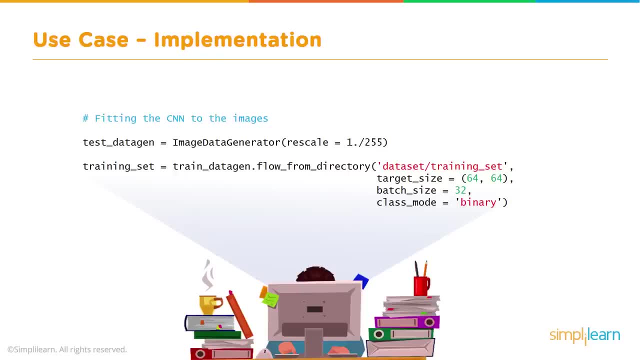 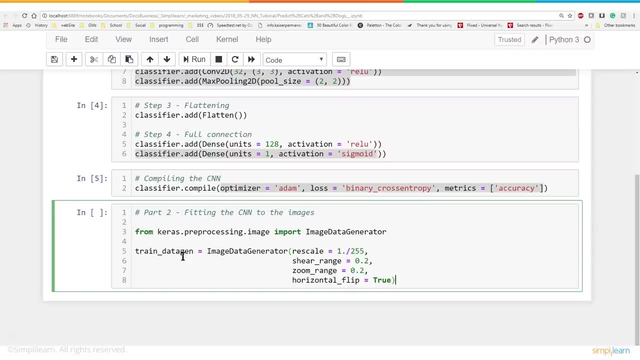 For testing it, Where you already know the answer. But you don't want to use that as part of the training set. So in here we jump into part two, Fitting the classifier neural network to the images, And then from Keras: 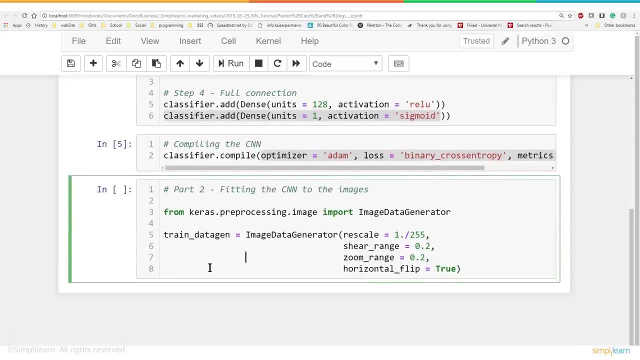 Let me just zoom in there. I always love that about working with Jupyter Notebook. So you can really see We're going to come in here, We do the cross pre-processing an image And we import image data generator. It's so nice of Keras. 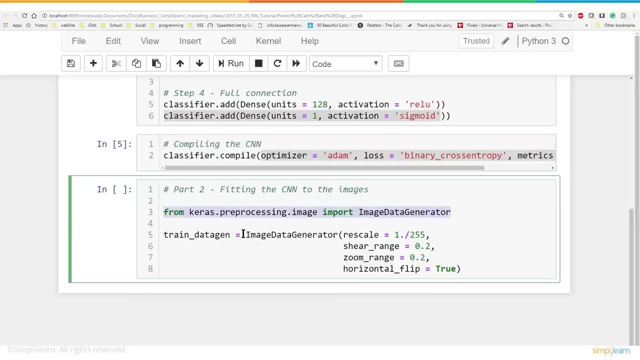 It's such a high end product right now Going out And since images are so common, They already have all this stuff to help us process the data, Which is great. And so we come in here, We do train data gen And we're going to create our object. 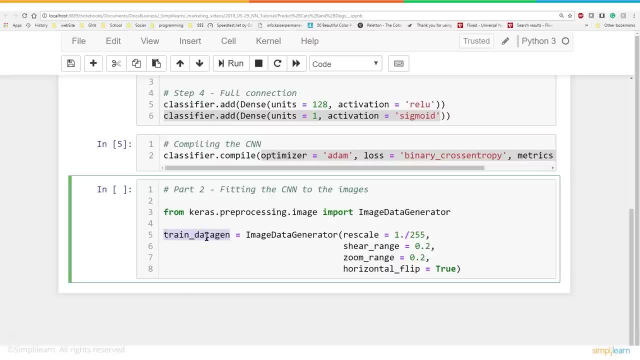 For helping us train it, For reshaping the data So that it's going to work with our setup And we use an image data generator And we're going to rescale it And you'll see, here We have one point. 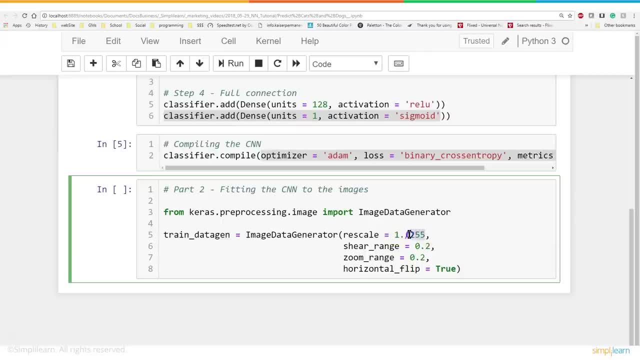 Which tells us it's a float value On the rescale over 255.. Where does 255 come from? Well, that's the scale In the color scale Of the pictures. we're using Their value from 0 to 255.. 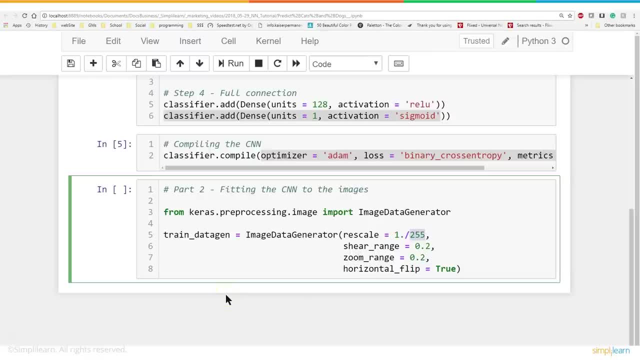 So we want to divide it by 255. And it will generate a number between 0 and 1.. They have shear range And zoom range. Horizontal flip equals true, And this of course, has to do with If the photos are different shapes and sizes. 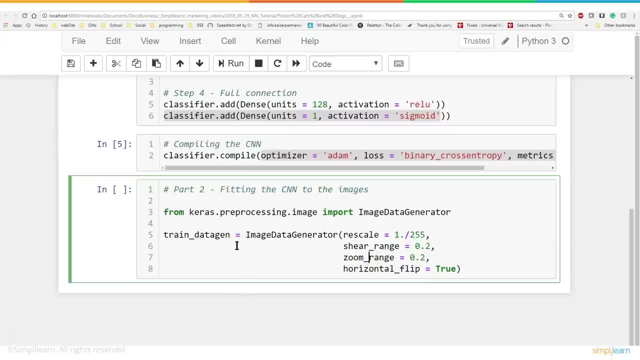 Like I said, it's a wonderful package. You really need to dig in deep To see all the different options you have For setting up your images. For right now, though, We're going to stick with some basic stuff here, And let me go ahead and run this code. 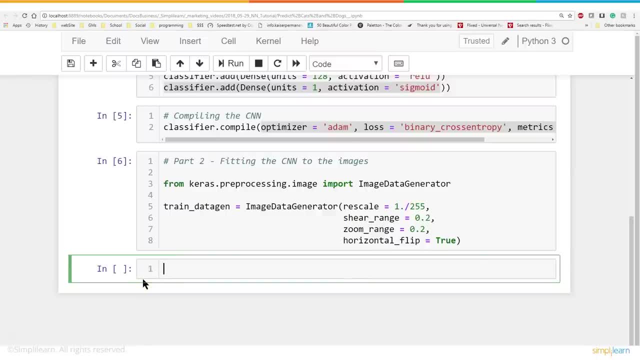 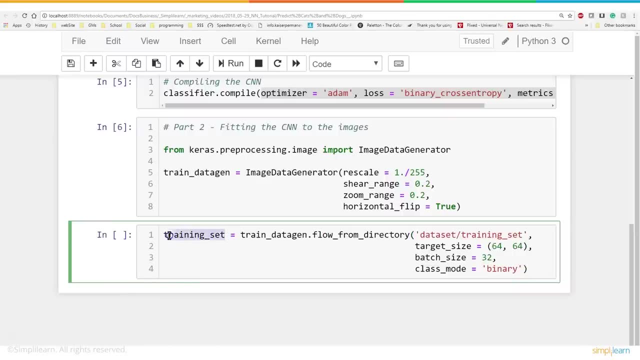 And again it doesn't really do anything Because we're still setting up the pre-processing. Let's take a look at this next set of code, And this one is just huge. We're creating the training set, So the training set Is going to go in here. 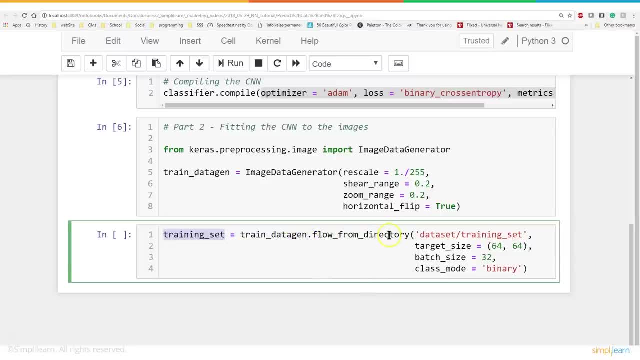 And it's going to use our train data gen. We just created Dot flow from directory. It's going to access, In this case, the path Data set, training set. That's a folder, So it's going to pull all the images. 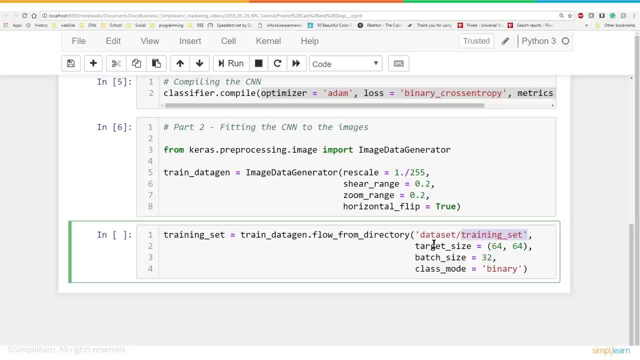 Out of that folder. Now I'm actually running this In the folder that the data set's in. So if you're doing the same setup And you load your data in there And you're doing this, Make sure wherever your Jupyter notebook is saving things to. 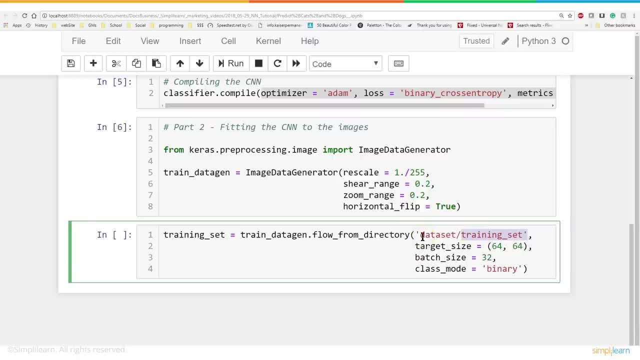 That you create this path Or you can do the complete path If you need to. You know C, colon slash, etc. And the target size, The batch size And class mode is binary. So the class is: We're switching everything to a binary value. 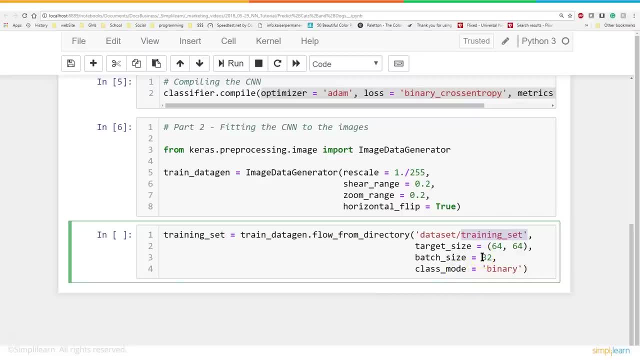 Batch size. What the heck is batch size? Well, that's how many pictures We're going to batch through the training each time And the target size: 64 by 64.. A little confusing, But you can see right here That this is just a general training. 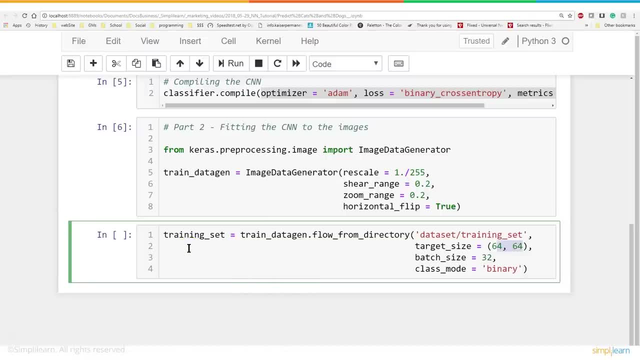 And you can go in there And look at all the different settings For your training set And, of course, with different data, We're doing pictures. There's all kinds of different settings Depending on what you're working with. Now let's go ahead and run that. 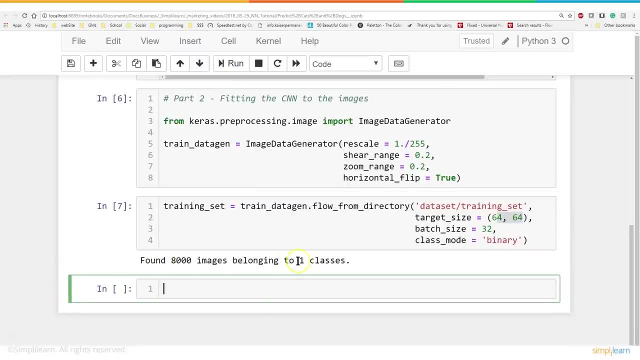 And see what happens, And you'll see that it found 800 images Belonging to one classes. So we have 800 images In the training set And if we're going to do this With the training set, We also have to format the pictures. 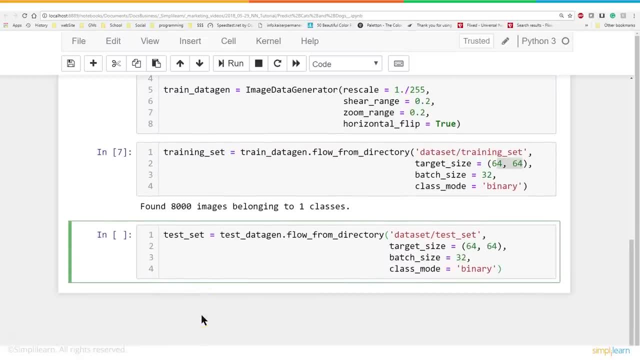 In the test set. So we're not actually doing any predictions. We're not actually programming the model yet. All we're doing is preparing the data. So we're going to prepare a training set And the test set. So any changes we make to the training set. 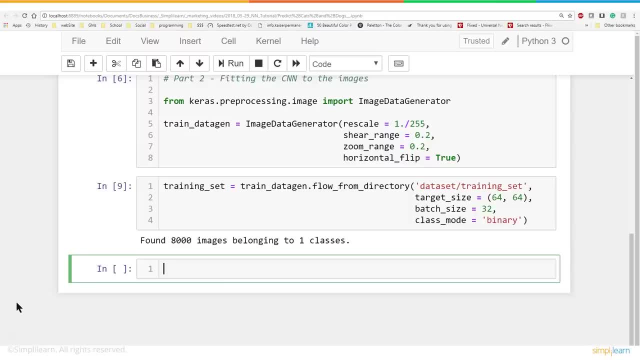 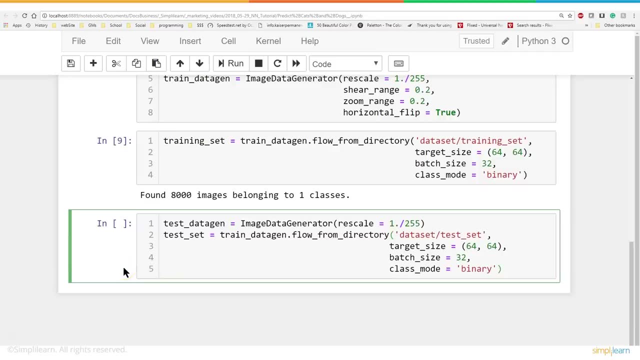 At this point Also have to be made to the test set. So we've done this thing, We've done a train data generator, We've done our training set, And then we also have- Remember- our test set of data. So I'm going to do the same thing with that. 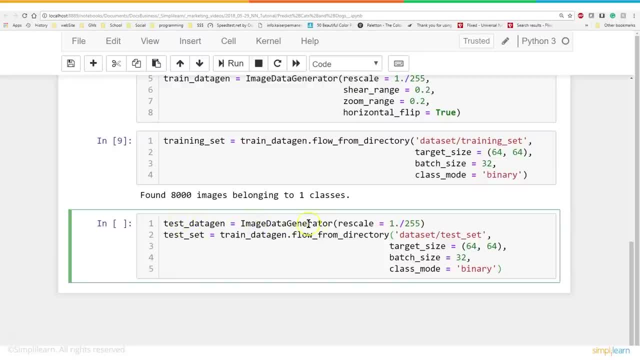 I'm going to create a test data gen And we're going to do this image data generator. We're going to rescale 1 over 255.. We don't need the other settings, Just the single setting for the test data gen. 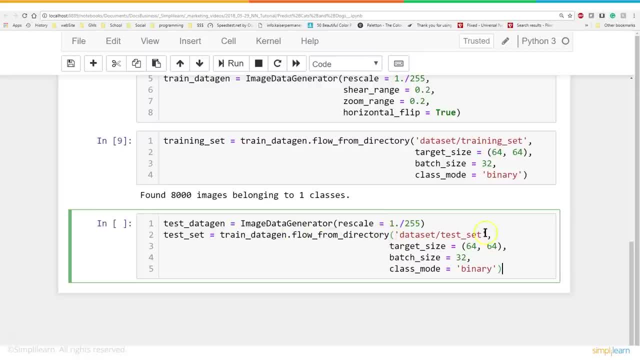 And we're going to create our test set. We're going to do the same thing we did with the test set, Except that we're pulling it from the test set folder And we'll run that And you'll see in our test set. 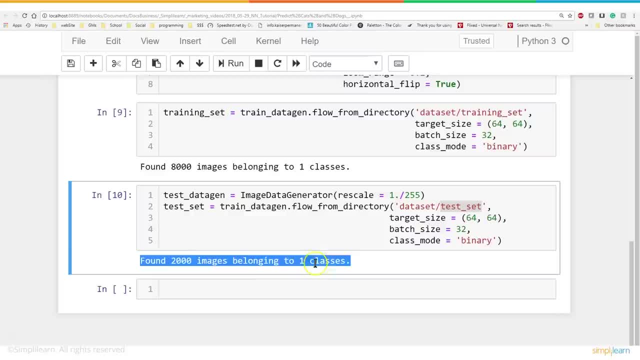 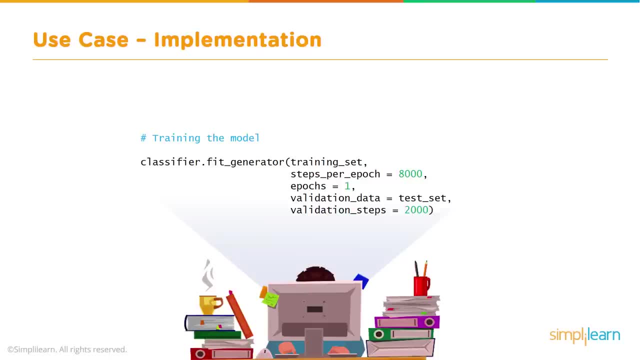 We found 2000 images. That's about right. We're using 20% of the images as test And 80% to train it. And then, finally, We've set up all our data, We've set up all our layers. 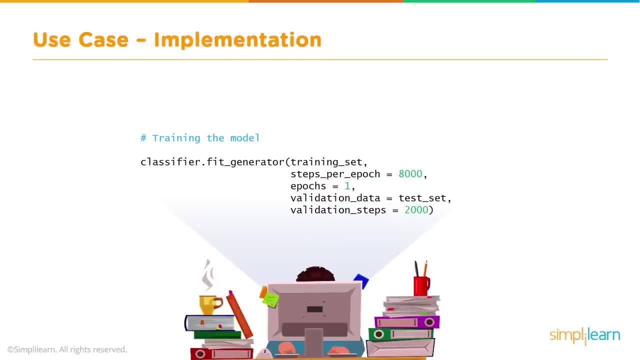 Which is where all the work is: Cleaning up that data, Making sure it's going in there correctly And we're actually going to fit it. We're going to train our data set And let's see what that looks like. And here we go. 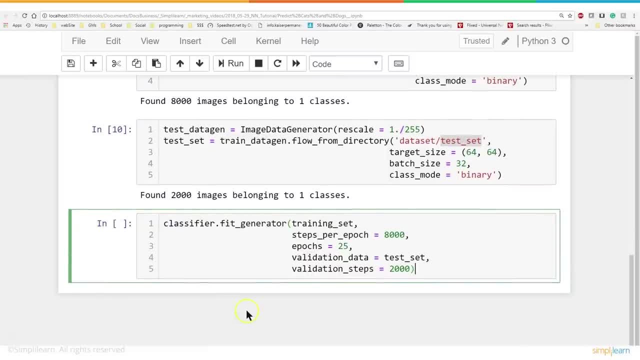 Let's put the information in here And let's just take a quick look At what we're looking at with our fit generator. We have our classifierfit generator, That's our back propagation, So the information goes through forward with the picture. 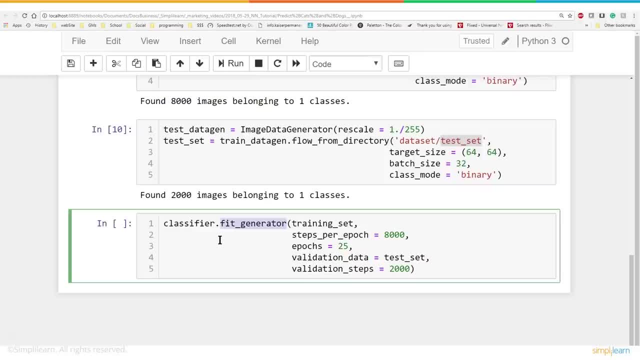 And it says: You're either right or you're wrong, And then the error goes backward And reprograms all those weights. So we're training our neural network And, of course, we're using the training set. Remember we created the training set up here. 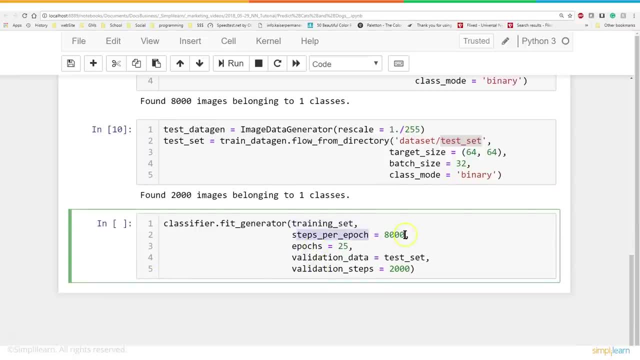 And then we're going steps per epic, So it's 8,000 steps. Epic means that That's how many times we go through all the pictures. So we're going to rerun each of the pictures And we're going to go through the whole data set 25 times. 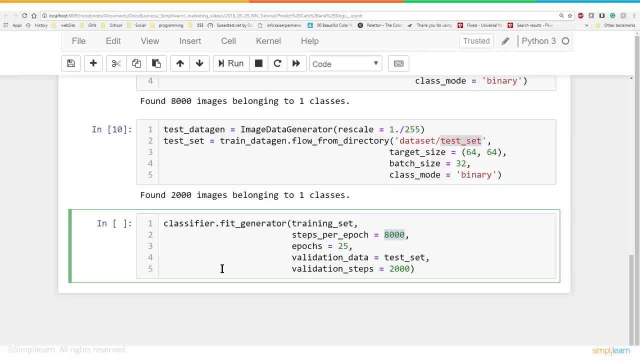 But we're going to look at each picture During each epic 8,000 times, So we're really programming the heck out of this And going back over it. And then they have validation data Equals test set. So we have our training set. 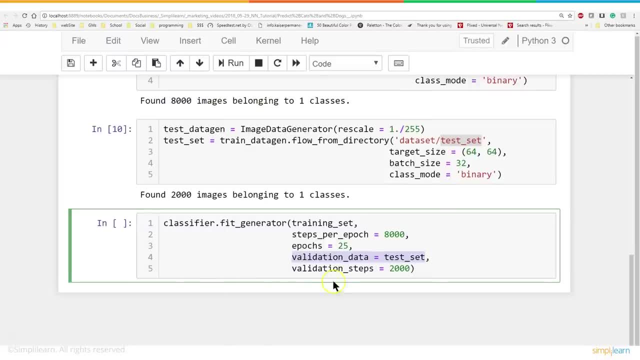 And then we're going to have our test set to validate it. So we're going to do this all in one shot And we're going to look at that, And they're going to do 200 steps for each validation And we'll see what that looks like in just a minute. 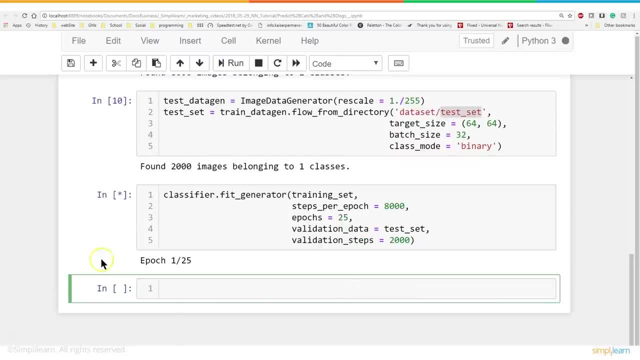 Let's go ahead and run our training here And we're going to fit our data And, as it goes, It says epic 1 of 25.. You start realizing that this is going to take a while. On my older computer It takes about 45 minutes. 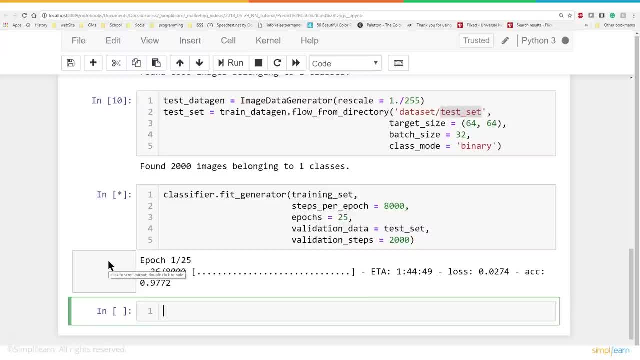 I have a dual processor And we're processing 10,000 photos. That's not a small amount of photographs to process. So if you're on your laptop- Which I am- It's going to take a while, So let's go ahead. 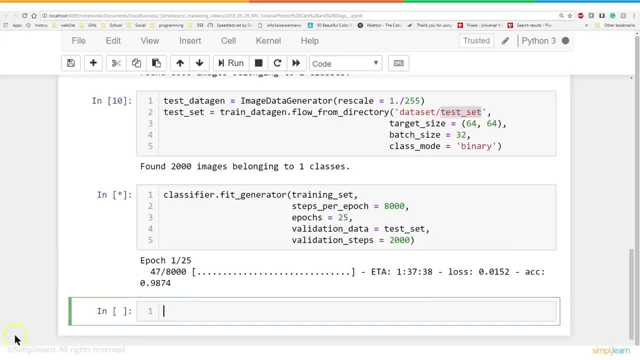 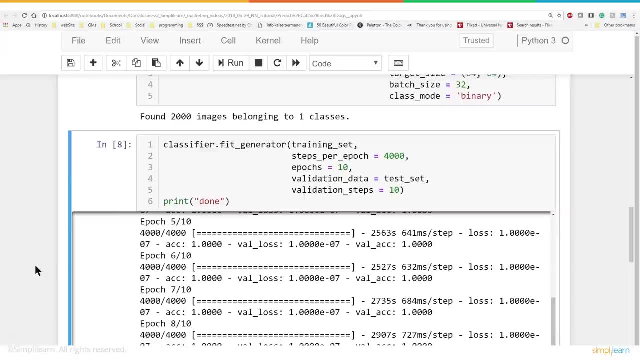 And go get our cup of coffee And a sip And come back and see what this looks like. So I'm back. You didn't know I was gone. I was actually a lengthy pause there. I made a couple changes And let's discuss those changes real quick. 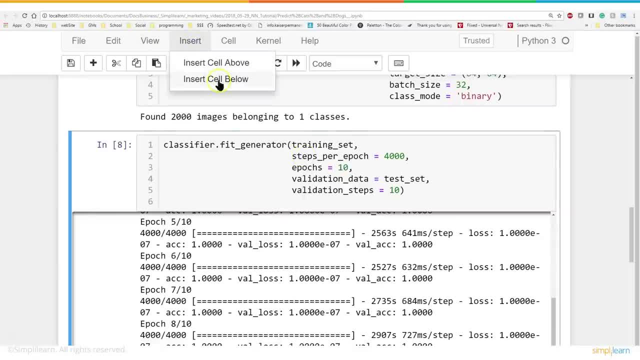 And why I made them. So the first thing I'm going to do Is I'm going to go up here And insert a cell above And let's paste the original code back in there And you'll see that the original code. 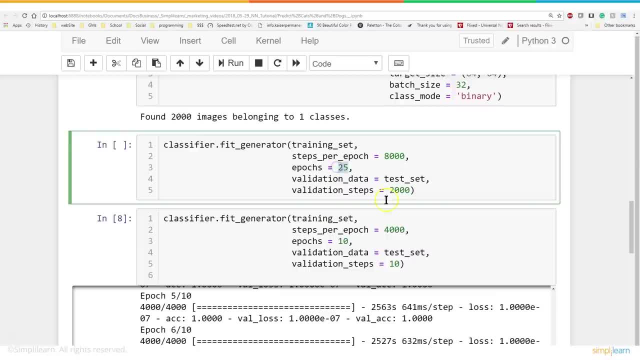 Was steps per epic: 8,000.. 25 epics And validation steps: 2,000.. And I changed these to 4,000 epics, Or 4,000 steps per epic. 10 epics. 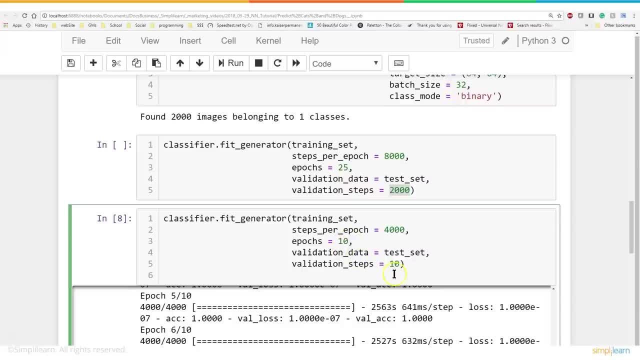 And just 10 validation steps, And this will cause problems. If you're doing this As a commercial release, But for demo purposes, This should work. And if you remember Our steps per epic, That's how many photos We're going to process. 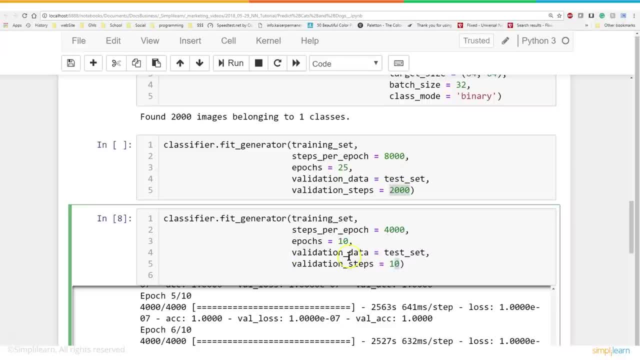 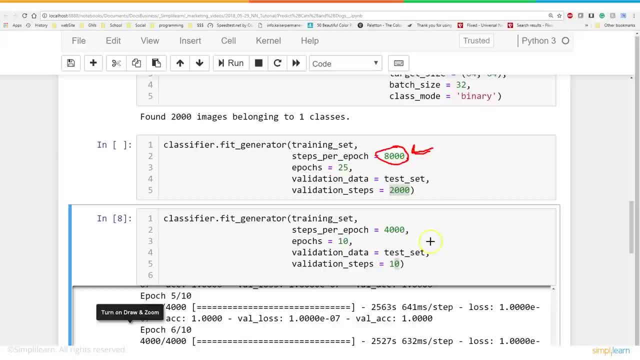 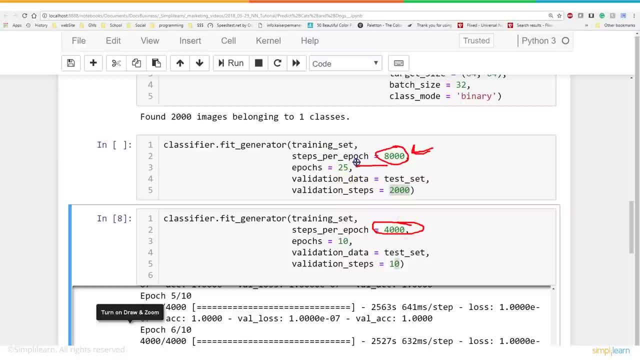 20 EPIC PICTURES HAVE THREE E depictors 20 E harvest Absolutely 100.. 200 each. 28,000.. 8,000.. 500.. cuatro pesos: 800.. 100 percent: 4,000.. 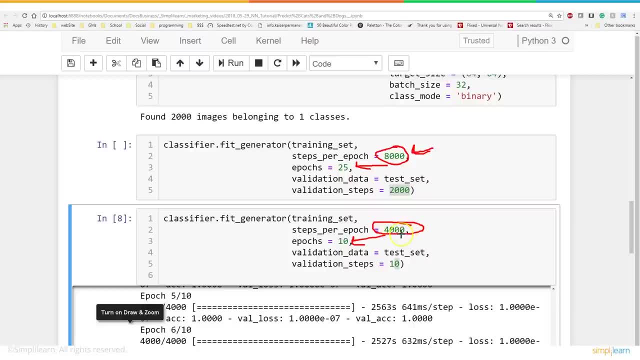 6,000. 8,000. 8,000 Trails each Explore. these Can manage these photos. The results of eachEpic Can do the math, Don't talk me About this. Causes change the validation step And this would cause some major problems in releasing, because I dropped. 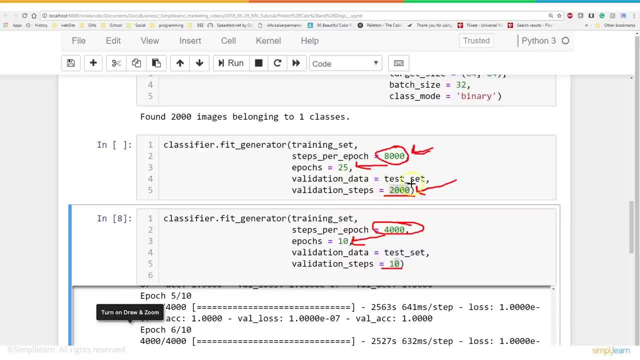 it all the way down to 10.. What the validation step does is it says we have 2,000 photos in our trainings or in our testing set And we're going to use that for validation. Well, I'm only going to use a random 10 of those to validate, So not really the best settings, but let me show you why. 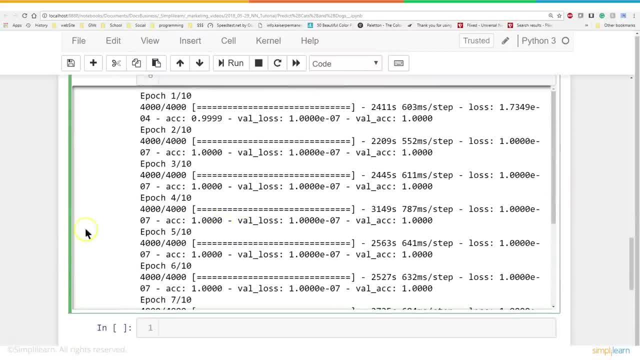 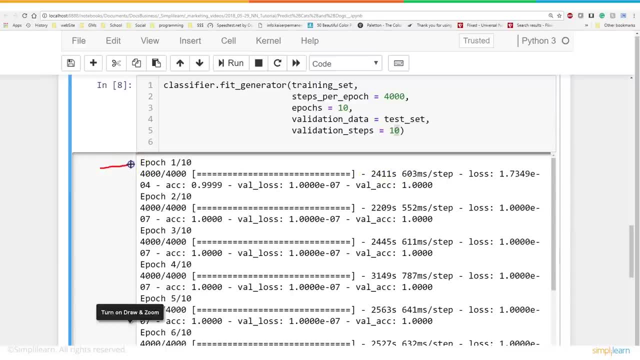 we did that. Let's scroll down here just a little bit And let's look at the output here and see what's going on there. So I've got my drawing tool back on And you'll see here it lists a run. So each time it goes through an epic it's going to do 4,000 steps, And this is where the 4,000 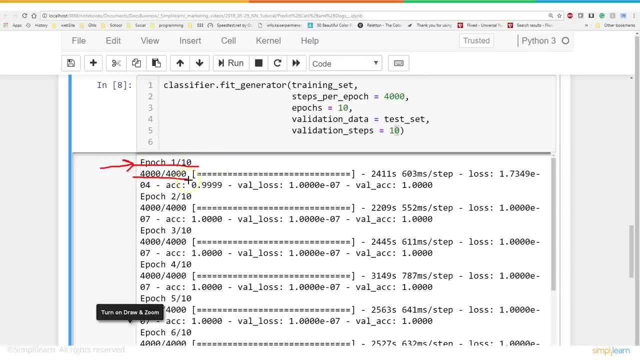 comes in. So that's where we have. We have epic 1 of 10, 4,000 steps. It's randomly picking half the pictures in the file and going through them And then we're going to look at this number right. 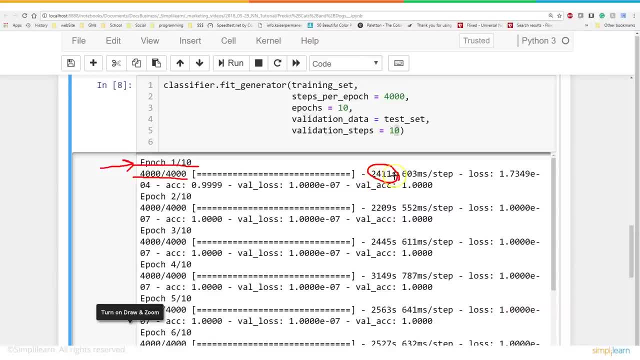 here. That is for the whole epic And that's 2,411 seconds. And, if you remember correctly, you divide that by 60, you get minutes. If you divide that by 60,, you get hours, Or you can just divide the whole thing by 60 times 60,, which is 3,600. 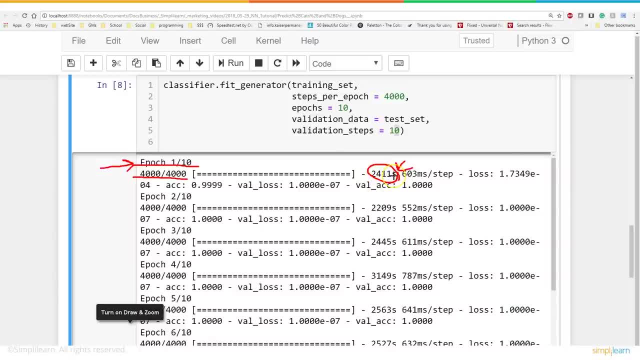 If 3,600 is an hour, this is roughly 45 minutes right here And that's 45 minutes to process half the pictures. So if I was doing all the pictures, we're talking an hour and a half per epic times 36. Or no 25. They had 25 up above 25.. So that's roughly a couple days. 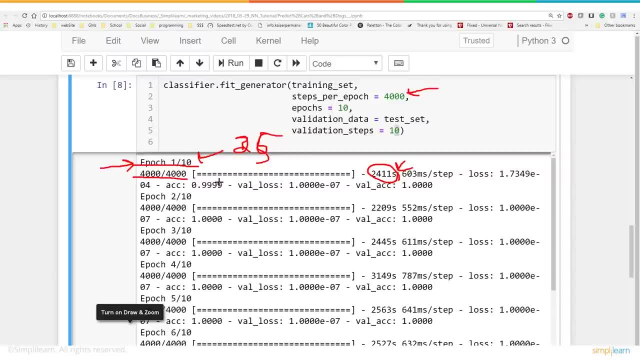 A couple days of processing Well, for this demo. we don't want to do that. I don't want to come back the next day. Plus, my computer Did a reboot in the middle of the night. So we look at this and we say, OK, we're just testing. 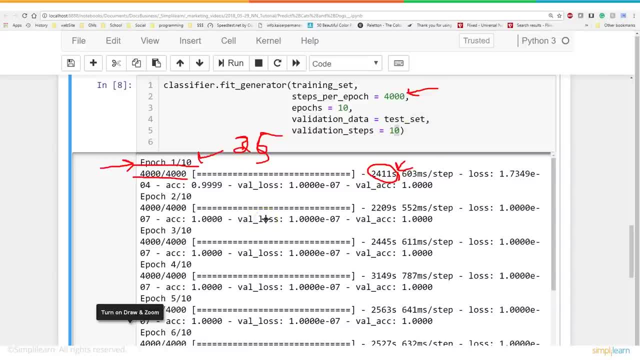 this out: My computer that I'm running this on is a dual core processor, Runs 0.9 gigahertz per second. For a laptop it was good about four years ago, But for running something like this it's probably a little slow. So we cut the times down, And the last one was validation. We're only 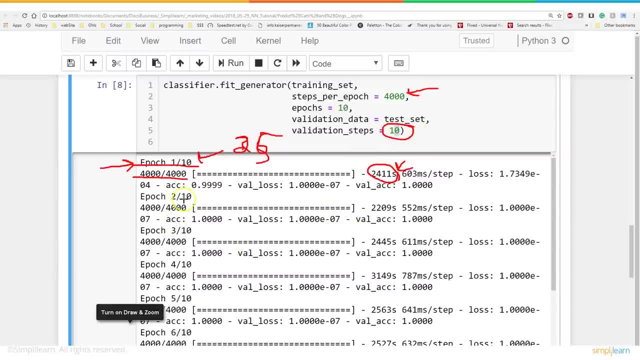 validating it on a random 10 photos. And this comes into effect Because you're going to see down here where we have accuracy, value, loss, value, accuracy And loss. Those are very important numbers to look at. So the 10 means I'm only validating. 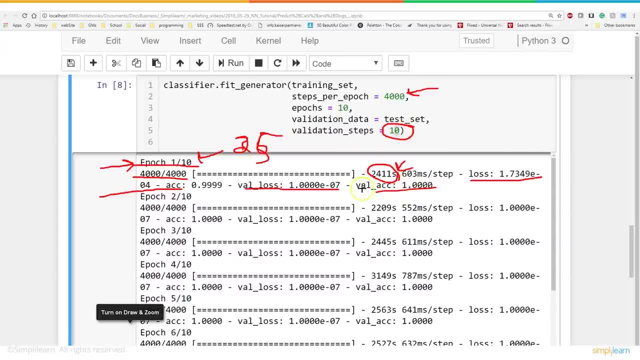 across 10 pictures. That is where, here, we have value. This is ACC is for accuracy, Value loss- we're not going to worry about that too much. And accuracy Now, accuracy is while it's running. it's putting these two numbers together. That's what accuracy is And value accuracy is at the 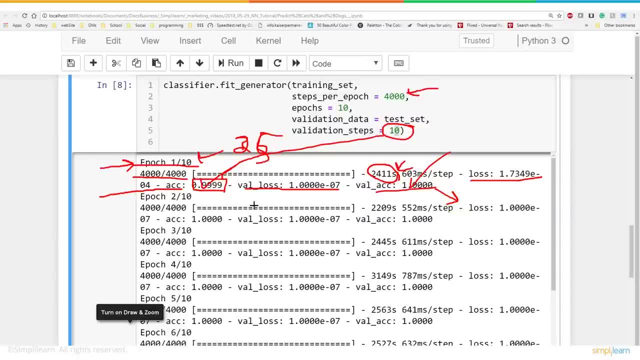 end of the epic. What's our accuracy? end of the epic. What is it looking at? In this tutorial we're not going to go so deep, But these numbers are really important. when you start talking about these, two numbers reflect bias. That is really important. Let me just put: 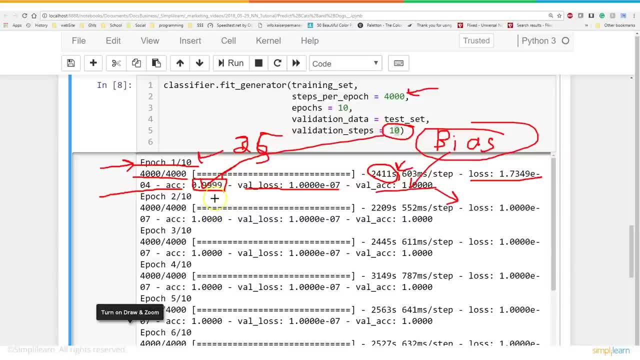 that up there And bias is a little bit beyond this tutorial, But the short of it is is if this accuracy, which is being our validation per step, is going down and the value accuracy continues to go up, that means there's a bias. That means I'm memorizing the photos I'm looking at. I'm not. 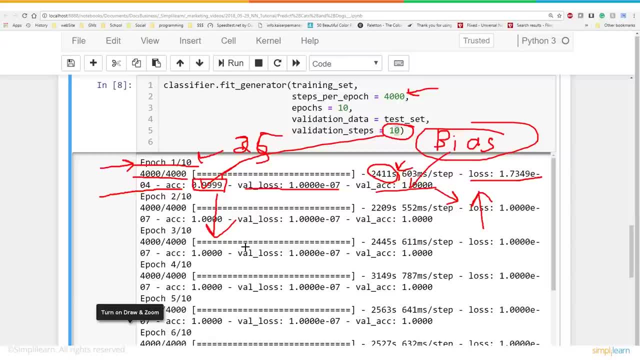 actually looking for. what makes a dog a dog? what makes a cat a cat? I'm just memorizing, And so the more this discrepancy grows, the bigger the bias is. And that is really the beauty of the cross neural network is a lot of built in features like this that make that really easy to 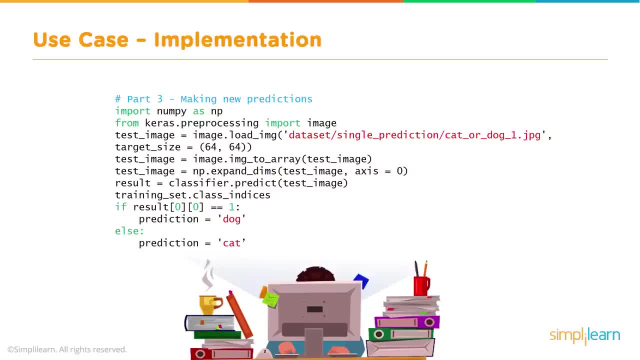 track. So let's go ahead and take a look at the next set of code. So here we are into part three. we're going to make a new prediction, And so we're going to bring in a couple tools for that, And then we have to process the image coming in and find out whether it's an actual dog or cat. 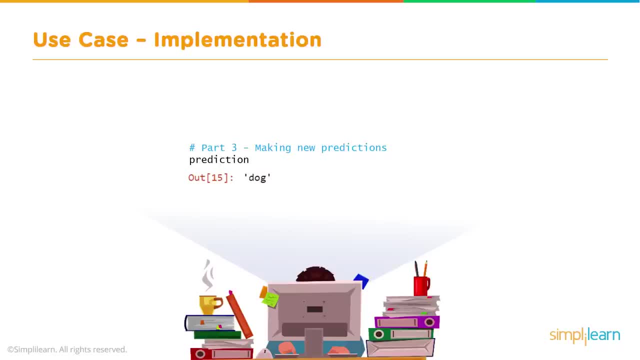 we can actually use this to identify it. And of course, the final step, part three, is to print prediction. we'll go and combine these And of course you can see me there adding more sticky notes to my computer screen, hidden behind the screen. And last one, 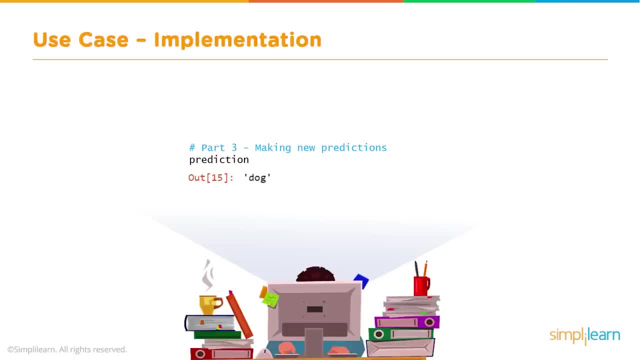 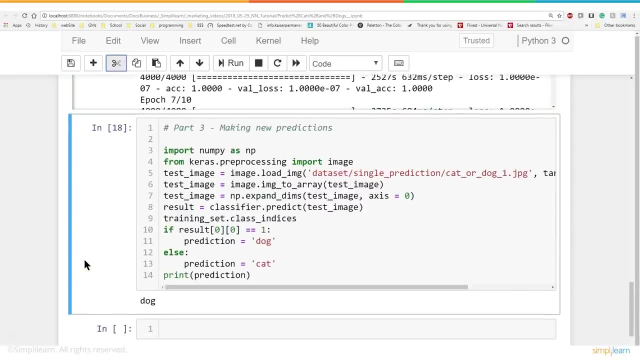 was: don't forget to feed the cat and the dog. So let's go and take a look at that and see what that looks like in code and put that in our Jupyter notebook, All right, and let's paste that in here, And we'll start by importing numpy as np. numpy is a very common package. 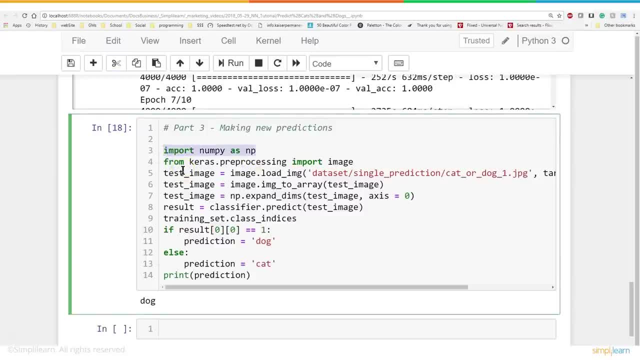 I pretty much imported on any Python project I'm working on. Another one I use regularly is pandas. they're just ways of organizing the data. And then np is usually the standard in most machine learning tools as a return for the data array, Although you can use a standard data array. 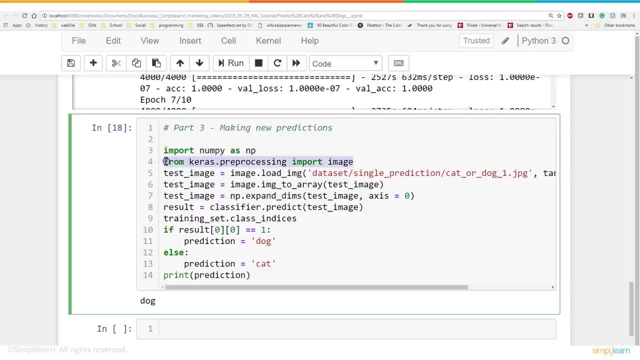 from Python And we have cross pre processing import image. this at all look familiar because we're going to take a test image And we're going to set that equal to, in this case, cat or dog one, as you can see over here. And you know, let me get my drawing tool back on. 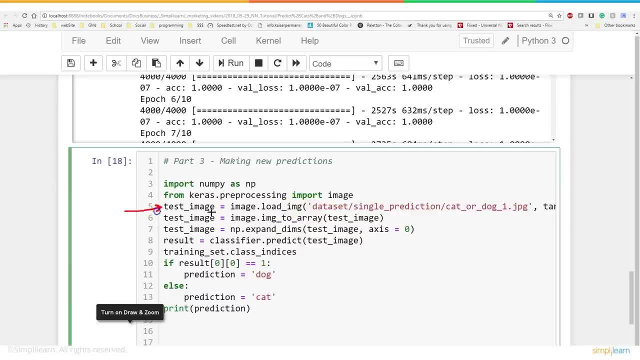 So let's take a look at this. we have our test image we're loading and in here we have test image one And this one hasn't. data hasn't seen this one at all, So this is all new. Oh, let me shrink the screen down, Let me start that over. So here we have my test. 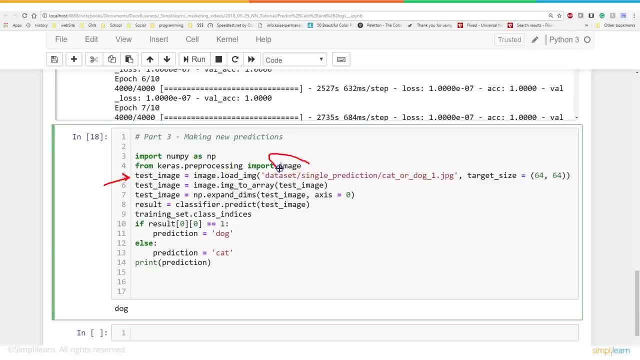 image And we went ahead and the cross processing has this nice image setup. So we're going to load the image and we're going to alter it to 64 by 64 print. So right off the bat we're going to cross this nice. that way it automatically sets it up for us, So we don't have to redo all our images. 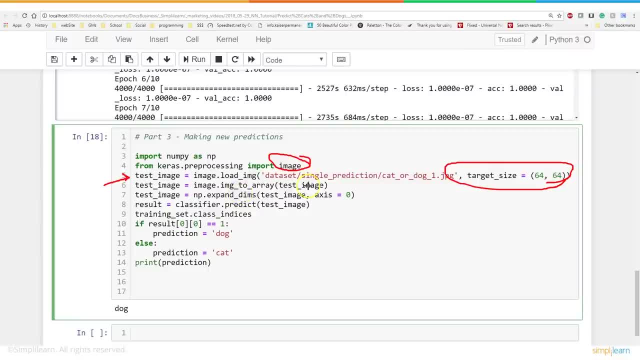 and find a way to reset those, And then we use also to set the image to an array. So again, we're all in pre processing the data, just like we pre process before with our test information and our training data, And then we use the numpy. Here's our numpy, That's from our right up here. 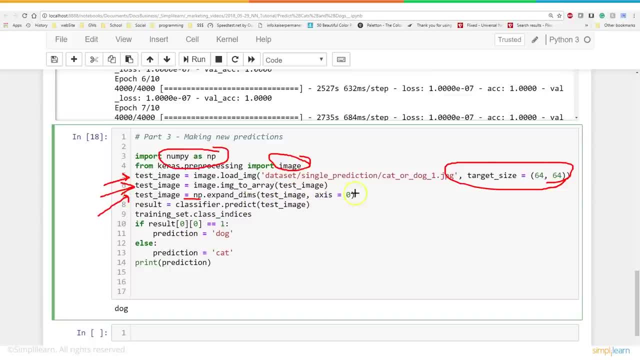 important numpy, as in P, expand the dimensions. test image axes equals zero, So puts it into a single array. And then finally, all that work, all that pre processing, And all we do is we run the result, we click on here, we go: result equals classifier, predict test image. And then we find: 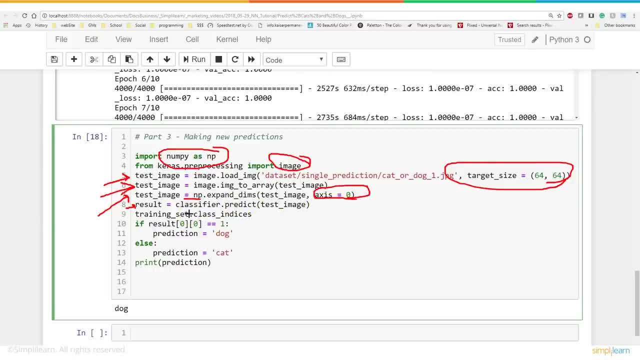 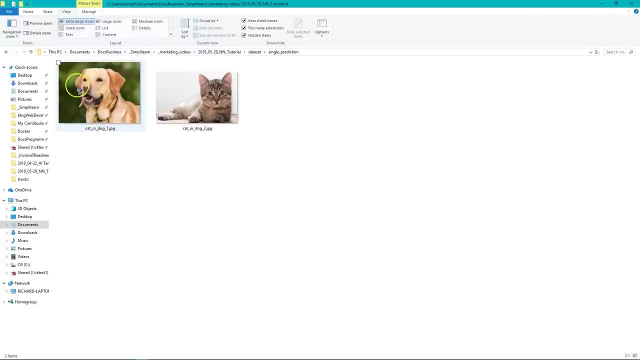 out. Well, what is the test image? And let's just take a quick look and just see what that is, And you can see when I ran it. it comes up dog, And if we look at those images there, it is cat or dog. image number one that 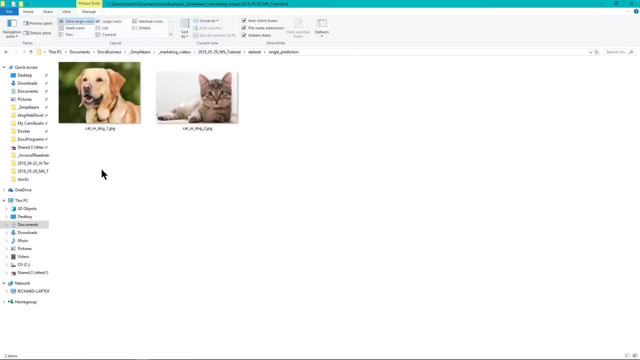 looks like a nice floppy eared lab, friendly, with his tongue hanging out. It's either that or a very floppy eared cat, I'm not sure which, but according to our software says it's a dog And we have a second picture over here. Let's just see what happens when we run the second picture. We can go. 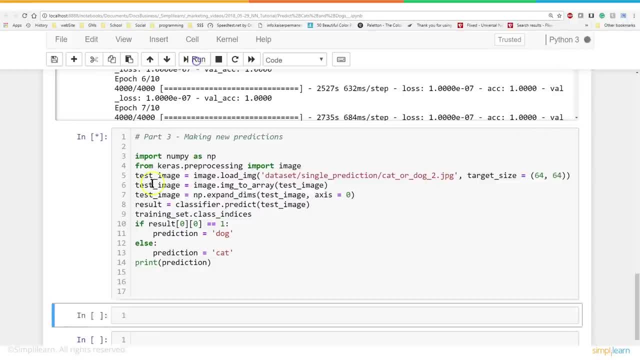 up here and change this from dog image one to two. we'll run that and it comes down here and says cat and we're going to see me highlighting it down there as cat. So our process works. you're able to label a dog a dog and a cat a cat just from the pictures. There we go, cleared my drawing tool And 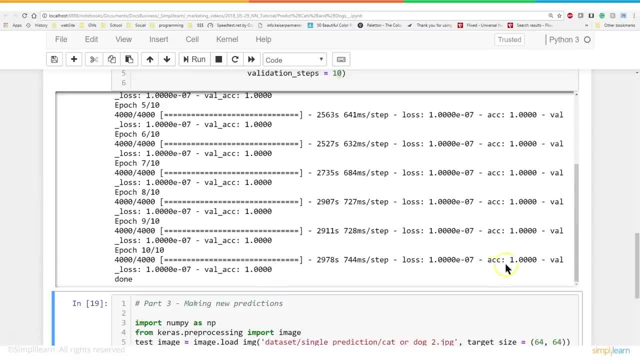 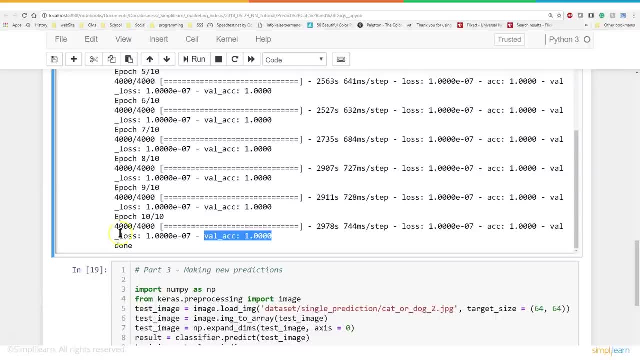 the last thing I want you to notice: when we come back up here to when I ran it, you'll see that has an accuracy of one and the value accuracy of one. Well, the value accuracy is the important one, because the value accuracy is what it actually runs on the test data. Remember, I'm only testing. 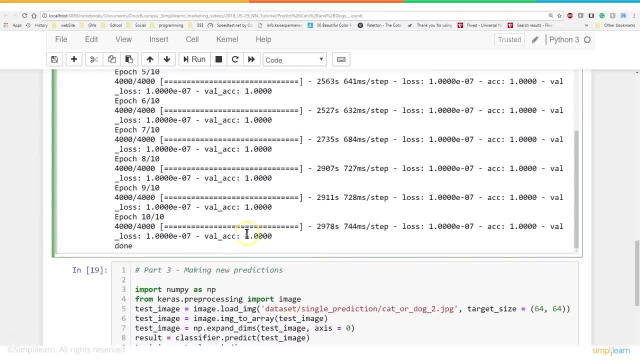 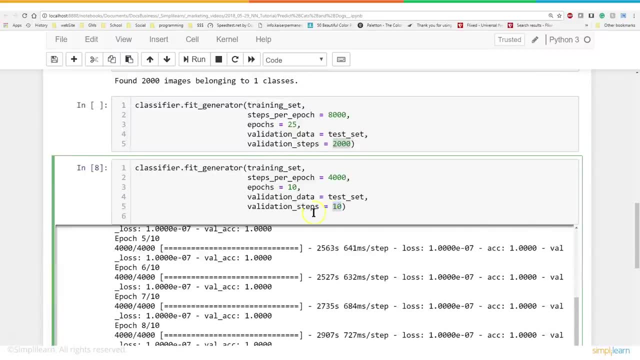 it on. I'm only validating it. on a random 10 photos Just happened to come up one. Now, when they ran this on the server, it actually came up about 86%. This is why cutting these numbers down so far for a commercial release is bad. So you want to? 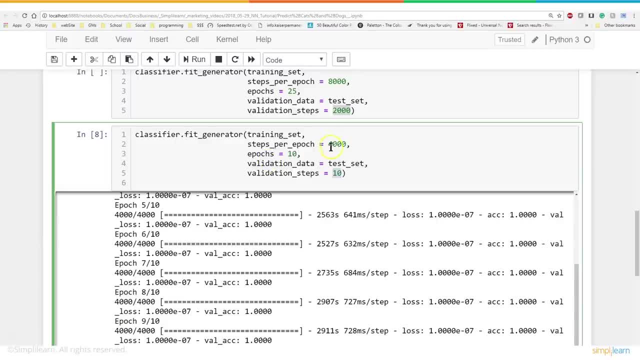 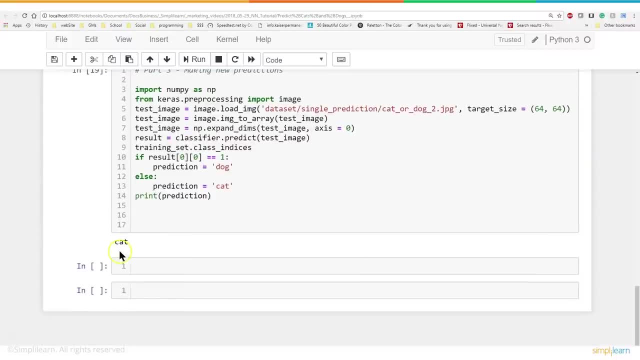 make sure you're a little careful of that when you're testing your stuff, that you change these numbers back when you run it on a more enterprise computer other than your old laptop that you're just practicing on or messing with, And we come down here and again you know we had the validation. 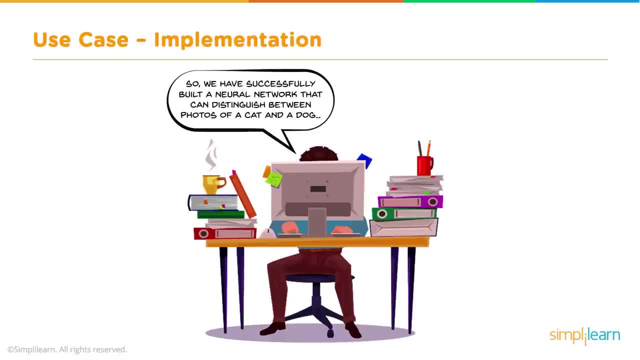 of cat, And so we have successfully built a neural network that could distinguish between photos of a dog. Imagine all the other things you could distinguish. Imagine all the different industries you could dive into with that. Just being able to understand those two difference of pictures. What 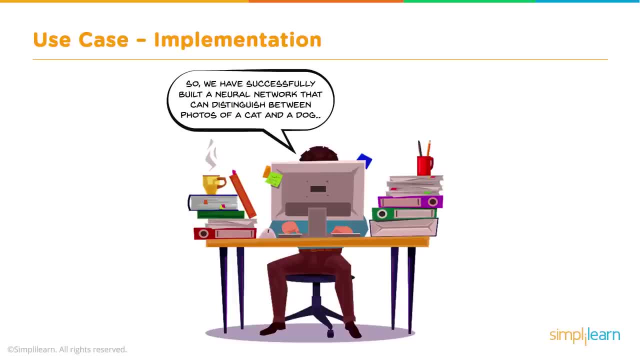 about mosquitoes. Could you find the mosquitoes that bite versus mosquitoes that are friendly? It turns out the mosquitoes that bite us are only 4% of the mosquito population. If even that, maybe 2%. There's all kinds of industries that use this And there's so many industries that 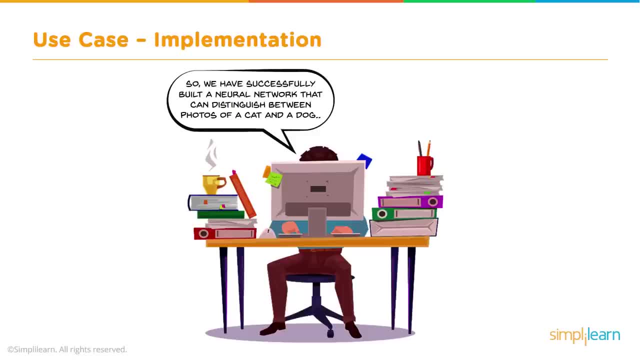 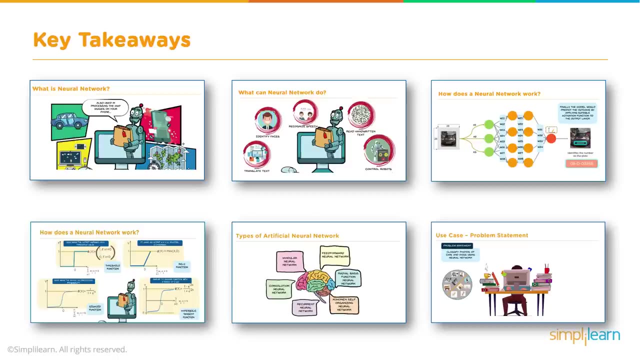 are just now realizing how powerful these tools are. Just in the photos alone, there is a myriad of industry sprouting. And I said it before, I'll say it again: What an exciting time to live in with these tools and that we get to play with So key takeaways. Well, we covered. what is a neural network? We? 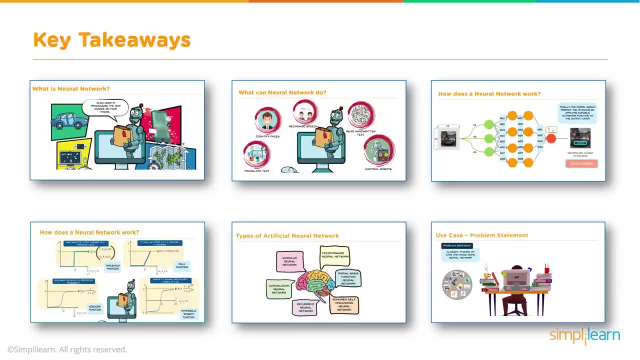 use all kinds of processing the map images on your phone. We talked about things that a neural network can do: Translate text, identify faces, all the way to control robots. You know lots of exciting things. How does a neural network work? So we discussed that with the different layers. 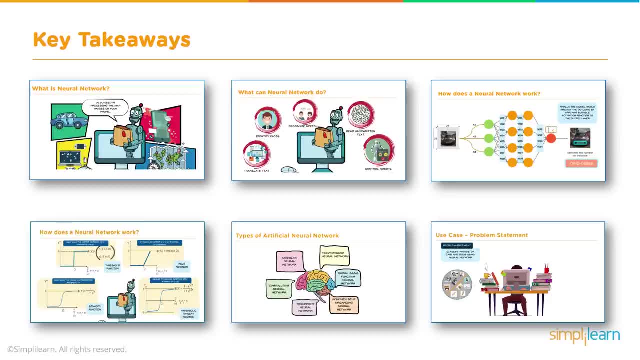 going from the picture to the input layer, to the hidden layers and their weights, to the final output layer. We also talked about how it does the math and computing the output as a yes or no, categorically true, false. We discussed types of artificial neural networks- A lot of vocabulary there from the feed forward neural. 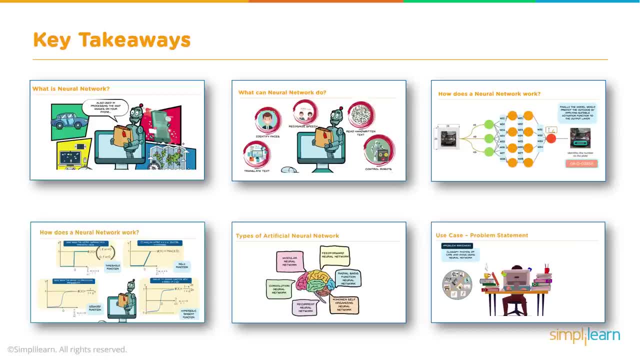 network which is the most commonly used. That's the one. the neural network we used is a feed forward neural network that does backward propagation to train. And there's a lot of other ones out there. There's the radial biases, the cohenin, self-organizing recurrent neural network. 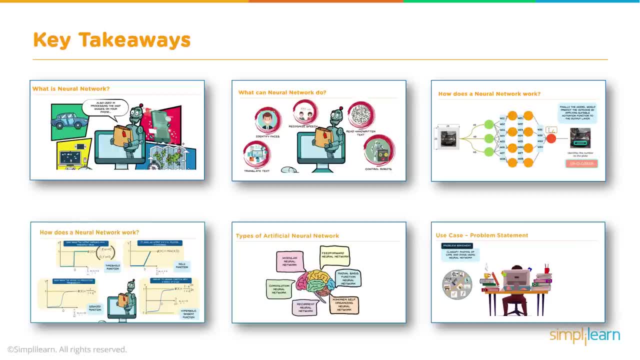 evolution. neural network- modular neural network- The big one was modular because it incorporates pieces of all the other ones, so that whatever you're working on now is a huge conglomerate of multiple networks, Just all cutting edge. All of it's new People even working on it don't even 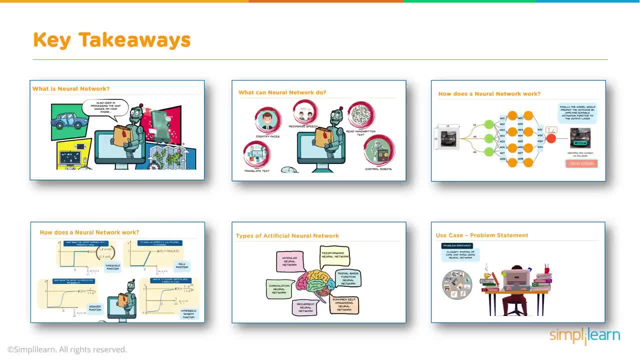 know where it's going. Again, very exciting times. And finally we dug through my favorite part. You can see, with my latte on one side, my old school pens and pencil and all my sticky notes working away. That's not actually me, by the way.